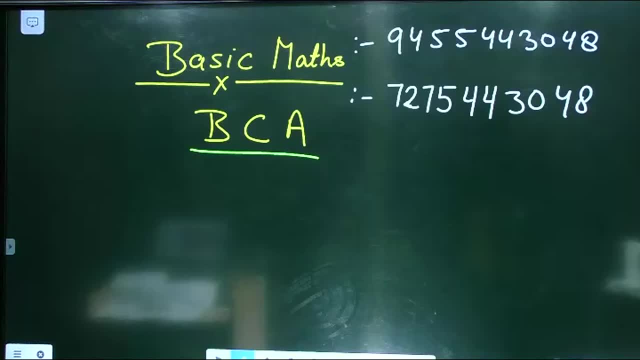 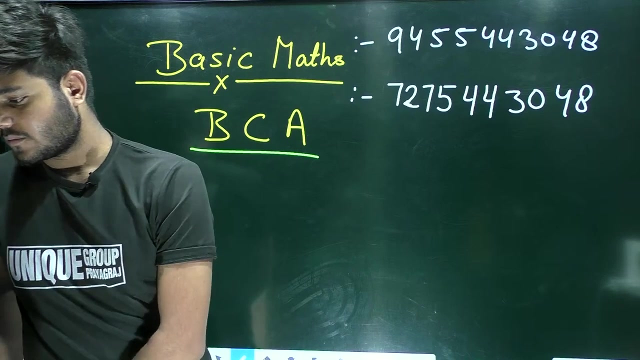 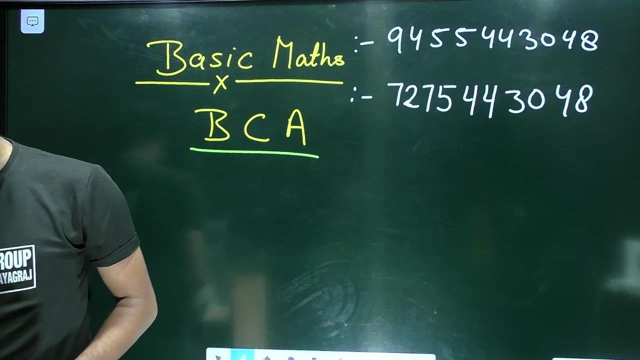 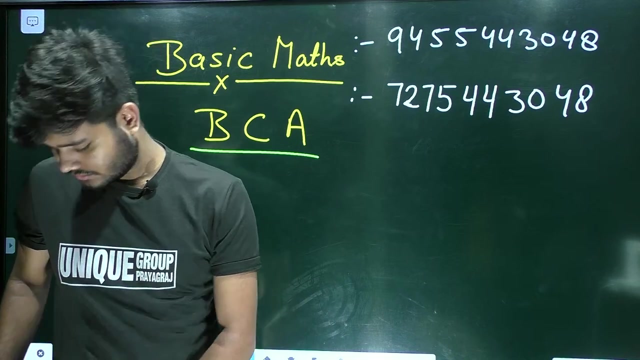 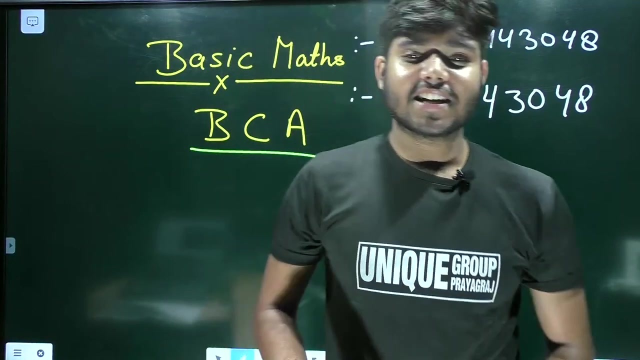 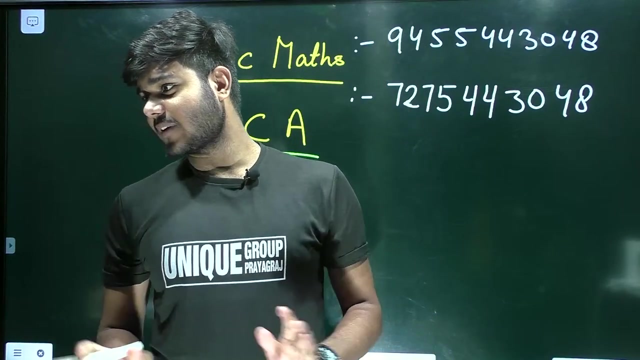 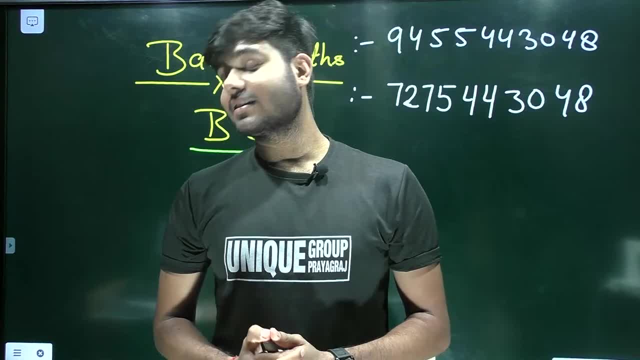 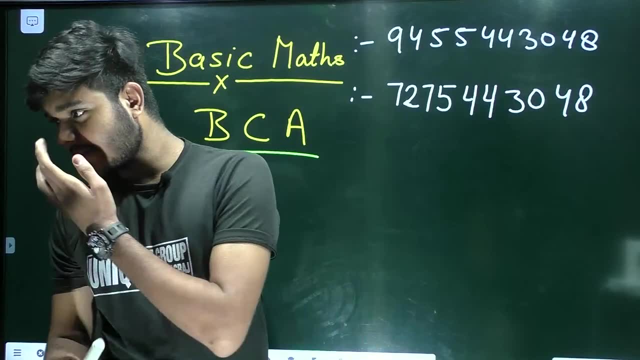 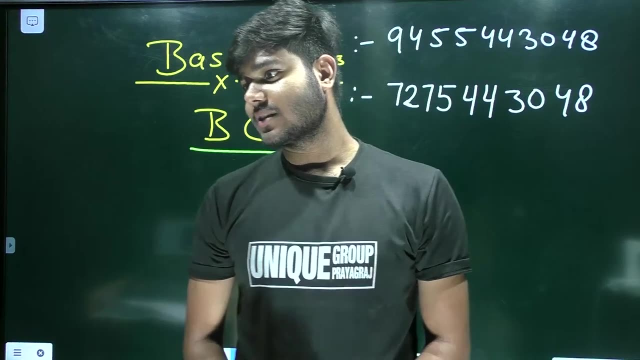 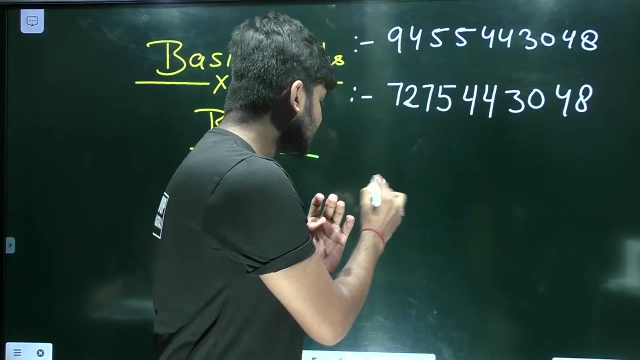 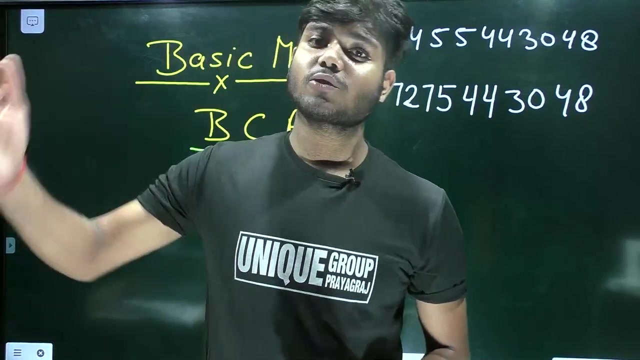 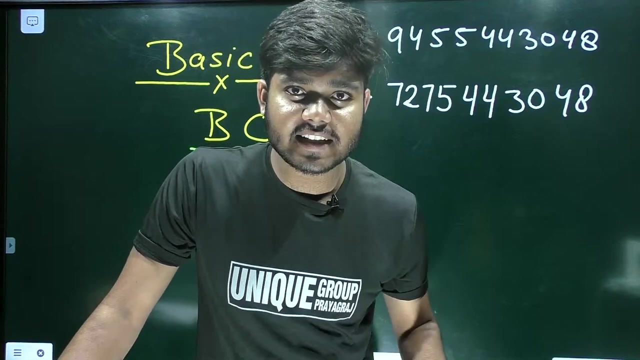 Hello, Hello, Hello, Hello, Hello, Hello. Like the session and share it with your friends. This session will be of basic mathematics, BCA, first semester, Any university Entrance exam. It will help you in everything If you are a 12th grader. 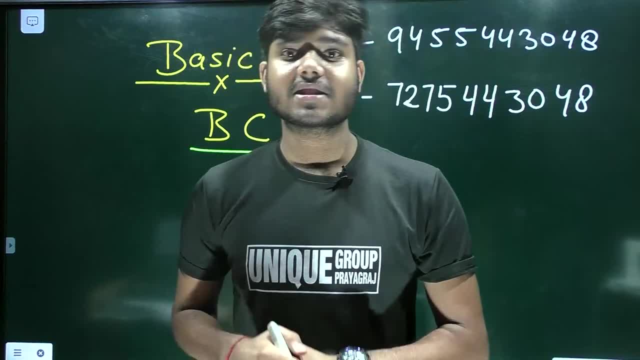 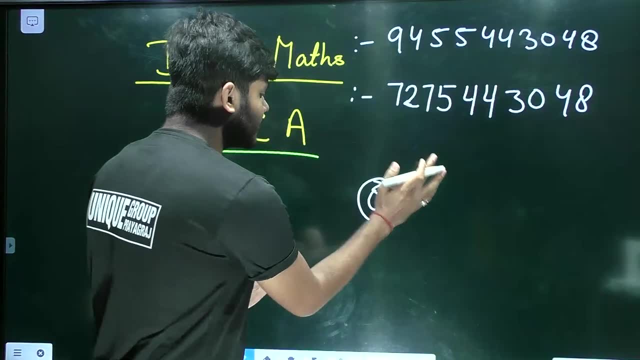 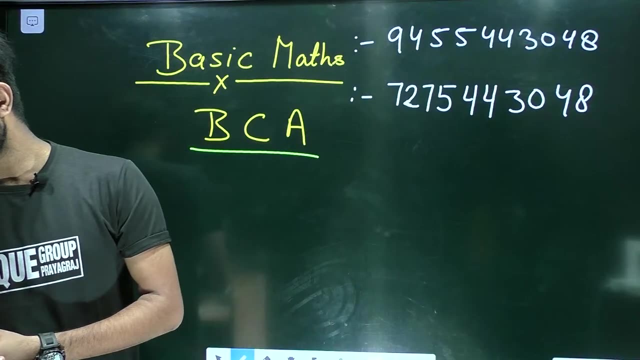 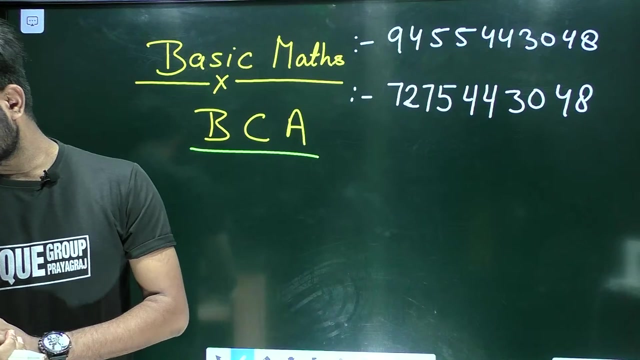 Then the chapters of determinant and matrix. That chapter is also in 12th class of 12th class of your class, So you just have to be carefree and support. You have to study hard And you can ask directly. Okay, Okay, Good morning everyone. Let's join quickly. 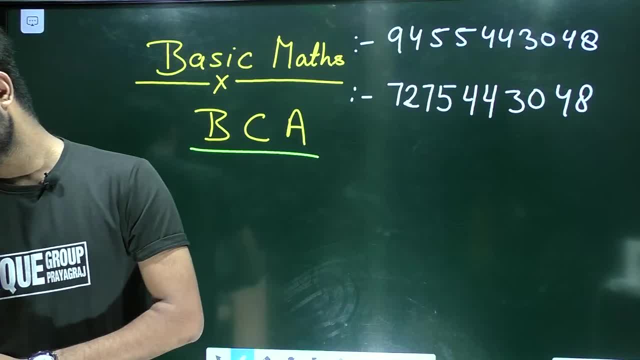 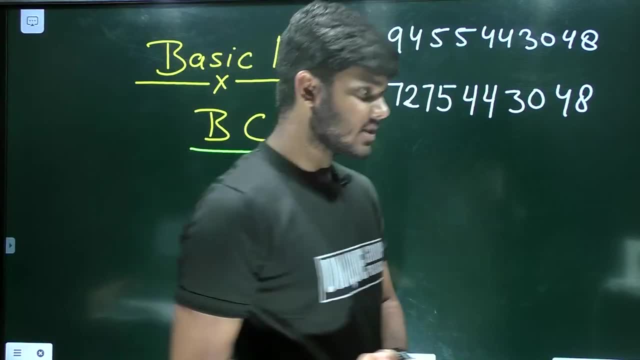 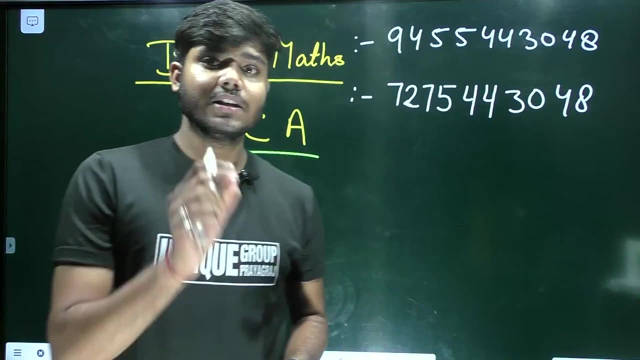 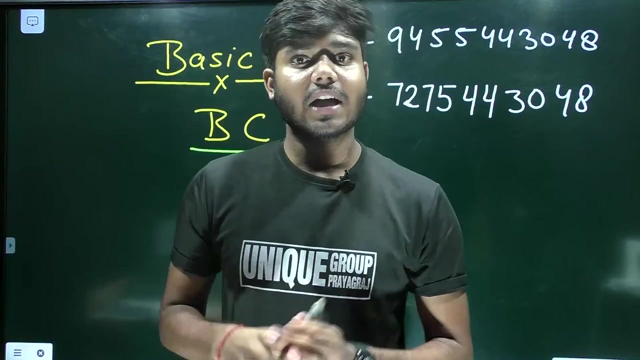 Arjun Kumar. Good morning, Let's go. Megha Kumari Abdul. Welcome everyone. From today, we will start basic mathematics- BCA. We will start Basic mathematics BCA. Notes will be provided daily. You can join telegram link. Whatever you will be taught daily, Notes will be given to you on telegram. 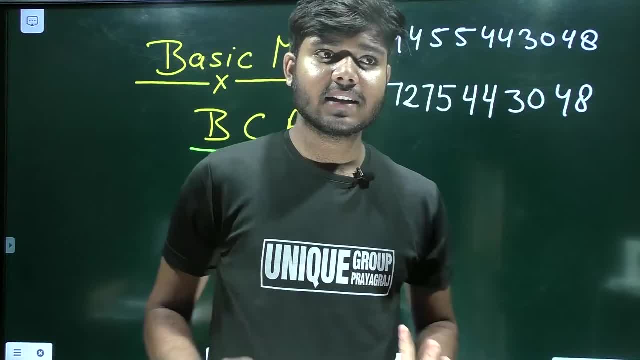 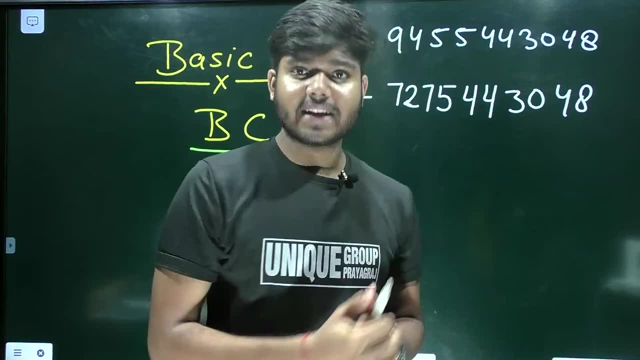 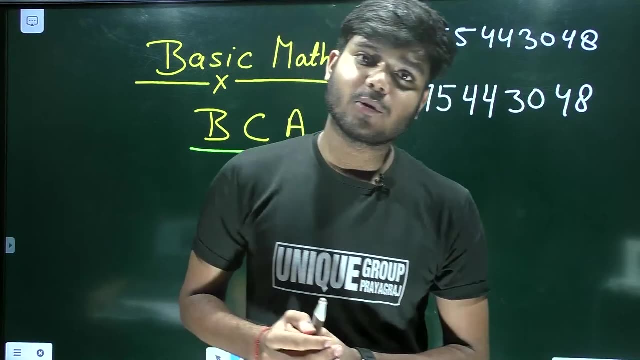 Okay, No need to worry about notes. No need to worry about class. Class will be provided. Take notes. Questions will also be provided. Suppose we finished one chapter, We will provide you questions On the basis of the same chapter. So what you have to do And whoever will solve. 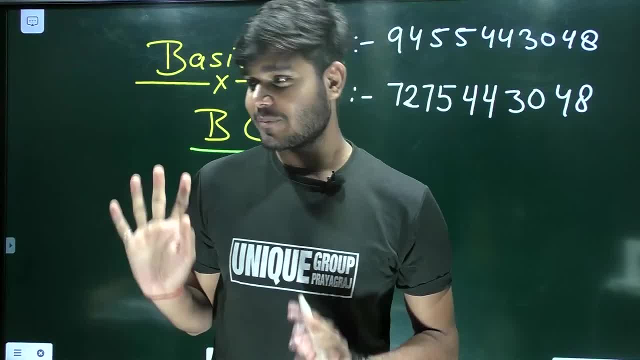 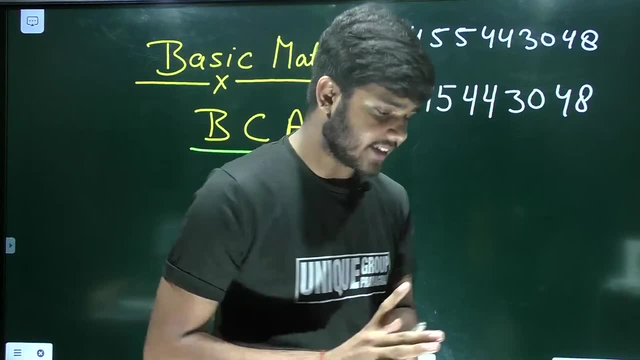 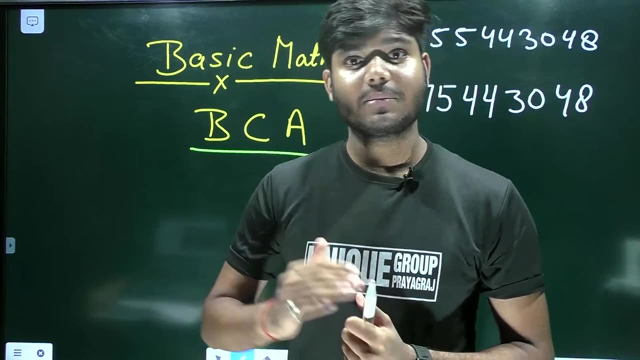 Who will get the correct answer Will get the correct answer. Okay, See, this is our rule. No, no, no, Megha kumari, Maths of 11th and 12th will not be taught. In basic mathematics There are some parts of matrix and determinant. Okay, So we will start it from zero level. 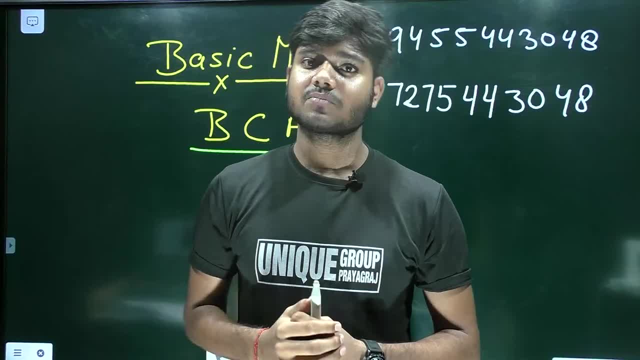 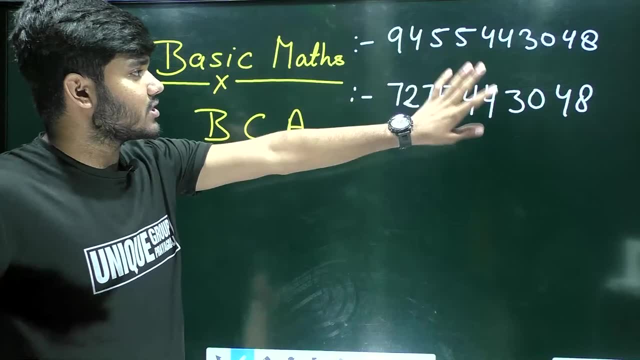 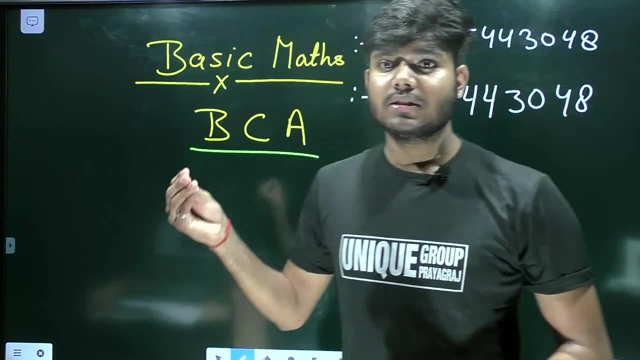 We will start from zero level. Means 11th and 12th will also come. See, we don't want to jump directly. You can do the class, without any doubt. Okay, And whatever problems you will face, This is your whatsapp number. You can do whatsapp here. Whatever you want to say. 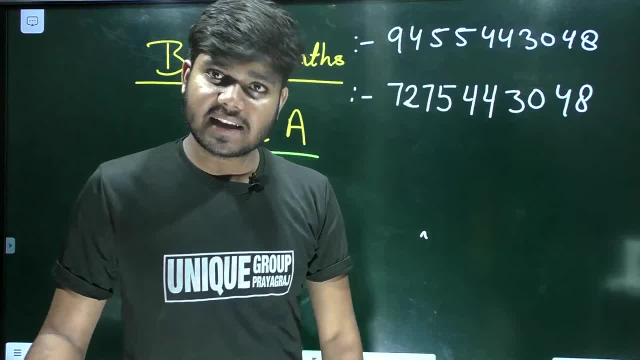 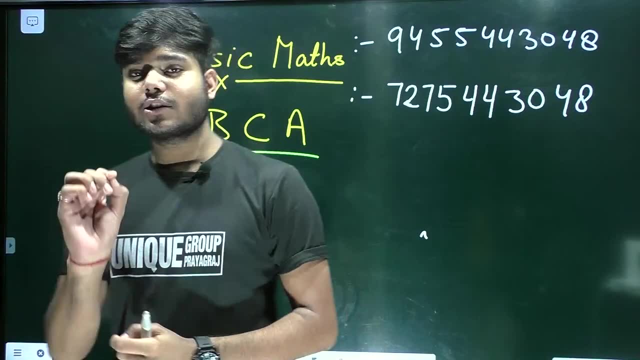 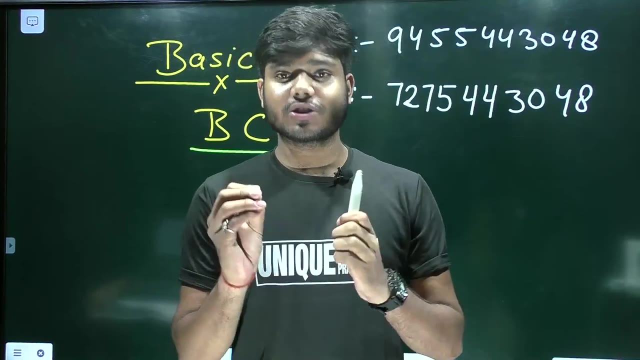 Ask or tell, Or if you want to say something related to class, What you have to do. You can message on whatsapp. You can join telegram link. You can take notes from there. Okay, See ignu or any university. All are available for university. All students are satisfied, Okay. 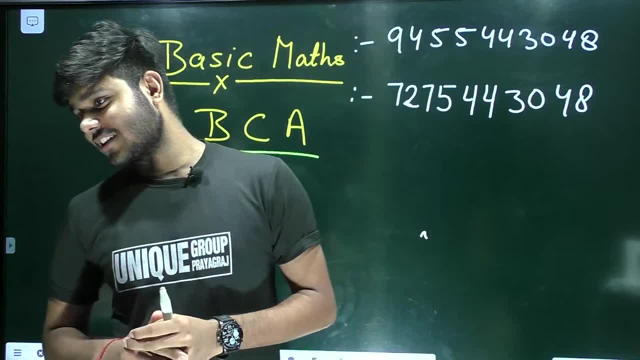 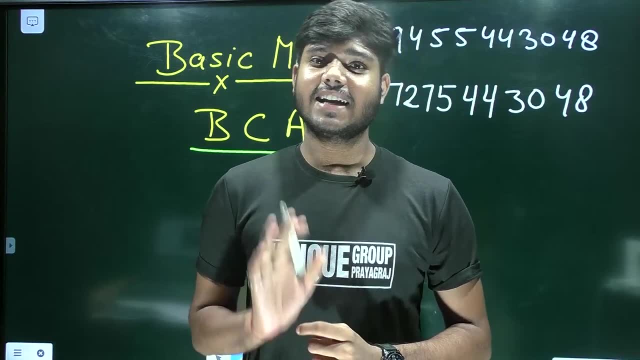 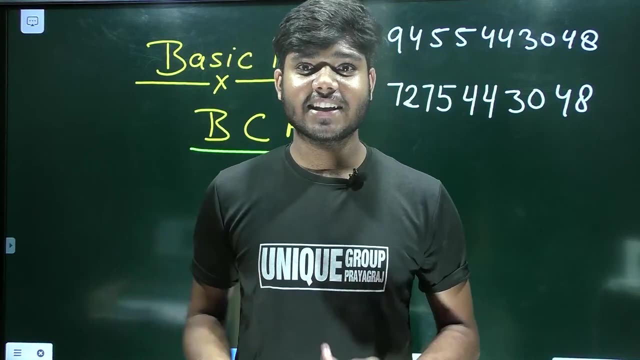 So what you have to do- See how many of you have come Like. just come See attendance. It is called attendance. Come to our class. What is attendance Like? What happens to this? We get motivated by your like And the more students you have, The more fun you will have. 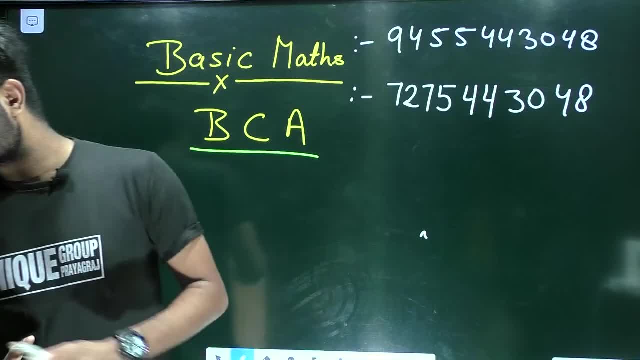 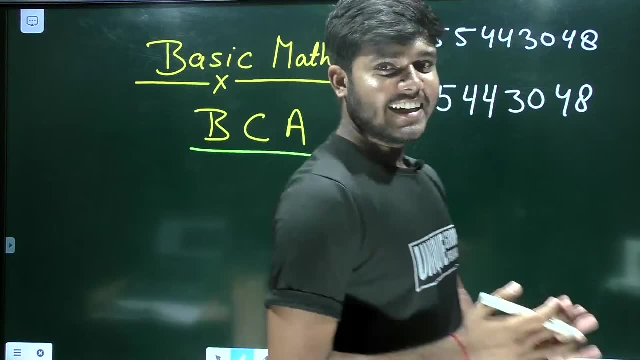 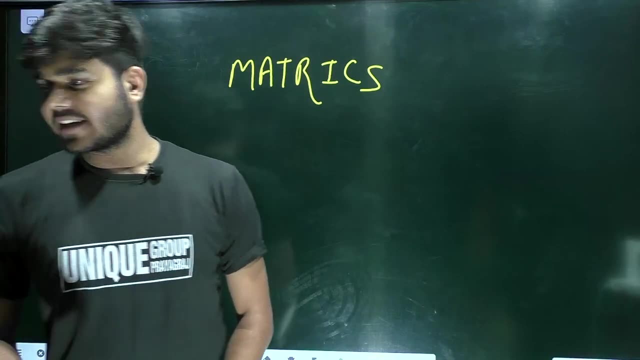 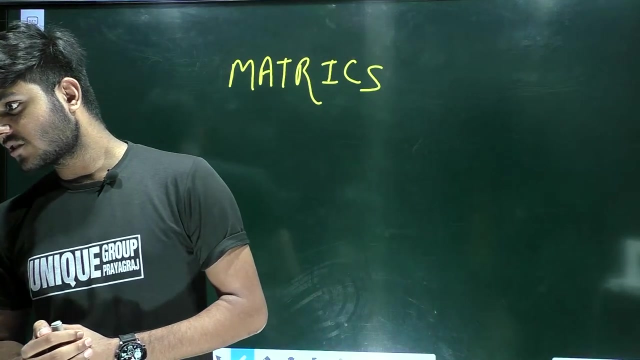 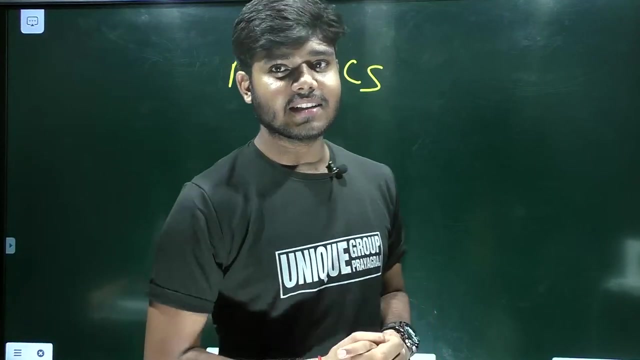 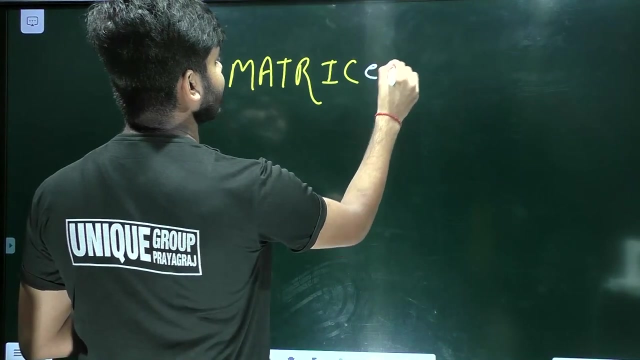 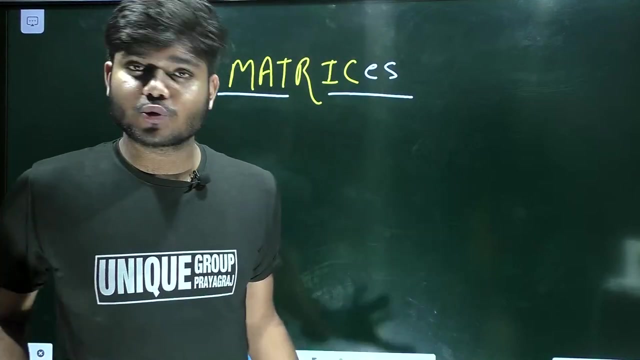 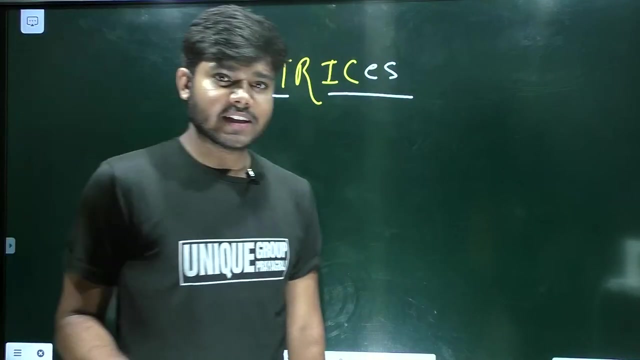 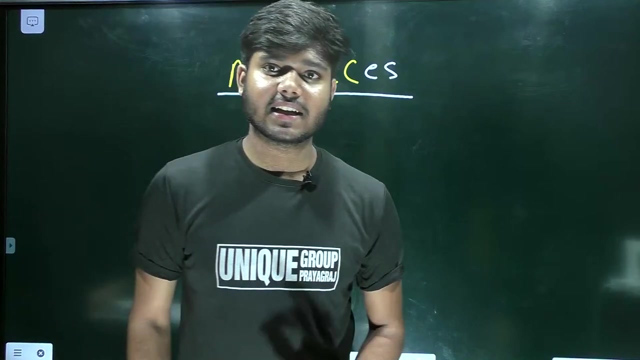 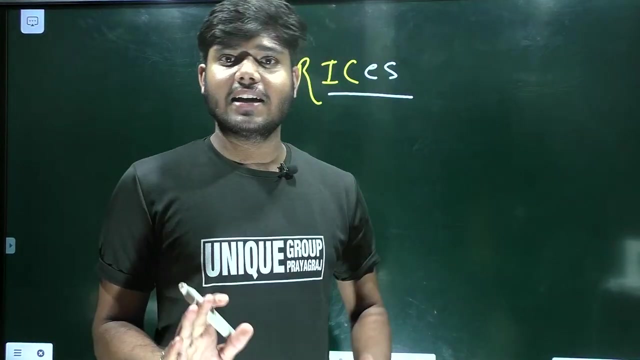 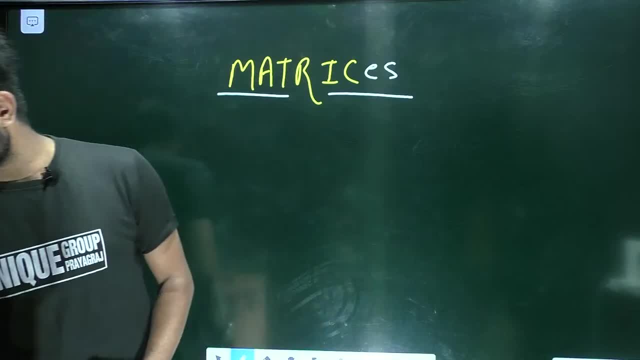 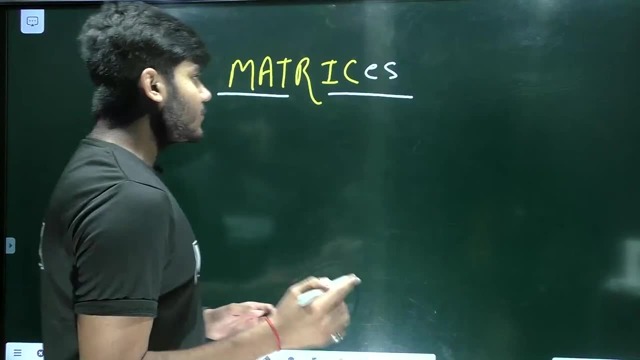 Those who don't understand will ask Any problem. We know matrices. Megha Kumari is a very good speaker. We will put up the questions and you will answer them. First of all, let's know what matrices are. What is matrices? 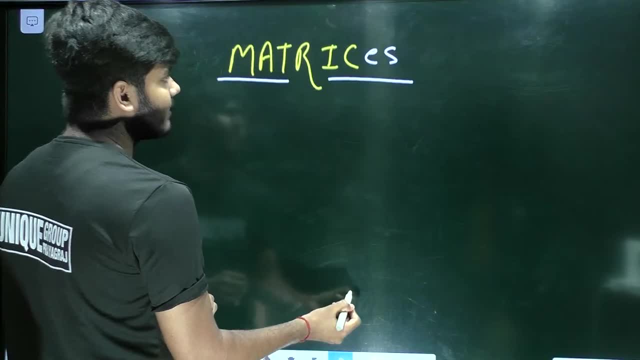 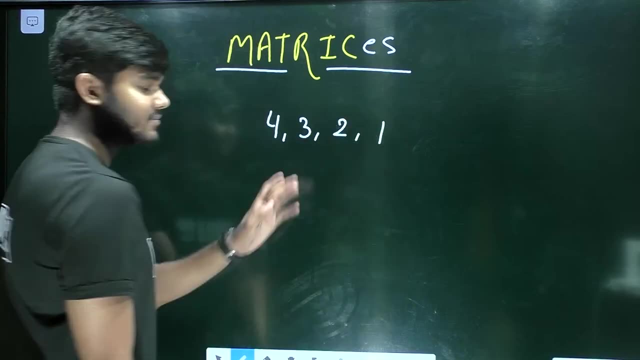 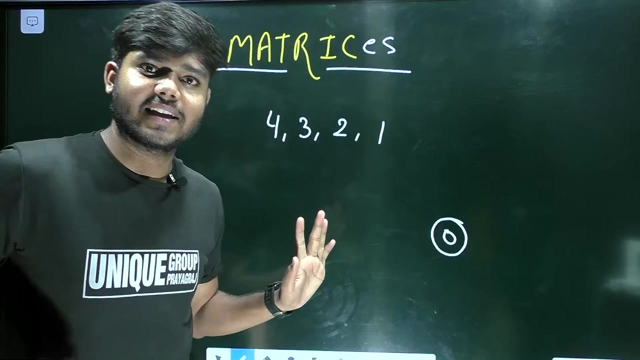 Suppose we take some numbers. Let me tell you the basics. Suppose we take some number: 4, 3, 2, 1. I am telling you from zero level. If any child has a certificate, he will also understand, Understand this. But on the basis of this. 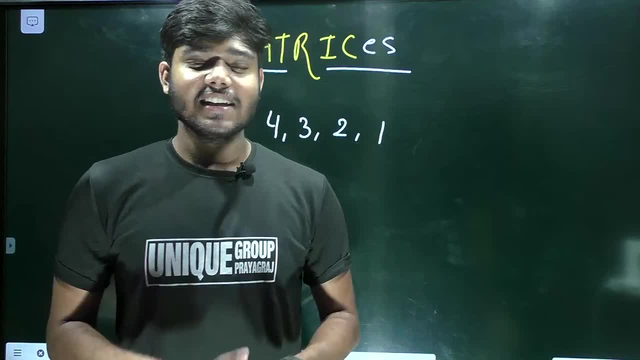 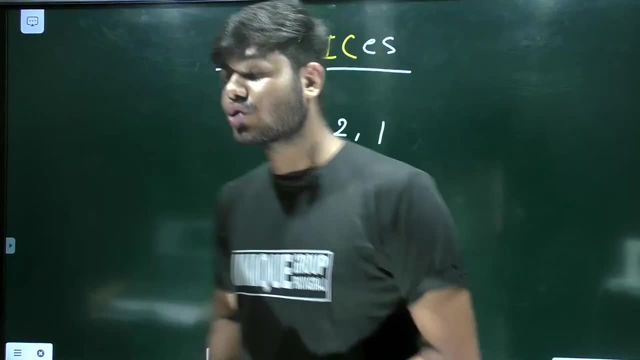 don't say that BCA Mathematics is like this, Because we are starting from zero. There will be a new extreme point Where you will also get a little hard. Some theorems will come. The theorems will fill the whole board. 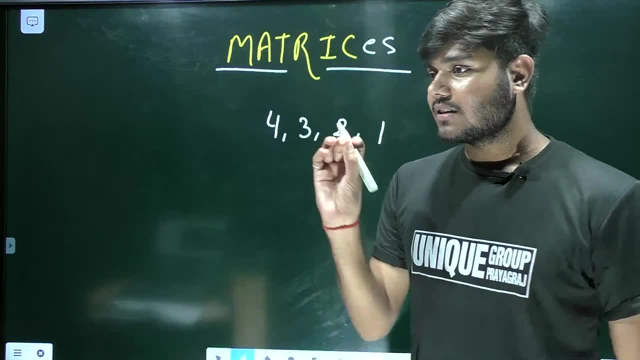 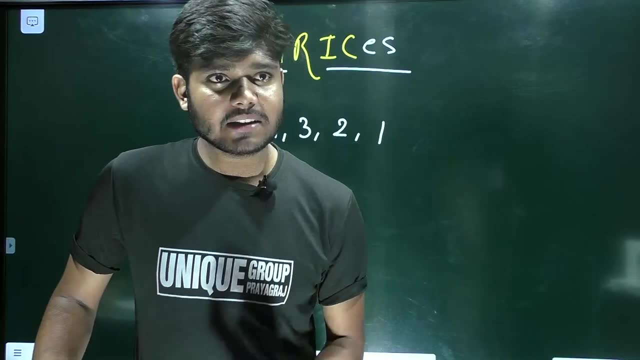 And you will study very easily. You will understand everything, But this is the only condition. Whether you are at home or anywhere, Do revise it once again. Mathematics is such a subject. If you don't revise it, the day you remember it. 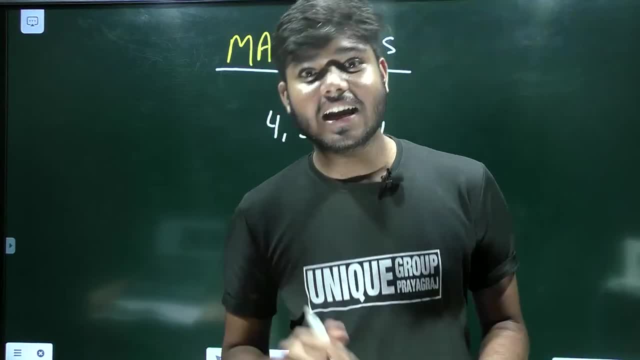 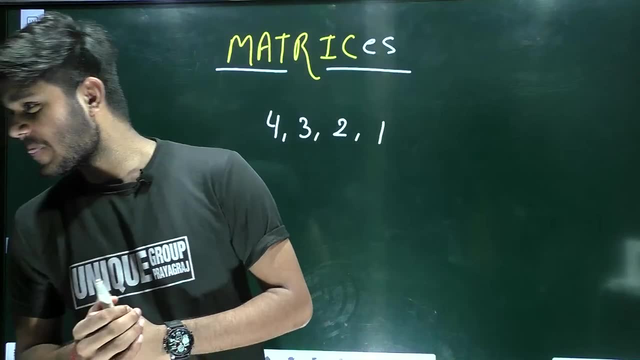 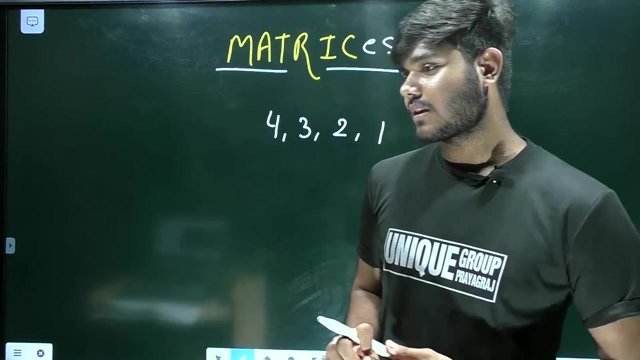 you will be amazed, But if you don't revise it, you will abuse your head And you will be worried yourself. Okay, Telegram is not opening. Okay, It will happen. There may be some network problem here. There will be some conditions. 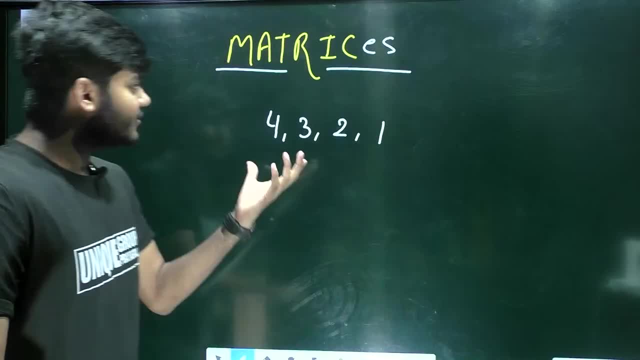 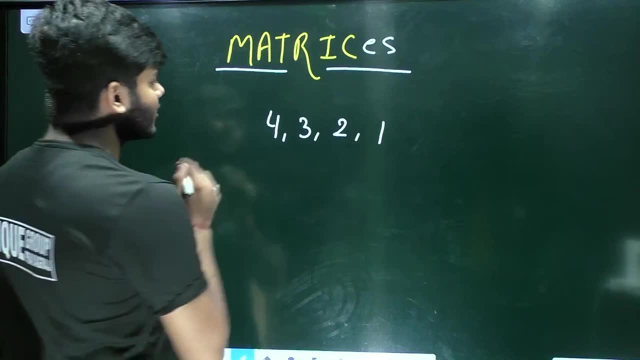 There is no problem, Telegram will also open. Let's move on to the class. What did we say? 4, 3, 2, 1.. We have some data or some numbers of the video. How can we write this? 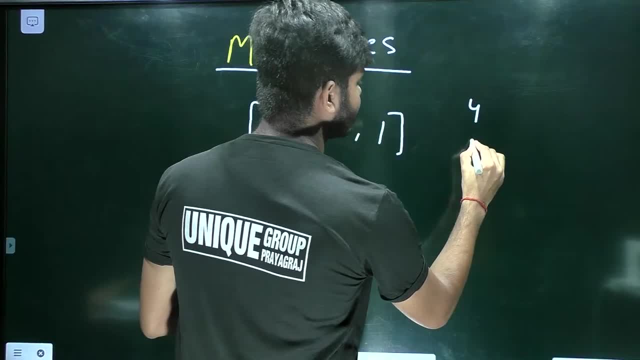 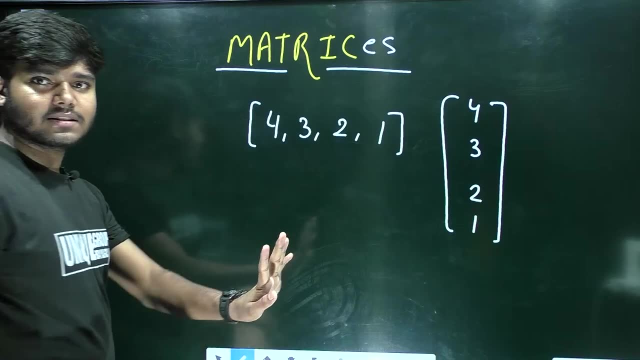 We can write it like this: No problem, We can write it like this: 4, 3,, 2, 1. We can write it like this: No problem, We can write it like this: 4, 3,, 2, 1. 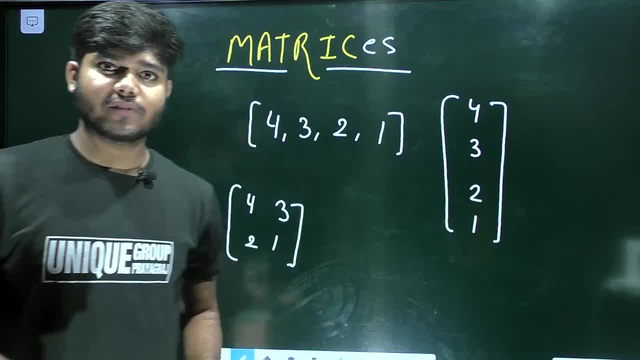 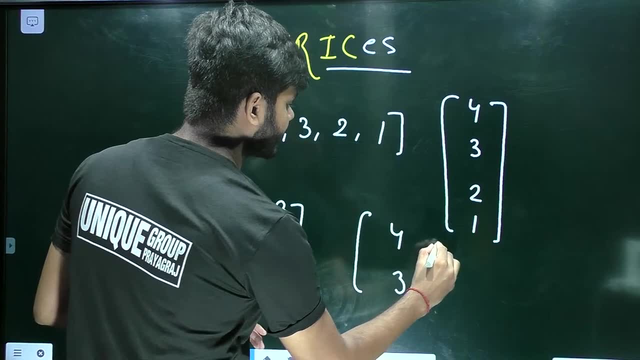 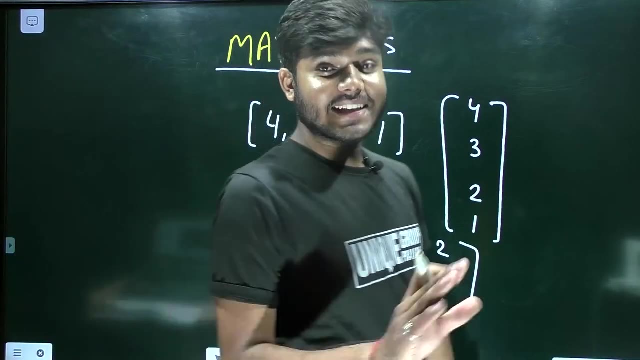 No problem, We have the same data. We just changed the writing method. Is it clear? We can write it like this: 4, 3, 2, 1. Okay, Okay, All of you. please like and subscribe. 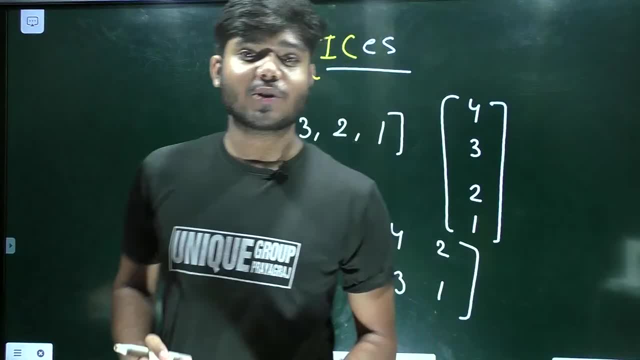 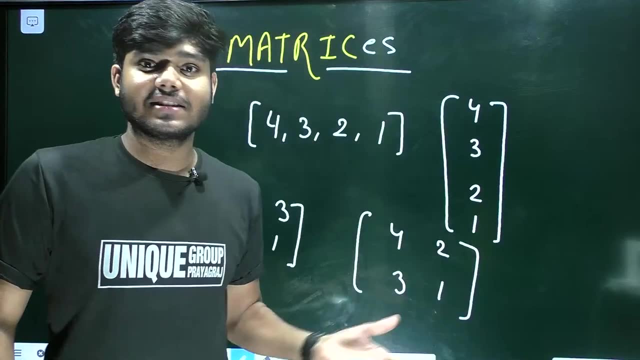 We will have a great session, Okay, And then we will make you a friend. There will be nothing too scary, Even if you can't understand or if you are facing difficulties. There won't be any such thing That I can't understand. 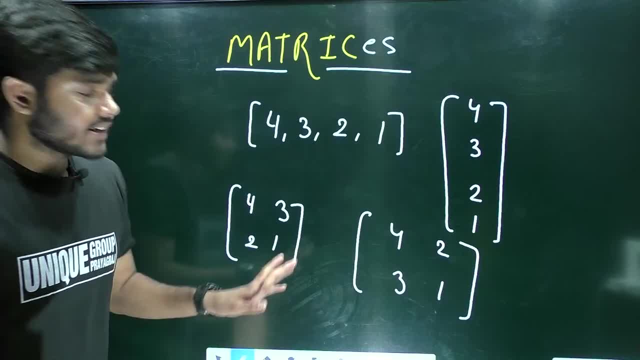 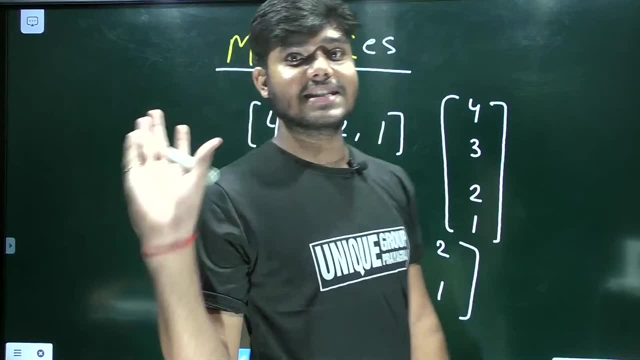 Nothing that you can't understand. All that we have to do is that we want you to explain it. Now we have her 4, 3,, 2, 1.. Now we have arranged it in different ways. What is a matrix? 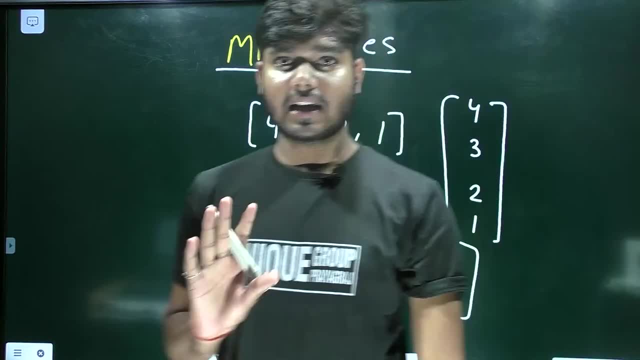 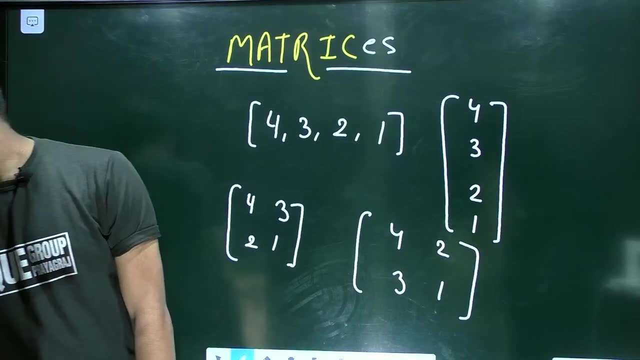 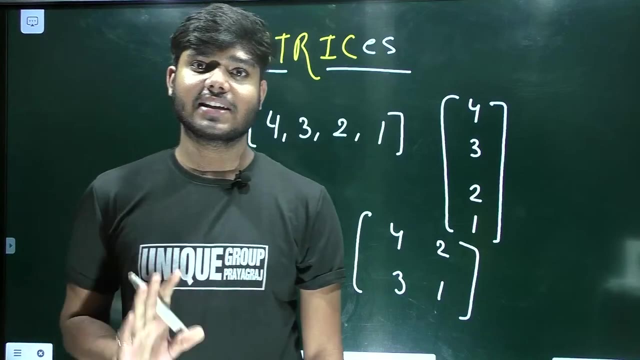 Matrix is a writing that exudes pentagons. You know what is rectangular? No, You will get the full math on YouTube, don't worry. you just read it with your mind. okay, you just read it with your mind. you see, come towards the class. okay, you will read. 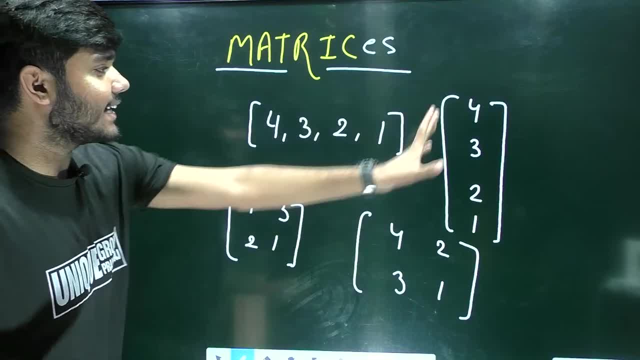 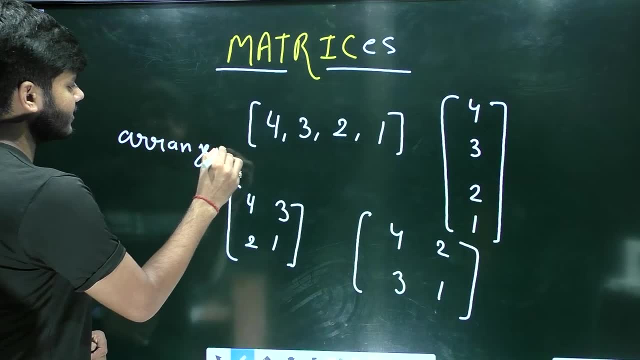 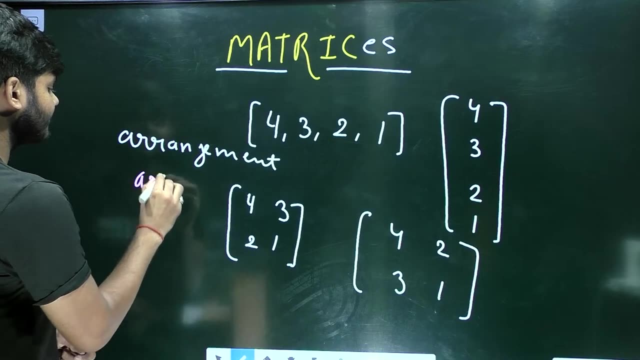 in the comments, see what we said. we said 4,, 3,, 2, 1 in a rectangular arrangement. in arrangement, see there is one word: arrangement, okay, arrangement, and for this we will use one more word. for this we will use one more word, which is called array. you will say: 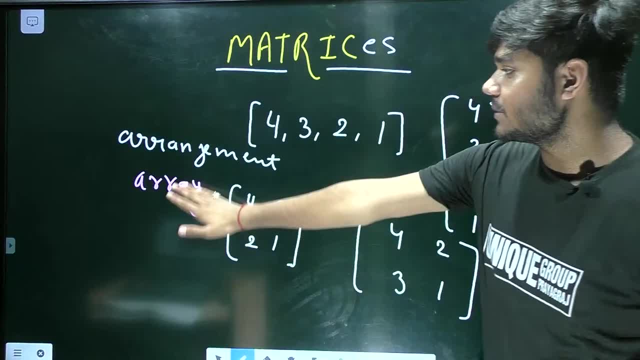 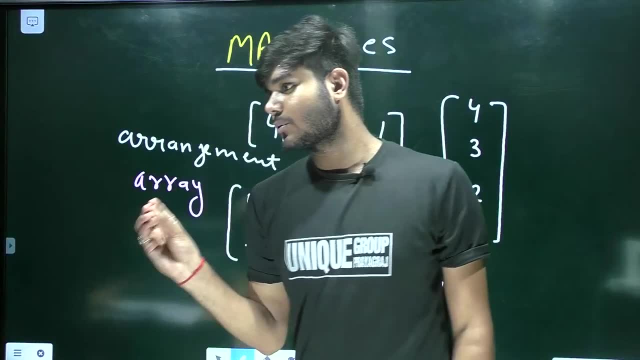 sir, what is array? what is array, then? array is called in Hindi. what is called sorry sarni, sorry sarni, what is called sarni is called sarni means you will know it very. 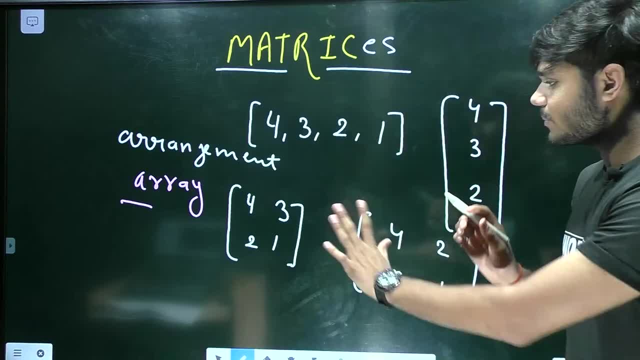 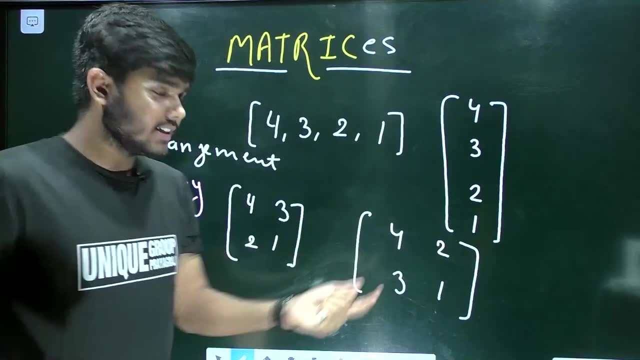 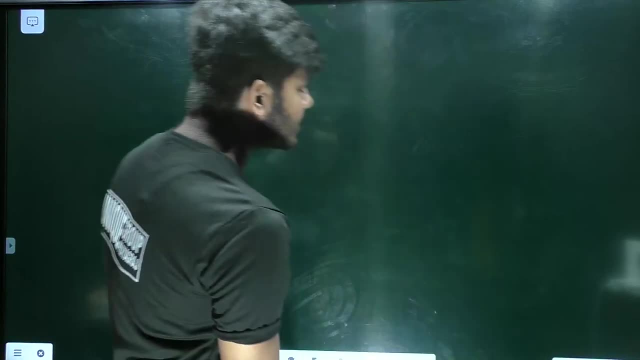 well, right, right, this is sarni. we are making sarni, okay, so what is matrix? when we keep the data in a rectangular form, then that arrangement is our matrix, right? so that time it is called matrix. attention, what is our arrangement? 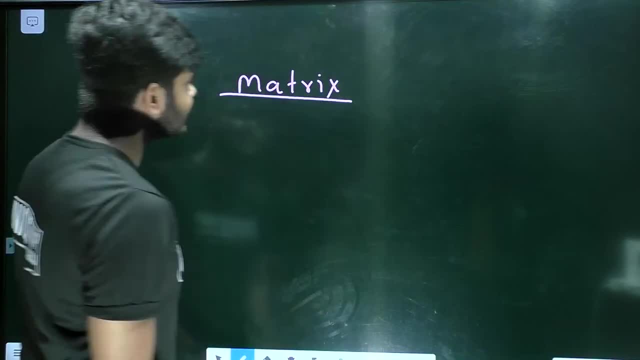 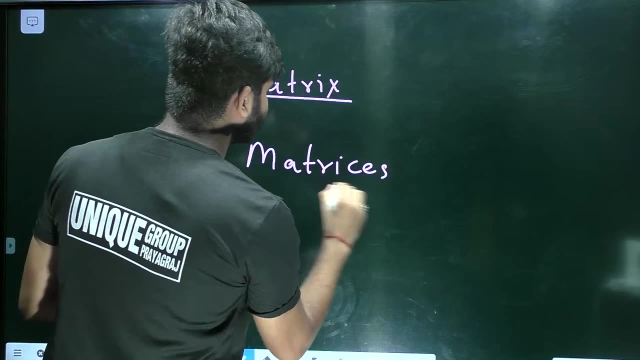 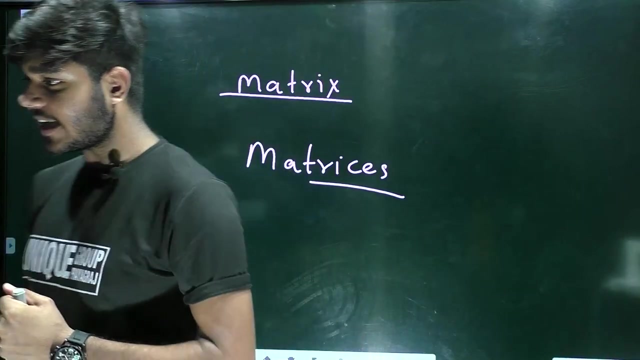 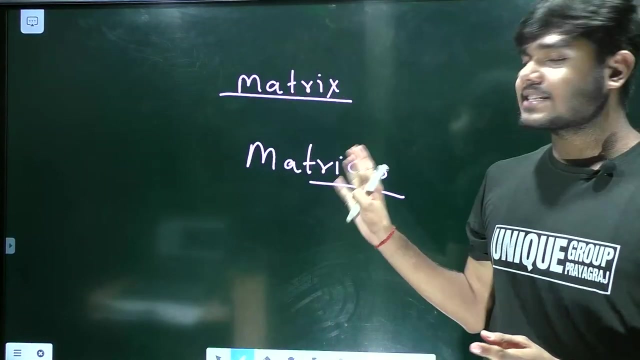 Brother, it says matrix. you will say that, sir, you said was matrices. now I am telling, are the differences two? both are not same. see. see, brother, what ie those people? What is the difference between matrix and matrices? 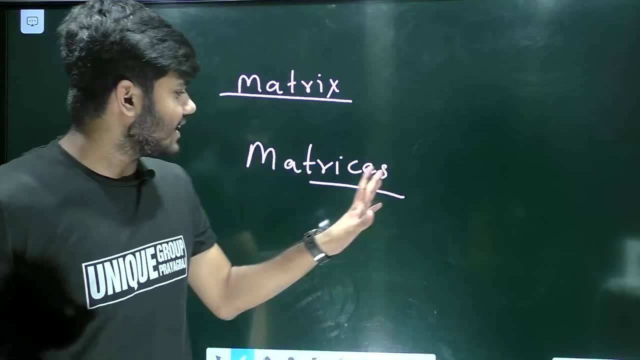 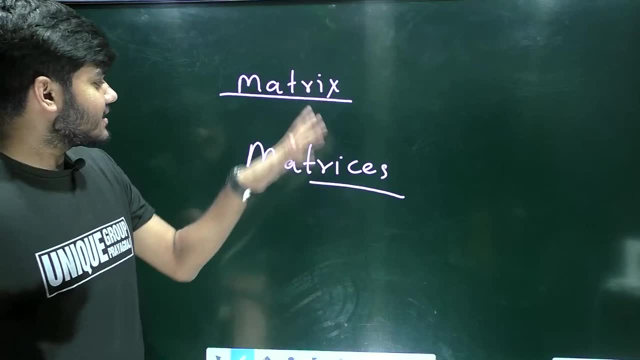 There is no problem in Maths. Here you can see that we are starting from zero level. If a child of 6th or 7th grade will also study, then he will understand So quickly. tell me what is the difference between matrix and matrices. 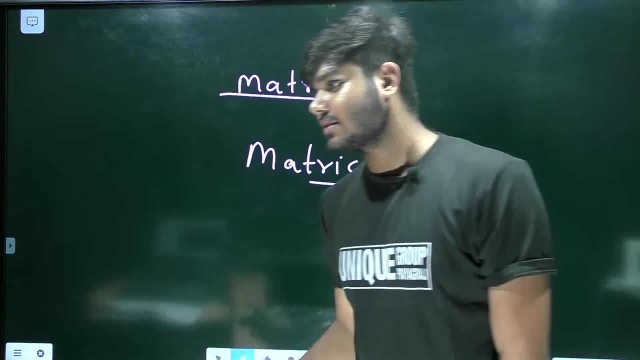 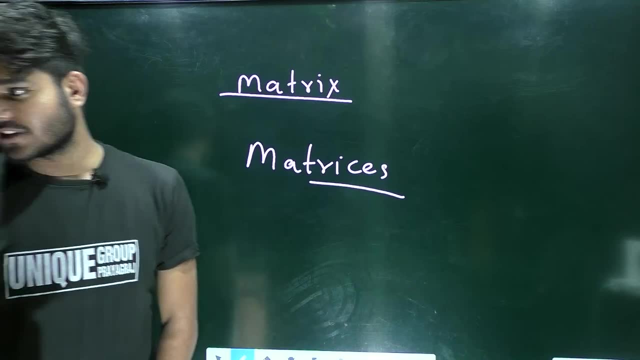 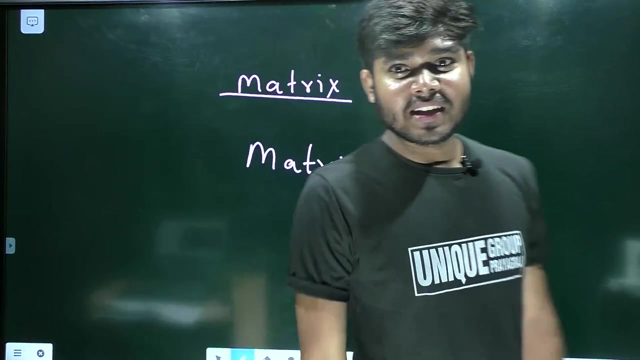 Arrow of elements is absolutely correct. Any data can be given to you. There is no problem in elements. Matrix is plural and matrix is singular. Mega Kumaris is absolutely correct. The only difference is that if there is one arrangement, then that is matrix. 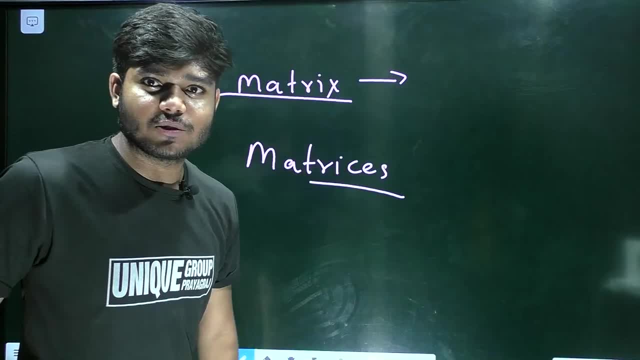 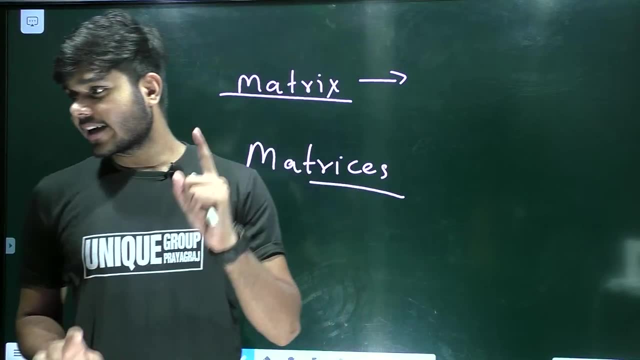 If there is one arrangement, then that is matrix, But if we put two or three matrices together and talk about both of them together, Do you understand? If there is one matrix, then that is matrix, But if we talk about two or three matrices together, then that is matrices. 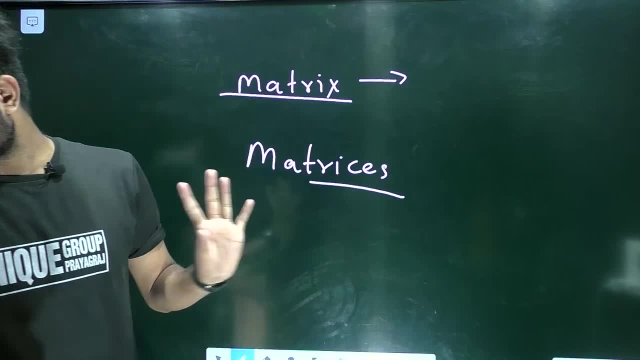 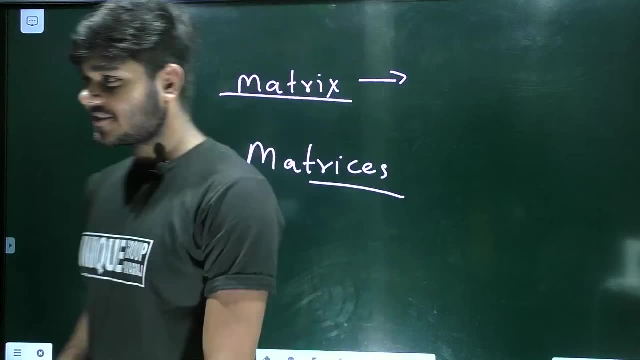 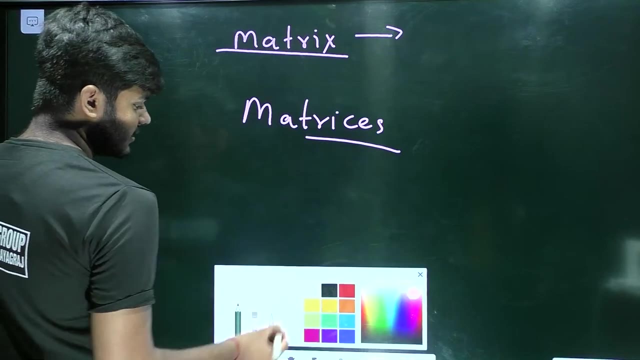 Group of matrix is known as matrices. Very good, Very good, Mega. Do you understand? Now let's talk about elements. Let's talk about elements. Suppose we have formed a matrix. This is how it is made. This is how it is made. 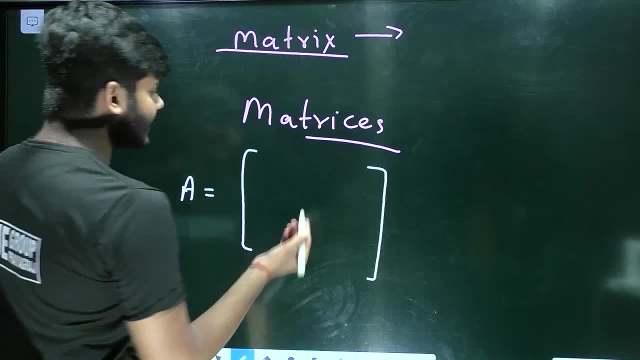 Rectangular form. We have taken this data. Suppose we are going to make 4, 3, 1.. Let's take 4, 3, 1.. 4, 3, 2, 1.. Let's take it here. 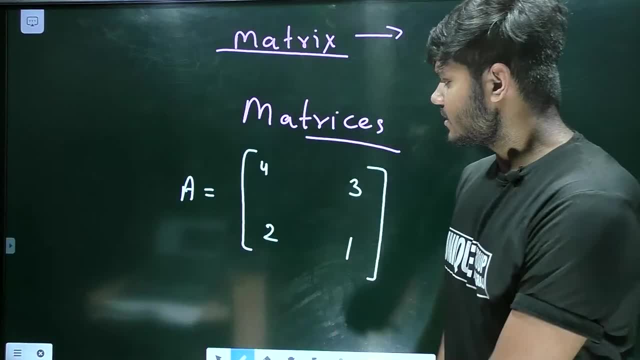 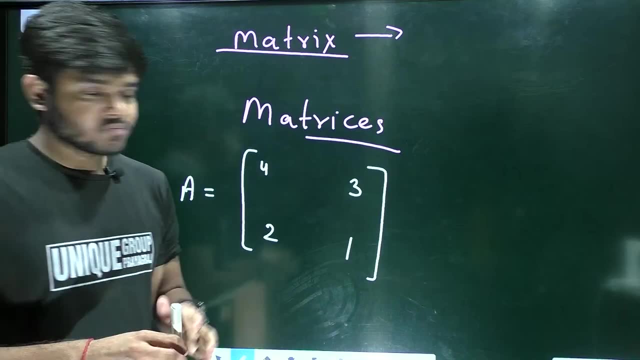 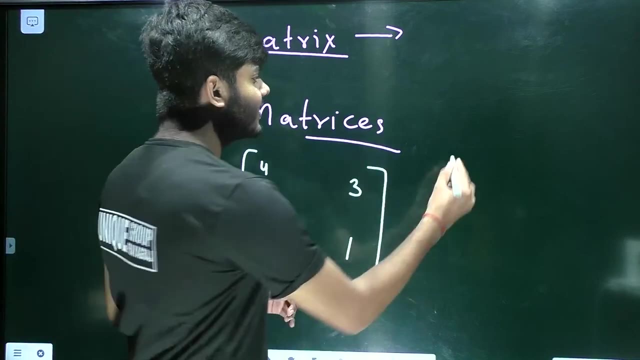 Does it mean to understand? It means to understand. Those who don't have math or commerce can understand. Okay, See. Then what are we saying? We have written this data, The data we have written. This is called an element in the language of matrix. 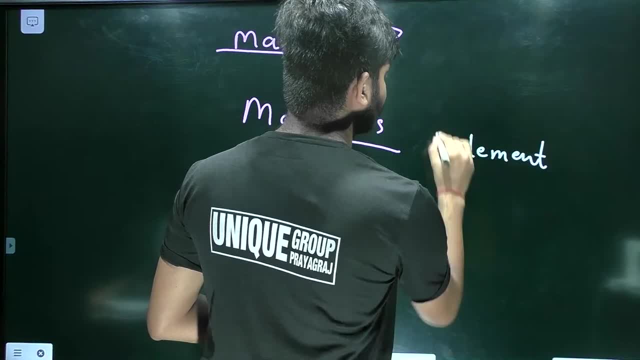 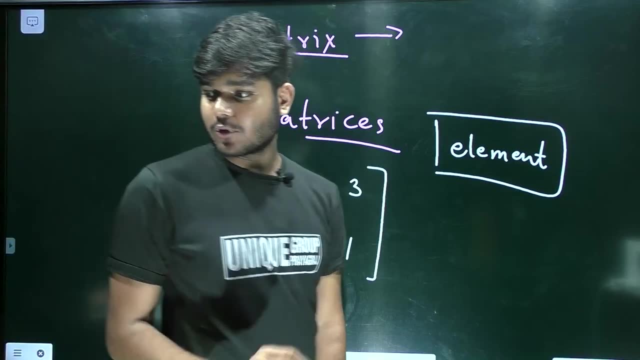 What do we say, dude? It is called an element. Do you understand What do we say? It is called an element. You guys can comment in between that from where you get it. If you understand, then give thumbs up also Okay. 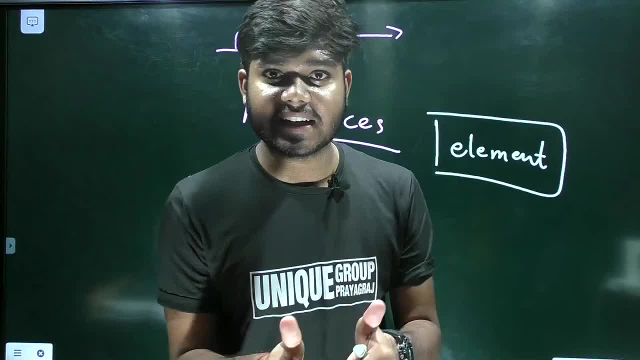 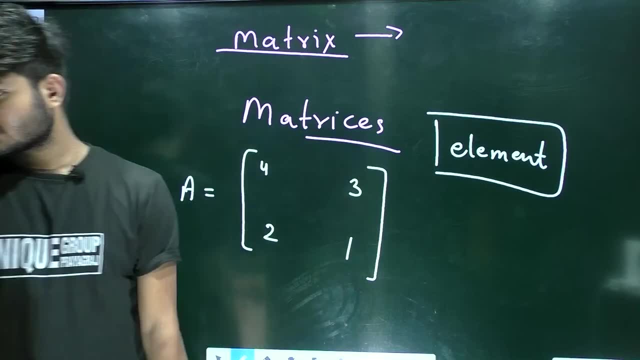 Or even if you think, whatever you are trying to study fast or you are less, then you should tell: Okay. Okay, Now see what we said. This element that we have written in the data, what is it? It is called element. That means that this element is called element. 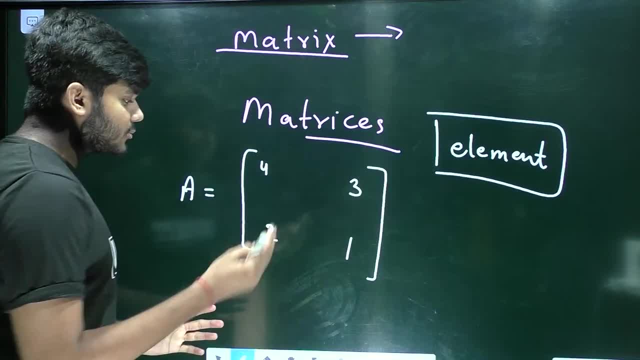 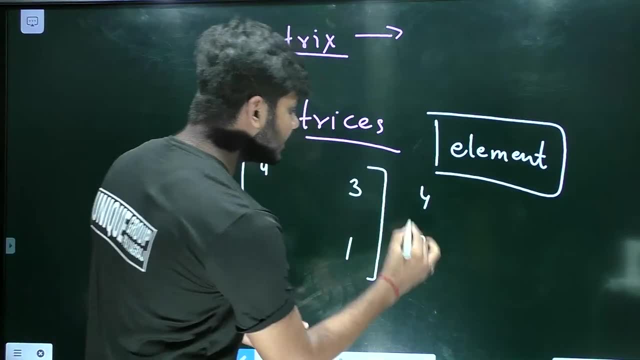 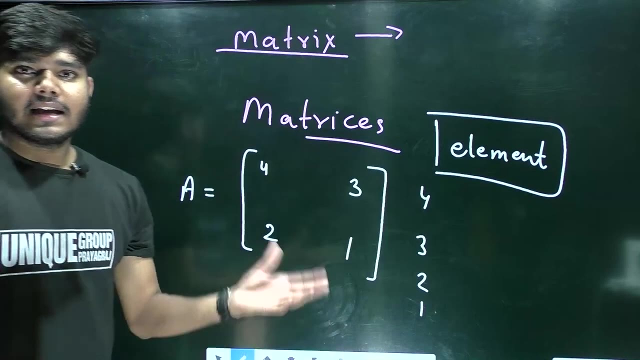 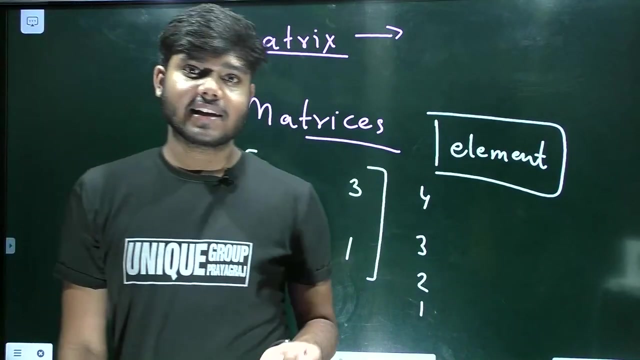 Yes, If we ask which are the elements in matrix A, one is element 3, one is element 2, one is element 3, one is element 4, one is element 2 and one is element 1.. Okay, tell me one thing: wherever you are from, like if you are from Uttar Pradesh, Bihar, Patna, Allahabad, Padayagraj, wherever you are from, we tell you that this gentleman is from here. 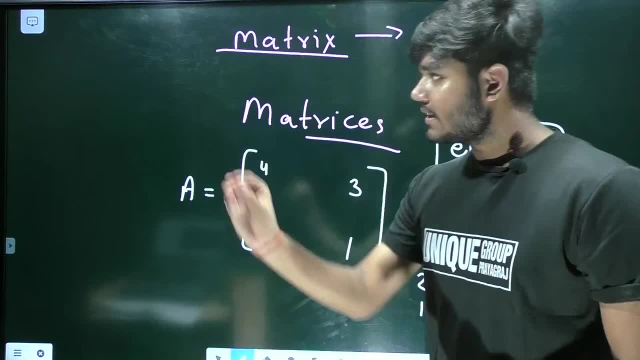 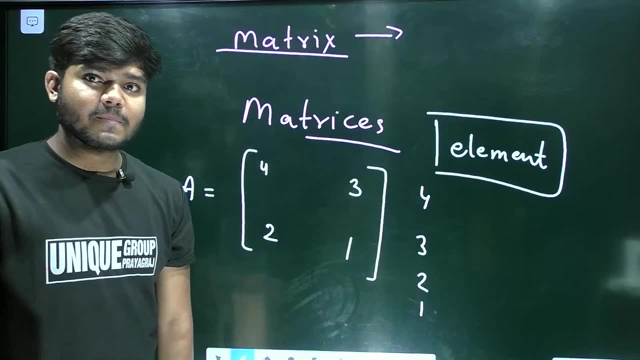 This gentleman or this madam belongs from here. What do we tell them? in particular, We tell them the place where they live. So when we write 4,, 3,, 2, 1 here, we have to tell them the place as well. 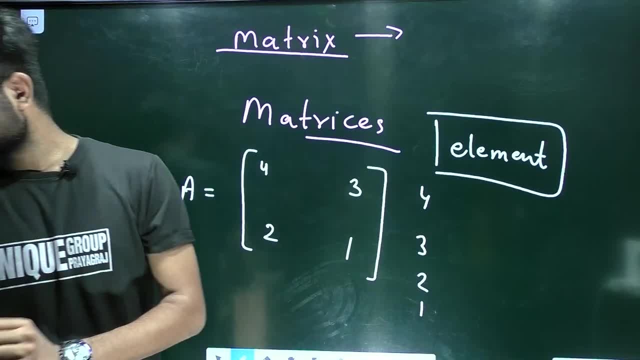 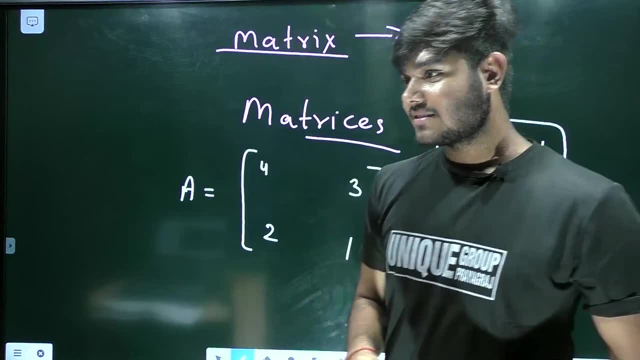 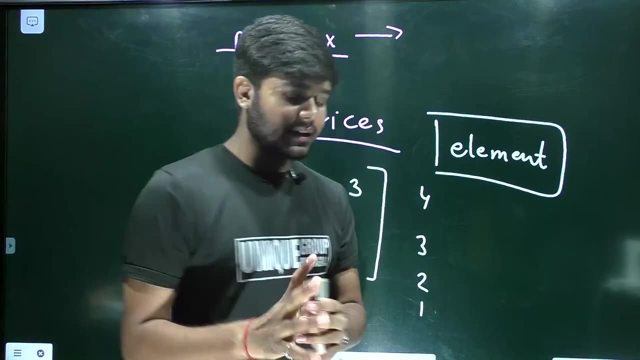 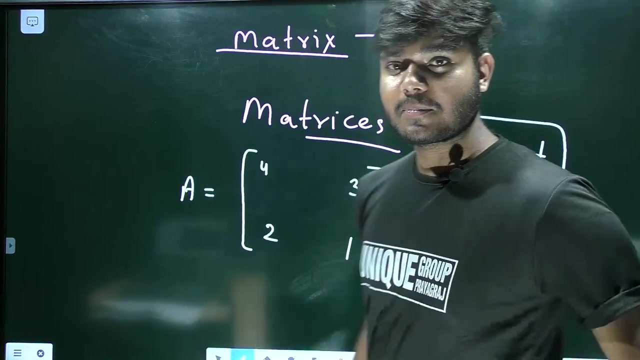 Where do they live? Okay, If we tell them that this house is there, Let's take someone's example. Let's assume that Megha ji is from Banaras. If someone asks where Megha ji is from, what will they say? They will say that Megha ji is from Banaras. 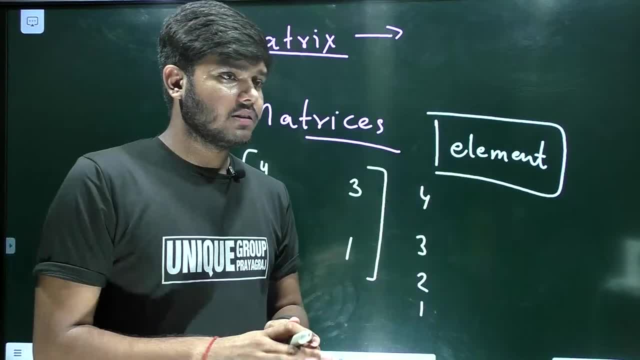 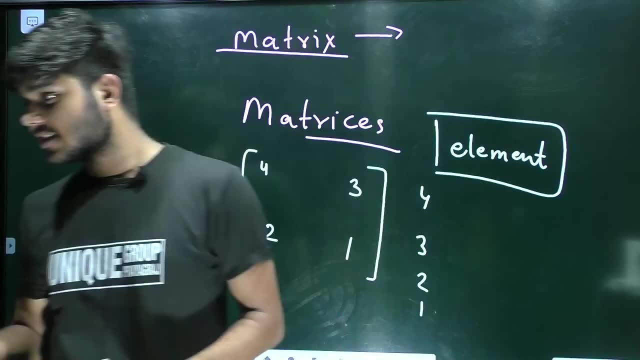 Okay, What happens? in particular, All the students in the Unique Online group, all the students ask where Megha Kumari is from. So what will they say? They will say that she is from Banaras. There are many other students like this. 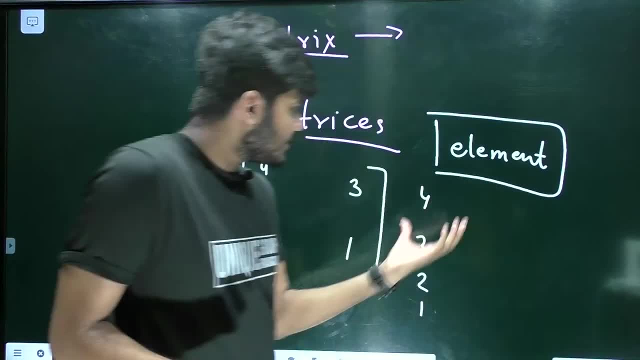 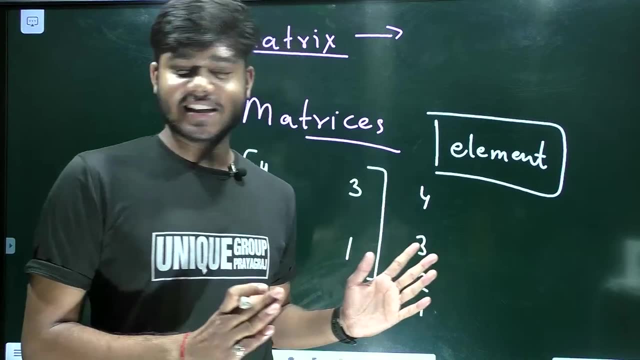 There is Abdul Bhai. Okay, So what do we tell them in particular? So it will be necessary to tell them the place as well. See those who have read it. it may seem like a toy to them. Those who have not read it understand it carefully. 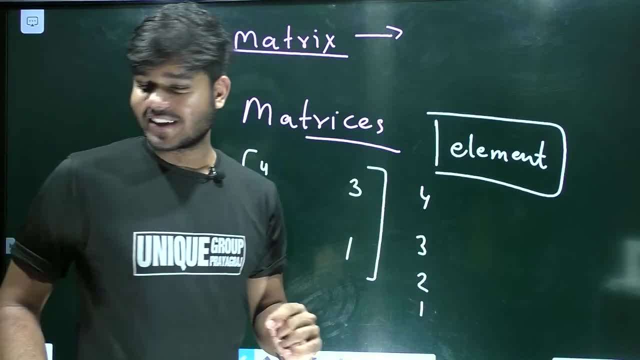 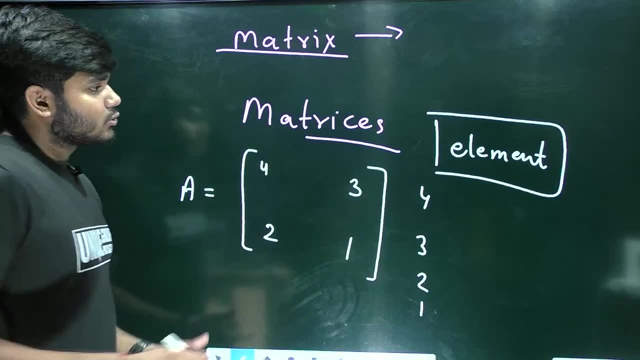 Okay, Maharashtra is here. Okay, okay, Let's see. So what did we say? As we have numbered here Right, So now we have to show these places as well. So we denote the element of the matrix with A. We are telling you in a very simple way. 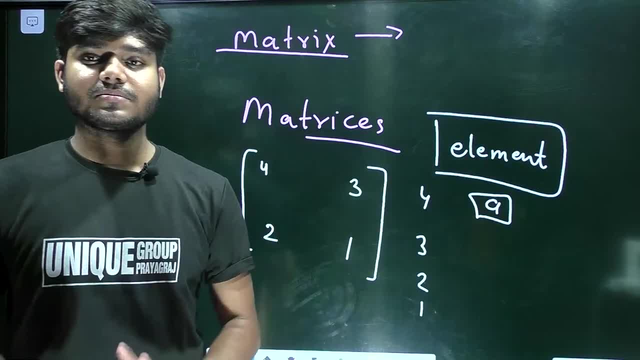 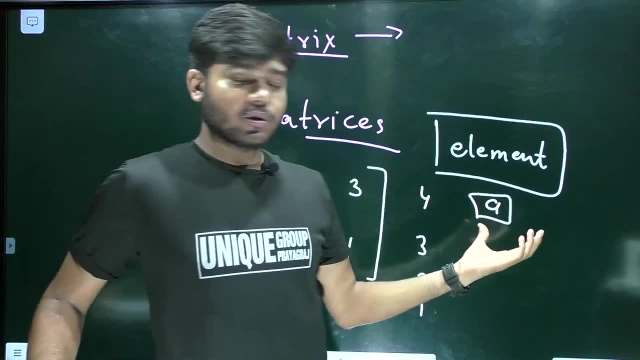 With basic things. We denote the element with A. To denote means wherever A comes. what does A mean? Element, The element of that matrix? Now you will say, sir, A is done, But A will not be A for everyone. 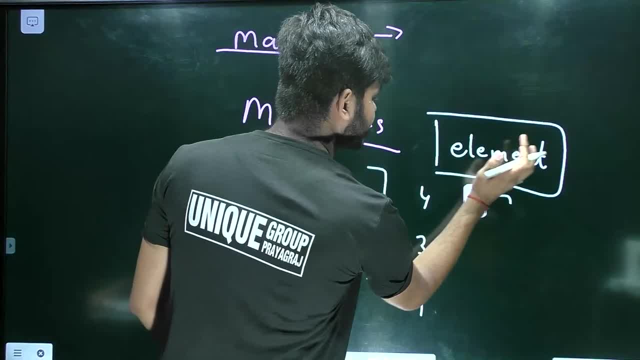 It won't happen right. It won't happen right. But what do we do for them? For them in the matrix: first we define row and column. Okay, First we define row and column, As we said, 4.. 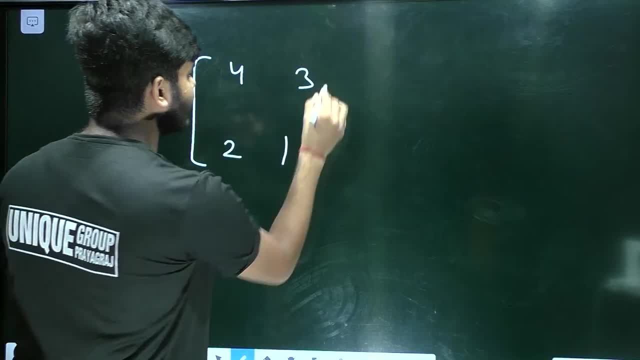 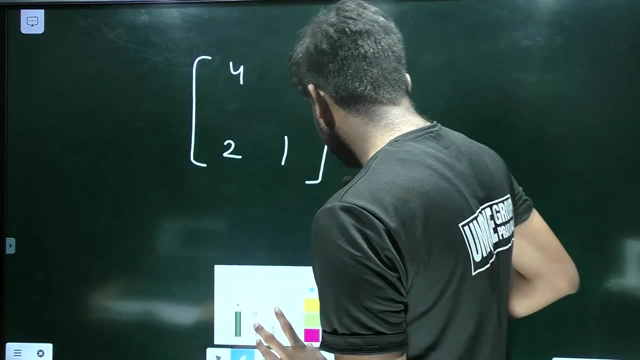 Three, Two, One. So what is row and what is column in the matrix? The most important thing, What is row and what is column? my friends understand it clearly. This, this, this, This is our row, right. 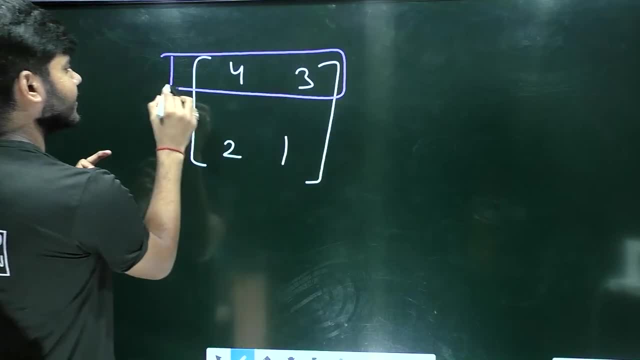 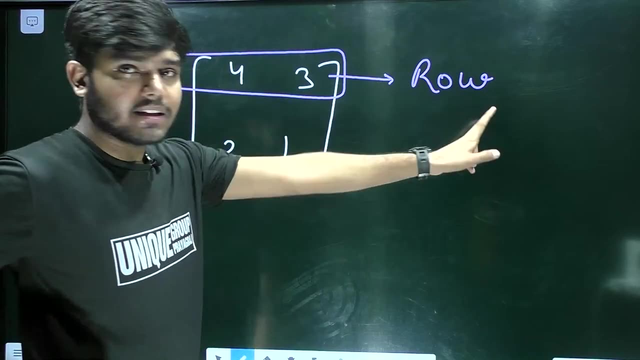 What is it? It is row. What is our A? It is row And, together with that, this particular line of ours. what is it? It is column. It is column, Right. It is column Right. What is it? 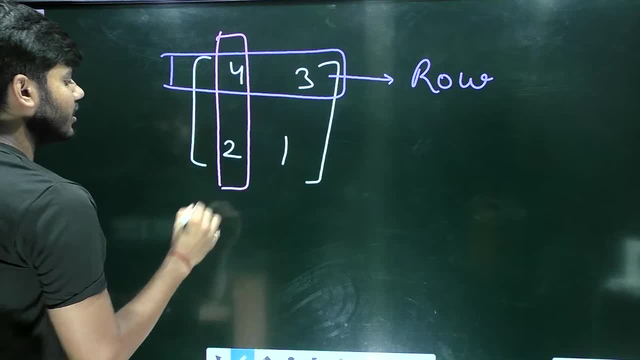 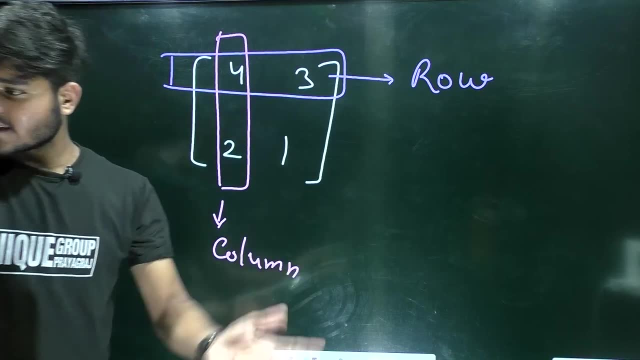 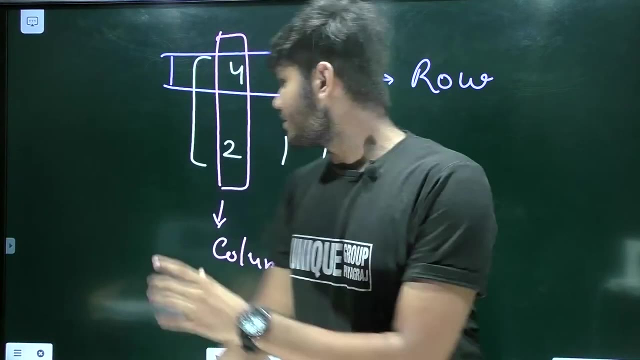 It is row. And what is it? It is column. Okay, What is it? It is a column. Understand the basics. I will give you more examples. Vertical is a row, Horizontal is a row, Vertical is a column. Don't get confused. 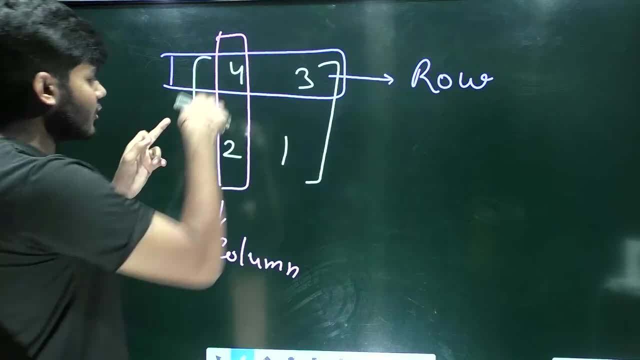 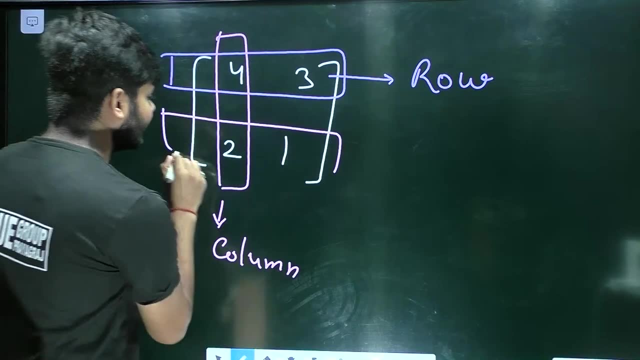 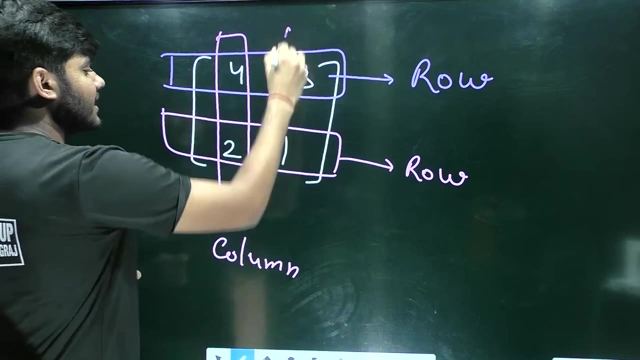 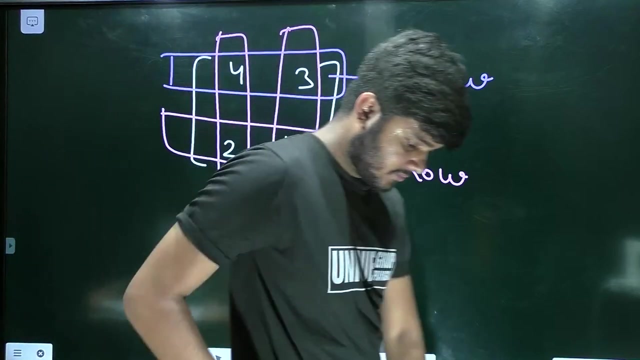 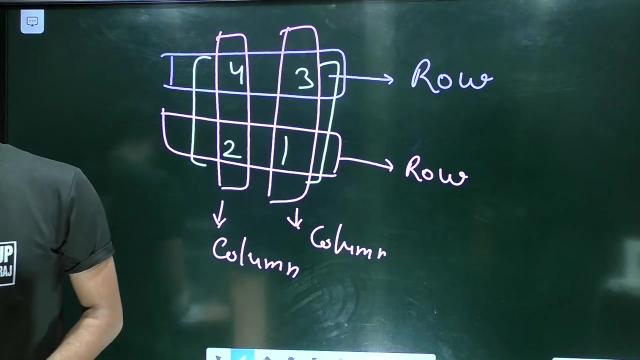 What did we say? This is a row and this is a column. How many rows are there in our matrix? Two rows. How many rows are there? Two rows? How many columns are there? Two columns? Do you understand? Two columns. 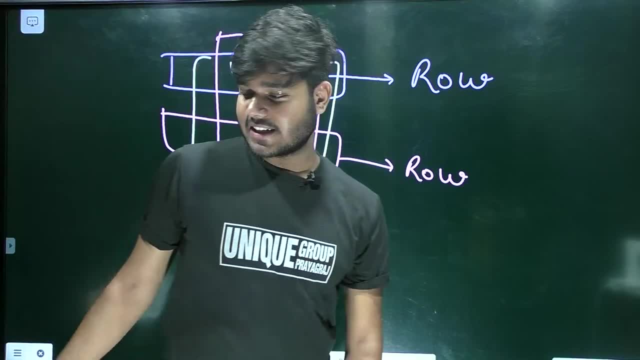 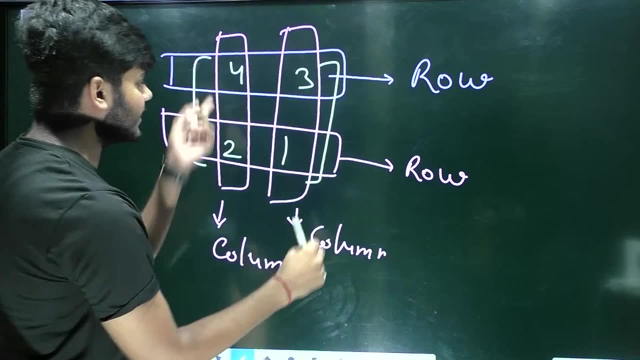 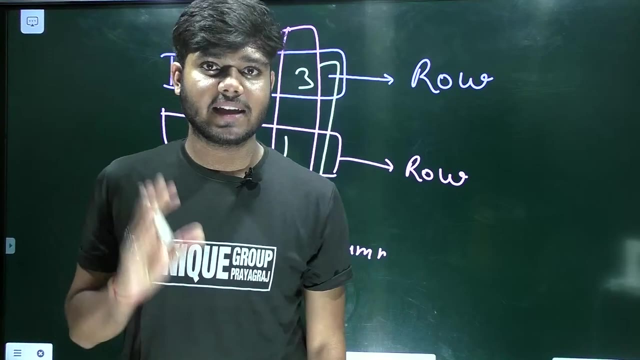 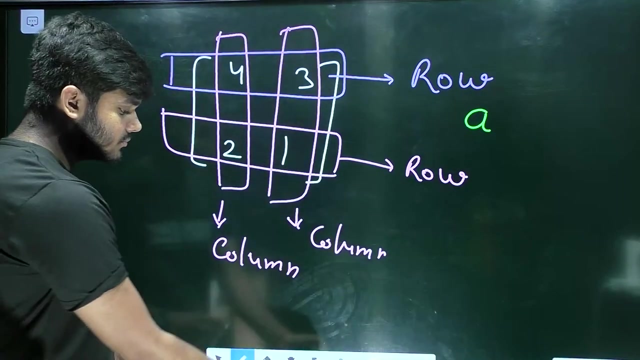 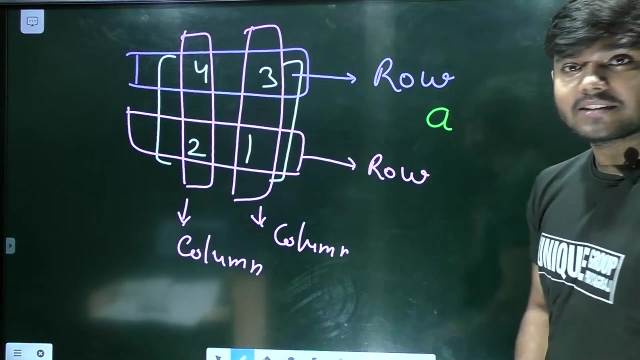 The sun is setting. Very good. What did we say? One row and one row To show the location of any element. how do we denote it? We say A, We will denote it with A. If we denote it with A, then we will not denote it with A. 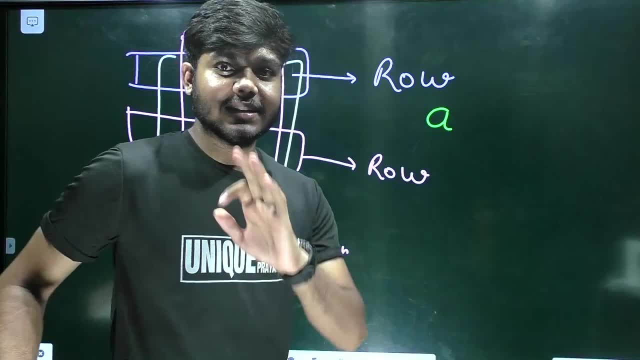 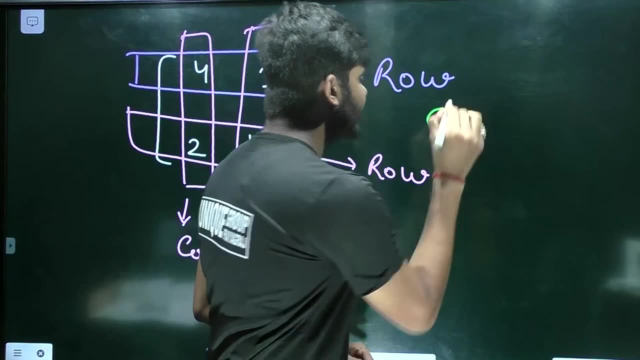 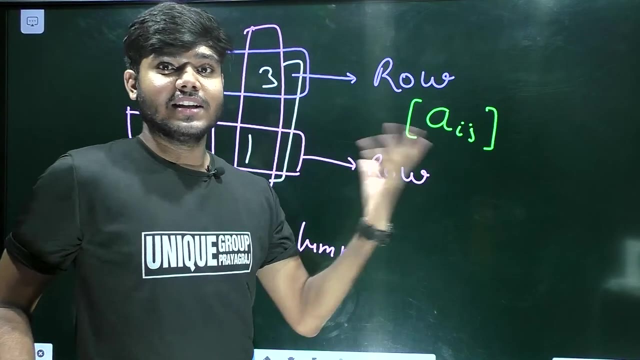 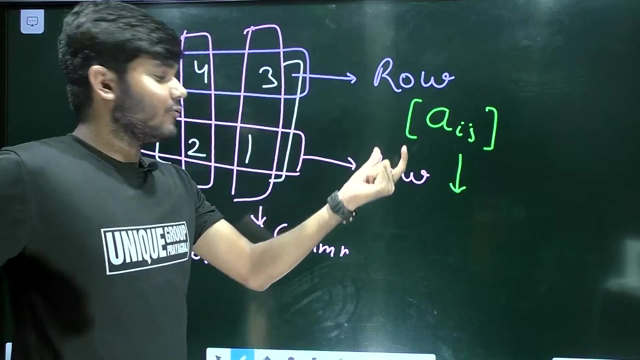 We will give it a particular location. What is the writing method? First you write I and then J. In this form, you will write any element. You will say: what is I and J? I means the number given by the element. In which row is it in that matrix? 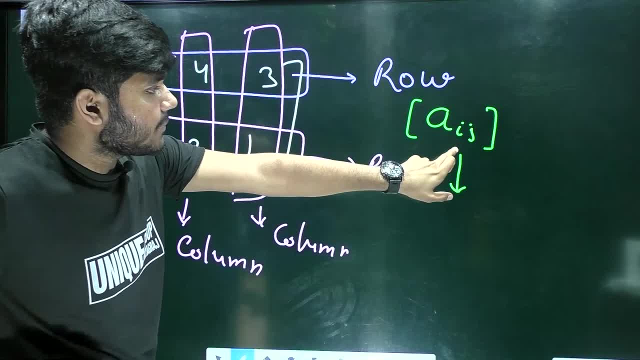 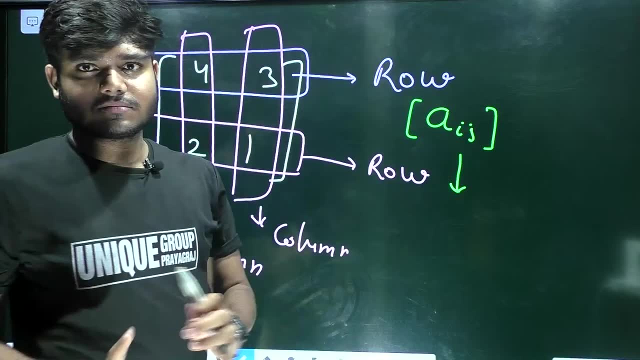 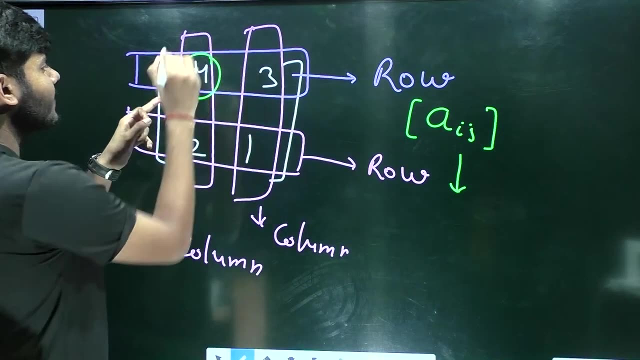 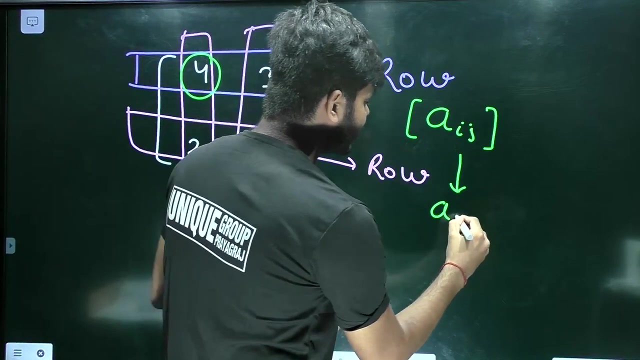 For example, it is 4.. What does I mean? In which row is that element in that matrix? It is very simple. What did we see? 4 is in the first row. What did we do in the first row? We wrote 1 in the first row. 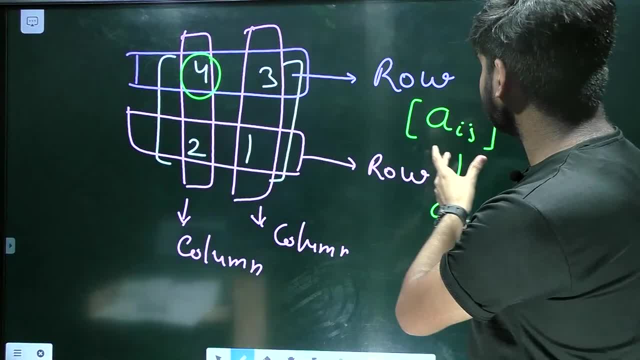 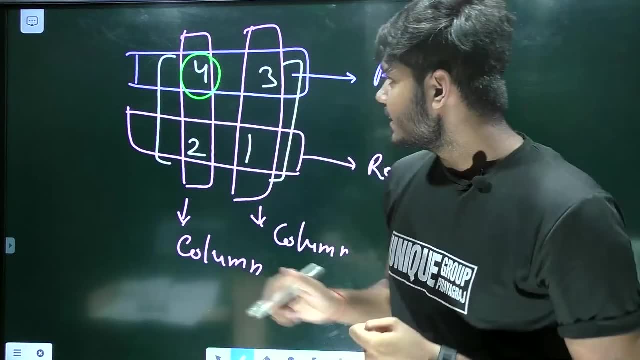 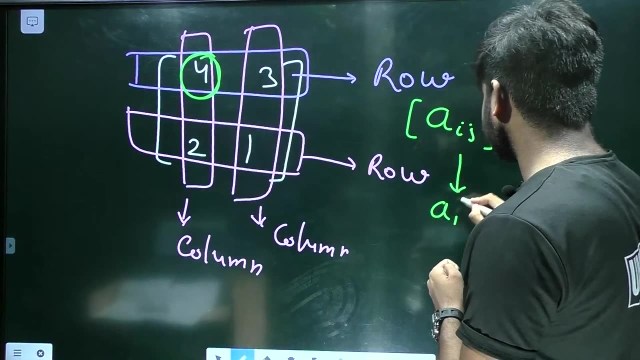 Then we said: what is J? J tells us that in which column is that element? We told the row: In which column is it? This is the first column. This is the second column. What is in the first column? It is 4.. 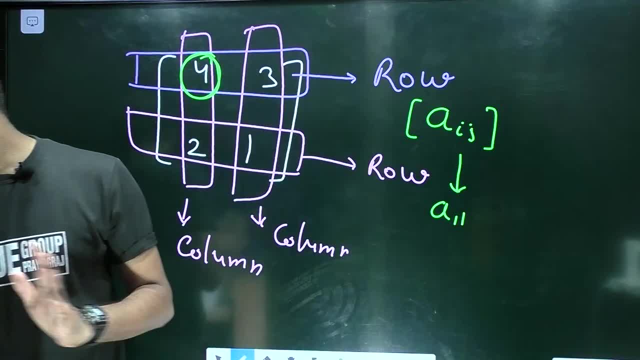 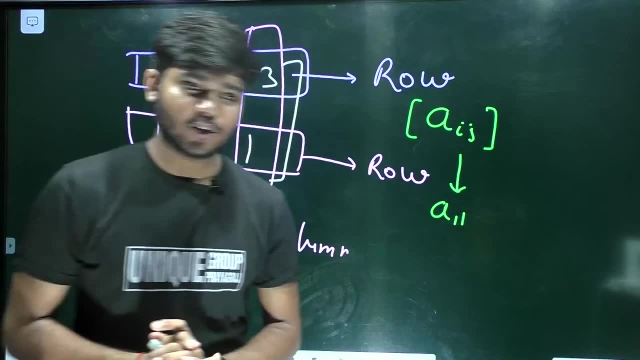 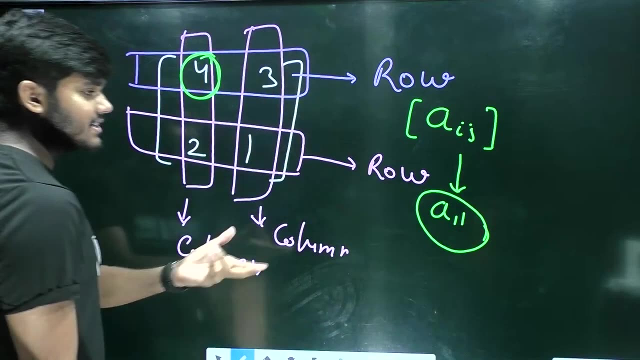 What is the value of J? 1. Is it clear? Is it clear? It is very good. What did we say? A11, A11, What is A11?? It tells a particular place for 4. Let's go back and you tell us. 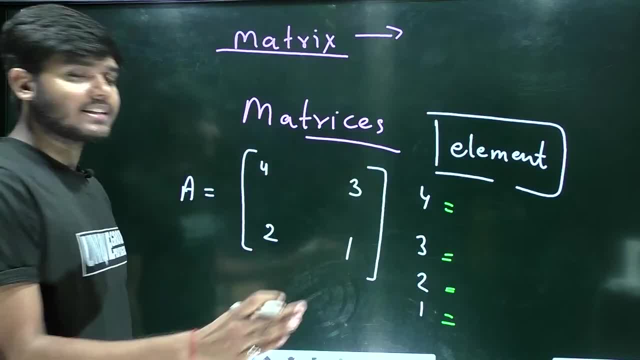 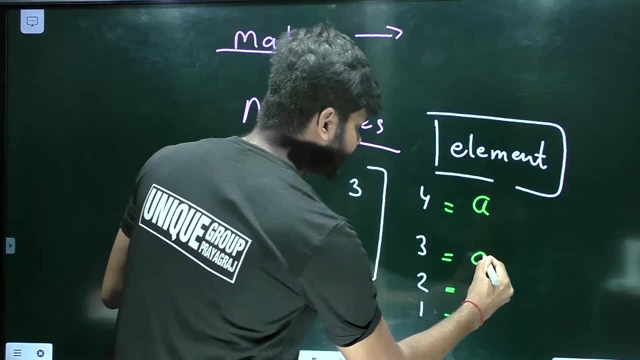 If you understand a little, you will tell us. If you don't tell us, there is no problem, We will repeat it again. What did we say? 4 is in the first row. Write A first. It is in the first row. 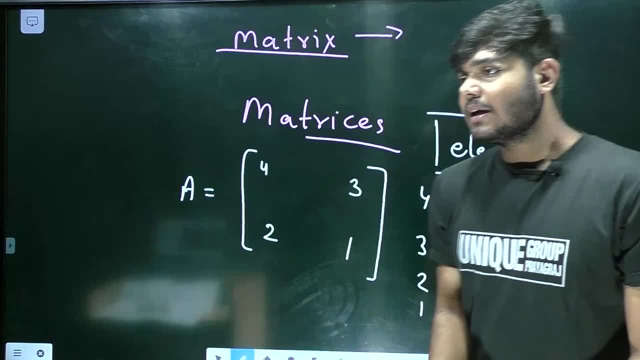 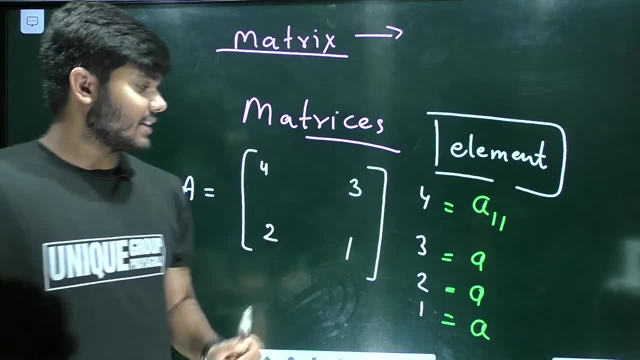 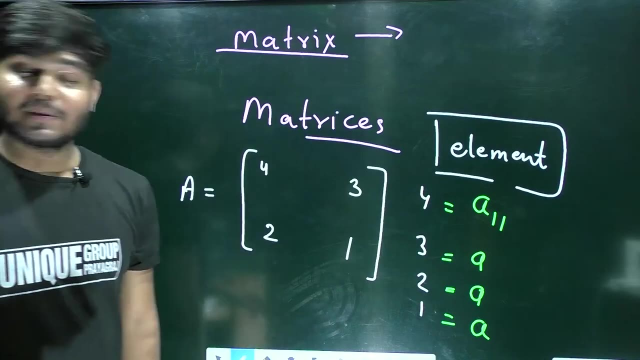 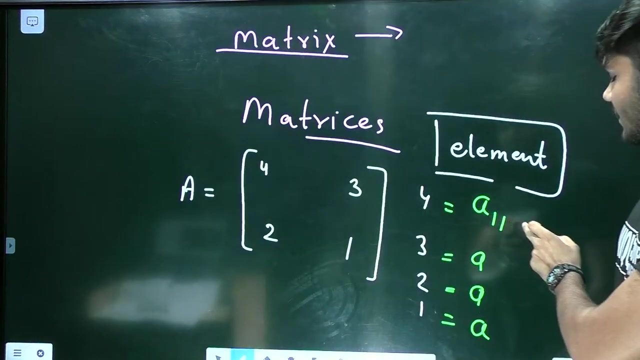 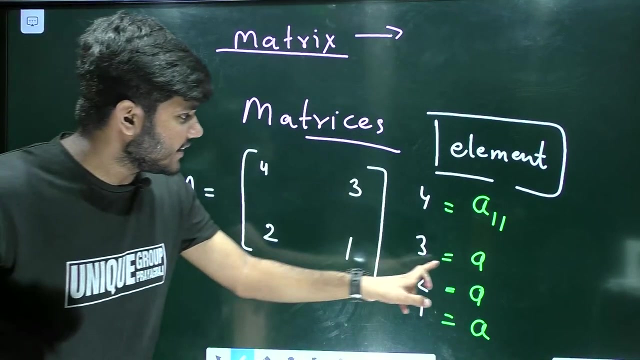 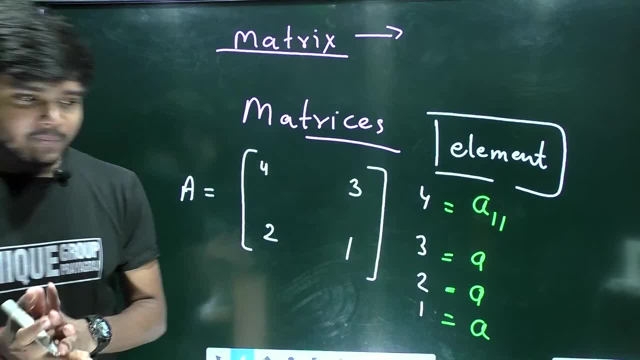 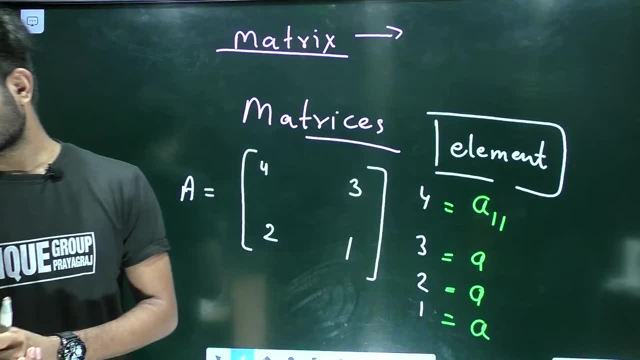 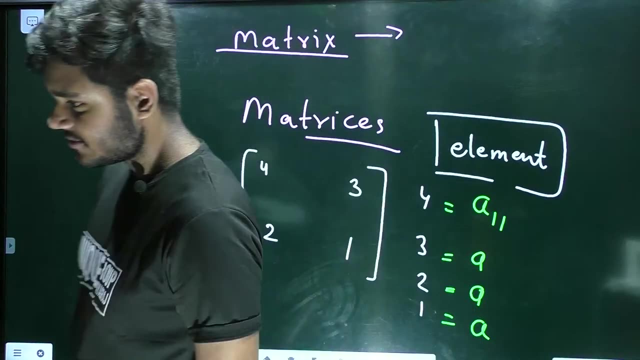 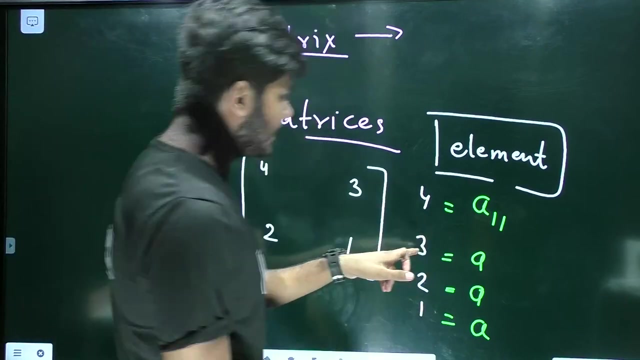 tell us the particular place, tell us fast, tell us fast. you only have 5 seconds. 5 seconds is enough. fast, fast, 5. 4. 3. 2. 1 ok done, very good. 1 ok, mix it. we are talking about 3, what i said. 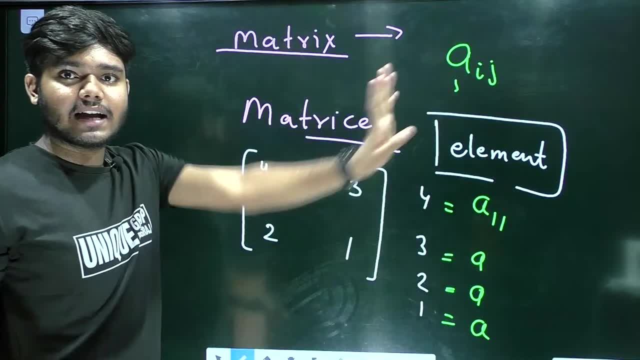 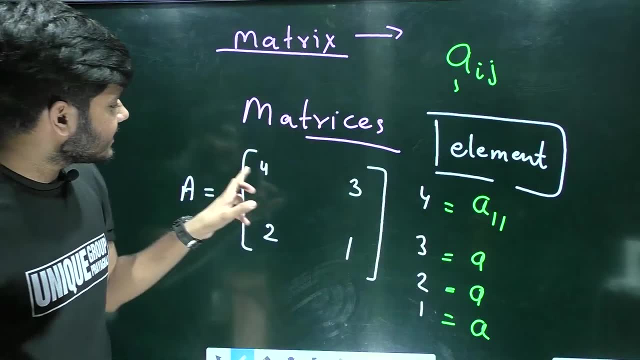 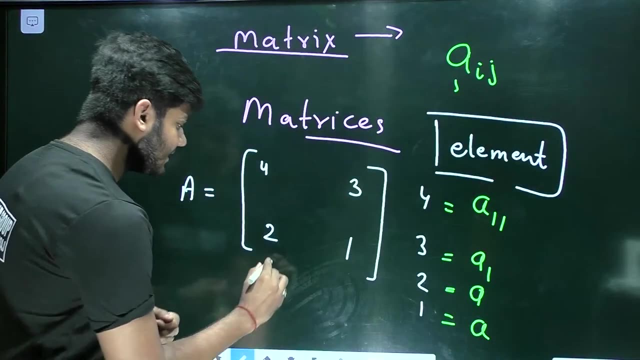 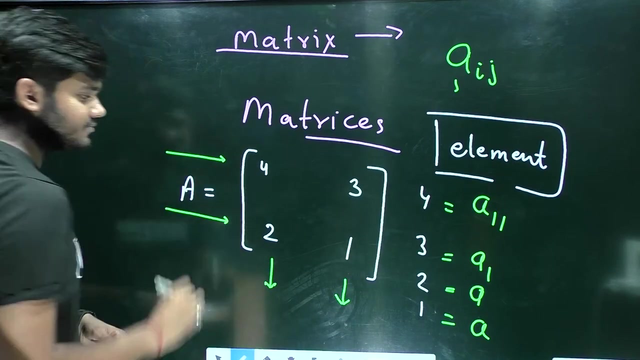 first you will write i, j. what is i in that row? sorry, in which row that element is? we are talking about 3. 3 is in first row, first row. in which column? first column, second column, first row, second row. is it clear arrangement? do you understand arrangement? 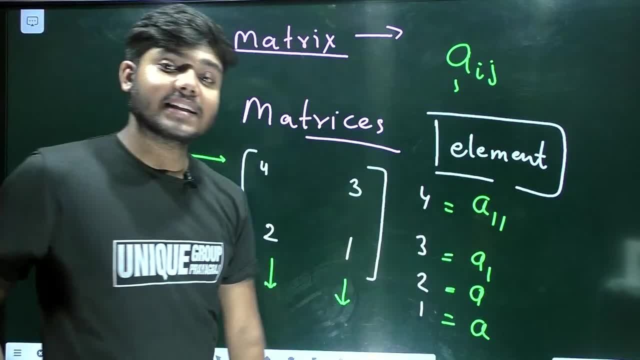 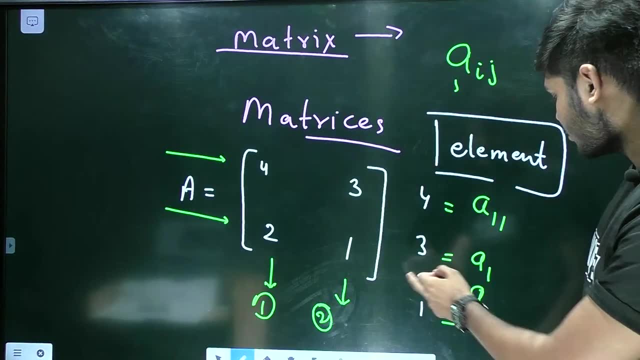 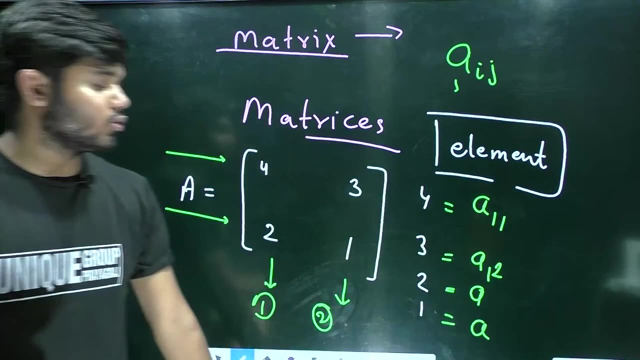 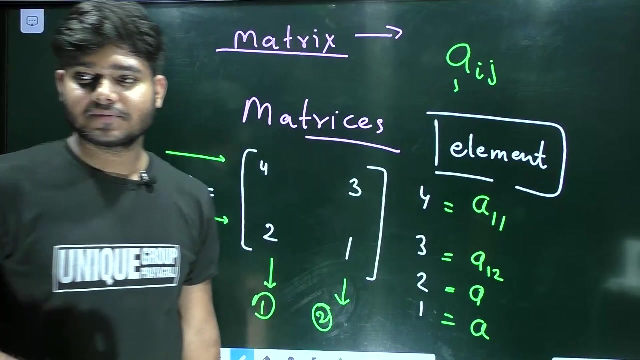 so what i said first one is in row. let's talk about column. first column is this, and second column is this: in second column we have written 2, so element 3, its value will be a12. what will happen? a12? oh, ok, when i say a12. 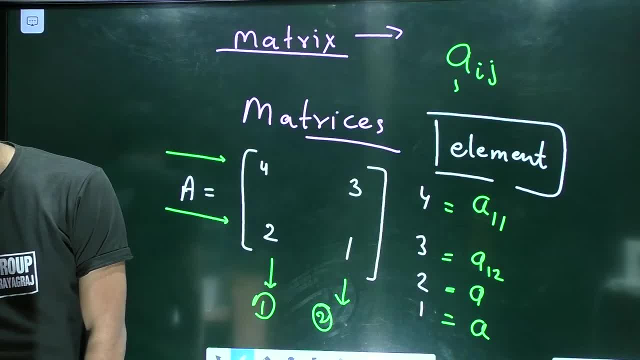 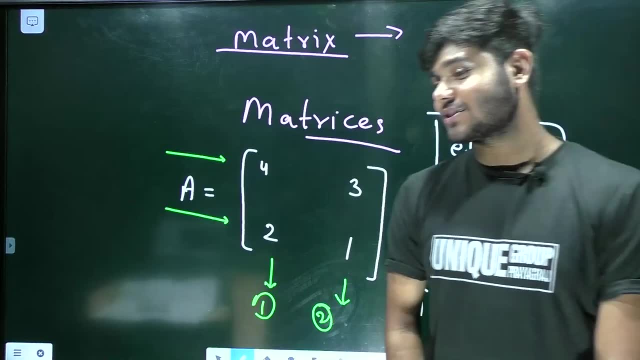 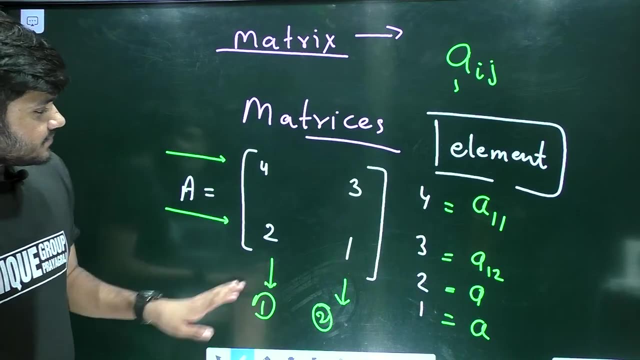 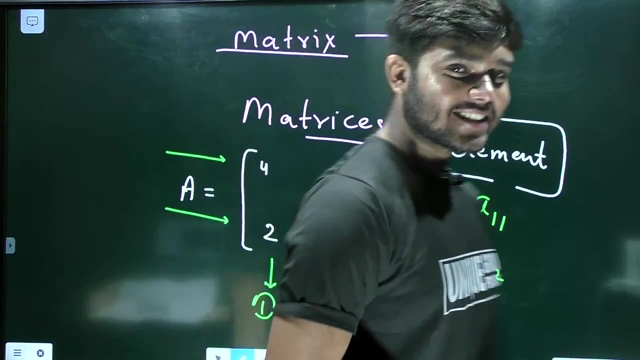 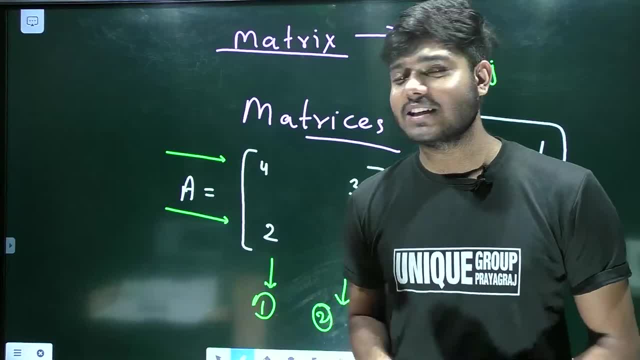 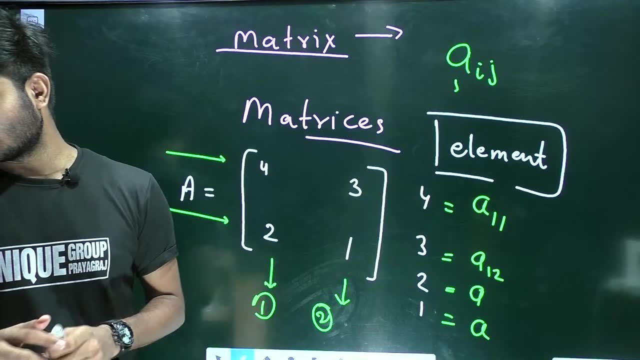 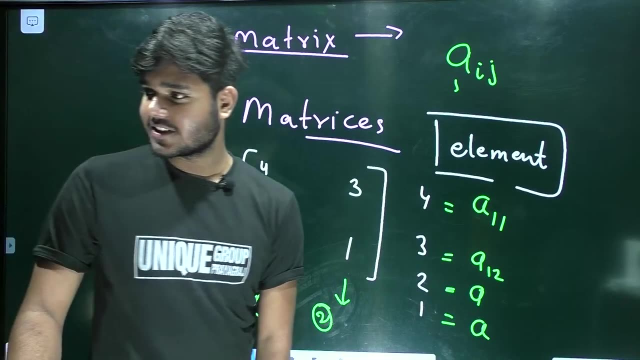 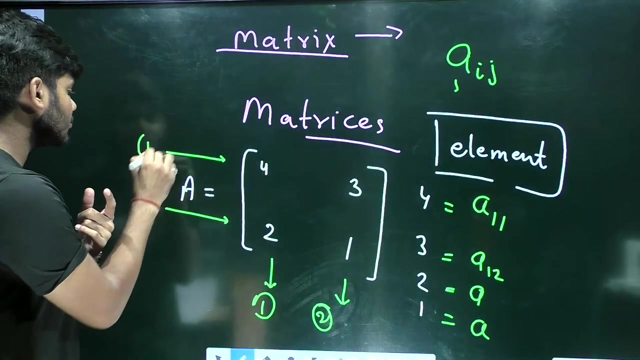 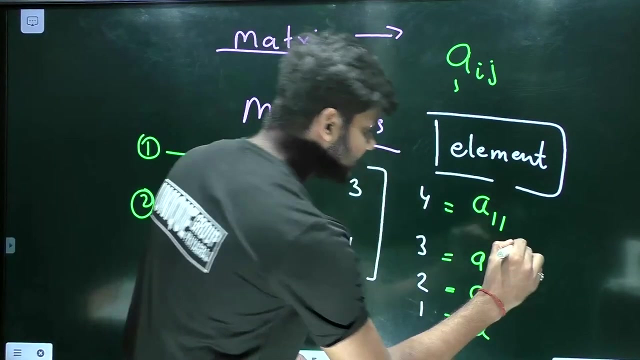 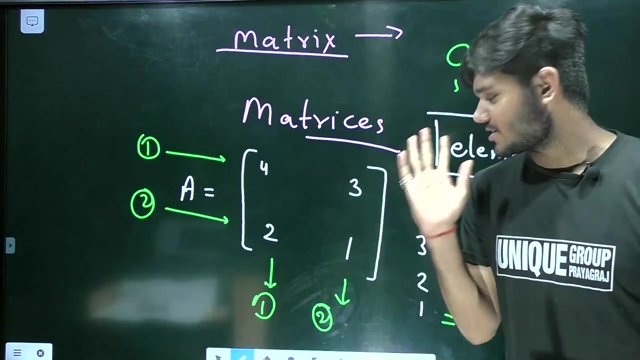 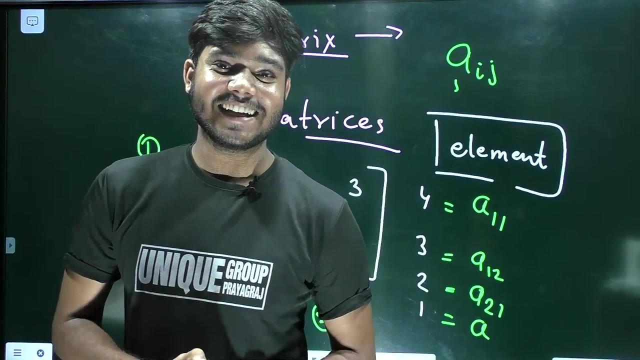 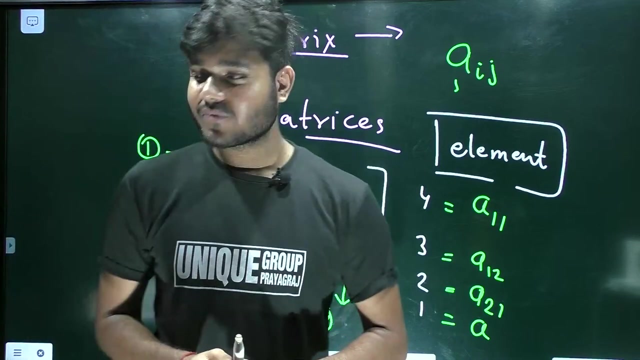 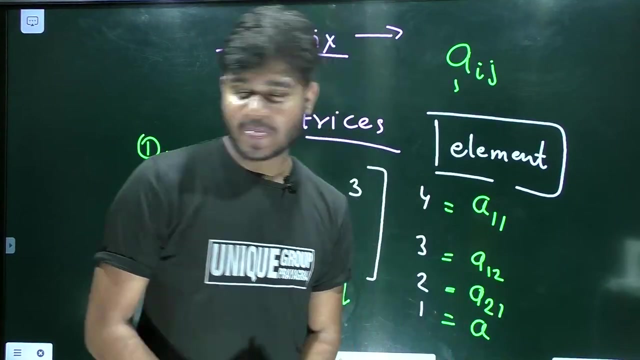 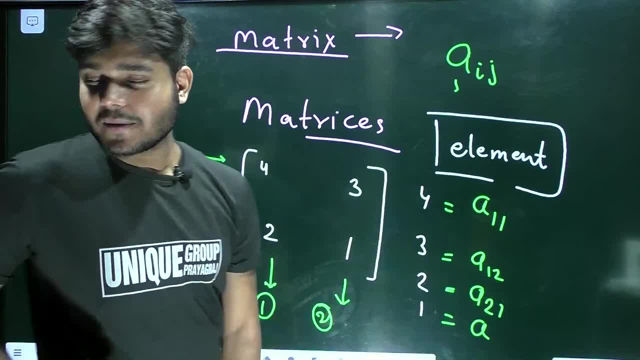 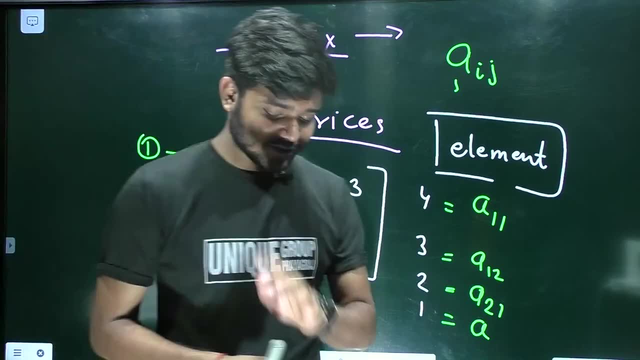 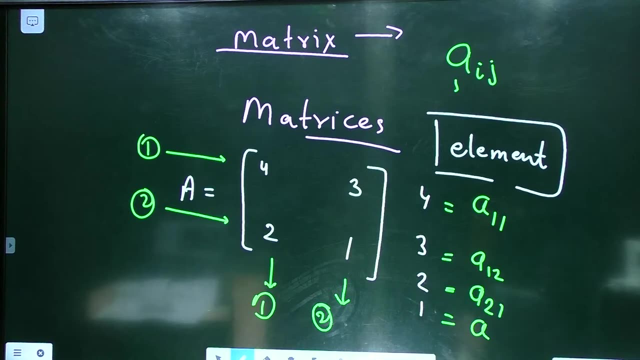 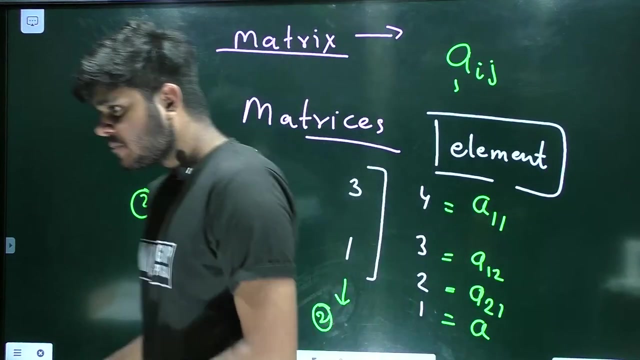 Did you understand? Then tell me what will be 1. Tell me what will be 1 1, 2, 2 equals to 1. 1, 2, 2. 2 equals to 1 1, 2, 2. 2 equals to 1. 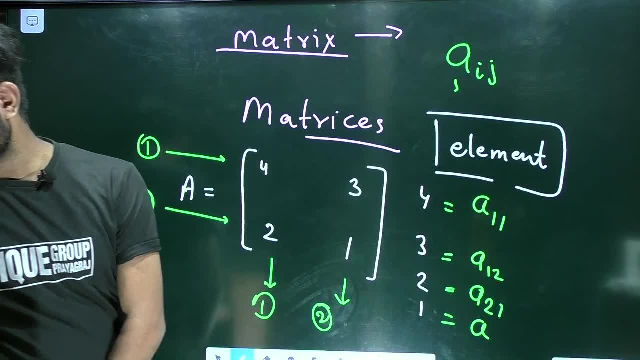 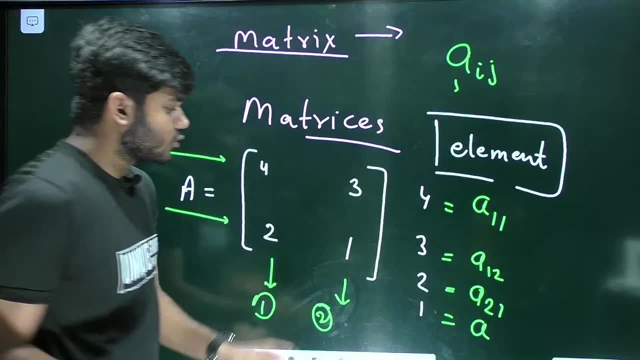 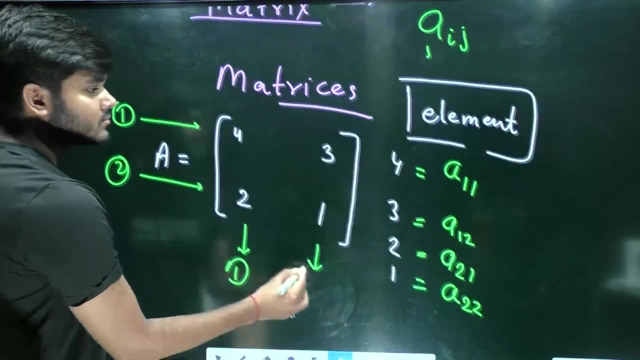 1, 2, 2, 2. Okay, Did you understand. Did you understand? There are many basic things in mathematics. So what did we say about 1? First row, then column. Which row is it in? Second row, Which column is it in? 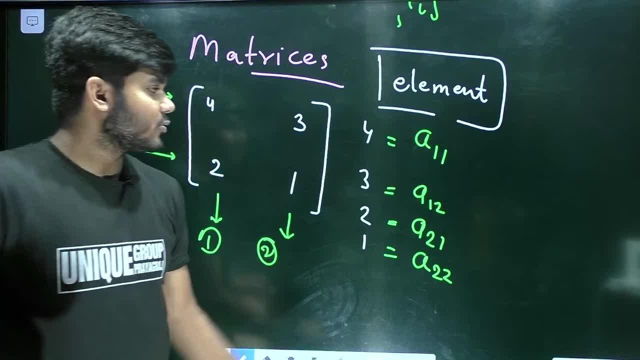 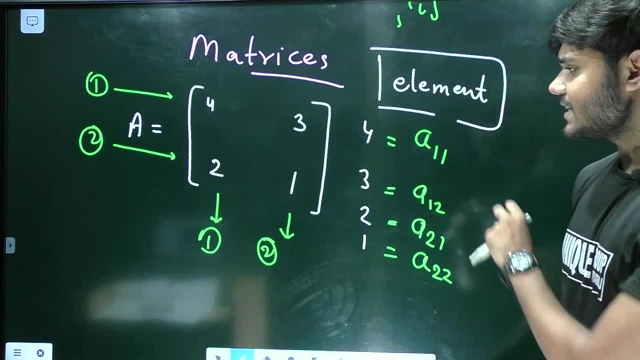 Second column is it in? So those who are in 4th class, Because it is also there in exam. So those who are in 4th class, Because it is also there in exam. It is very basic, It is very good In this. you need to keep in mind. 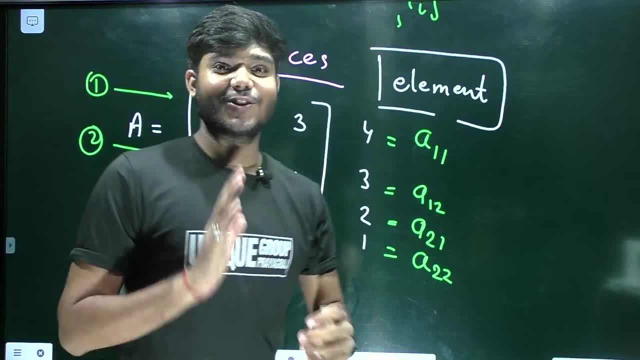 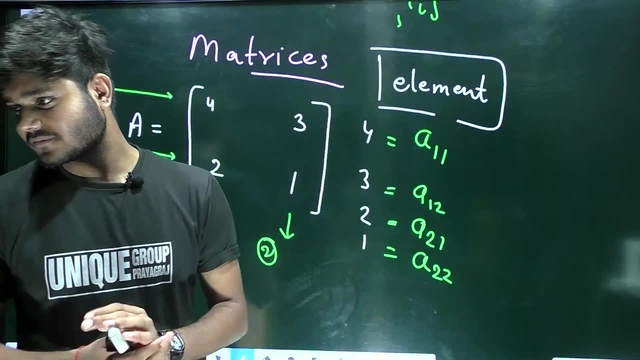 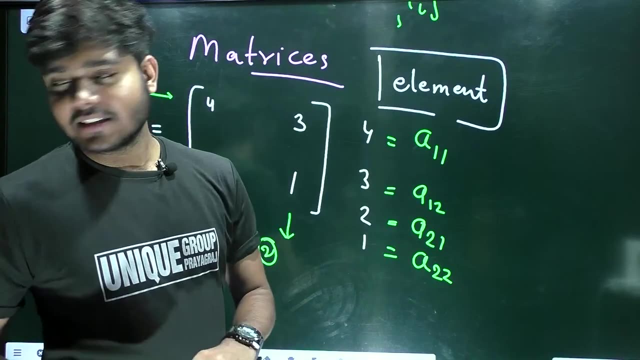 Which row means which column, Which row means which column. Now you understood. So, guys, Please like, share, And by doing so, Please share it, Call your friends and friends. Let's move on to the next part of the session. Let's take some more examples. It was very easy. 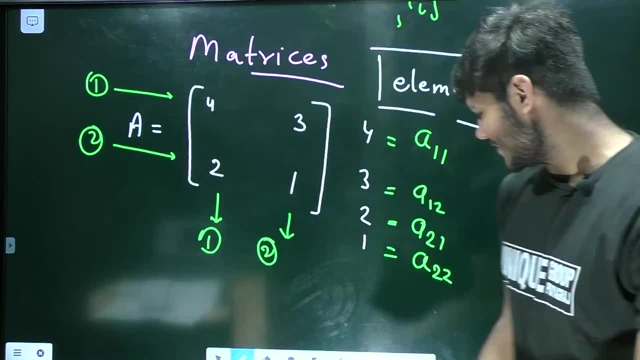 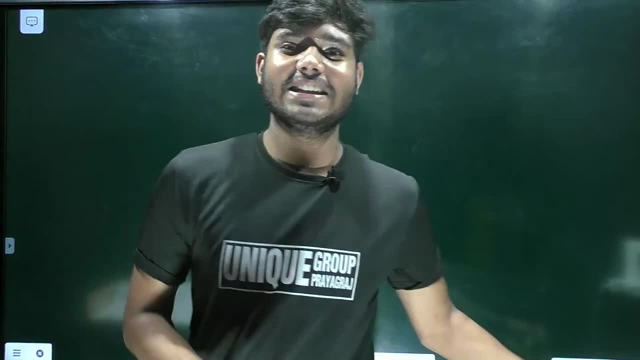 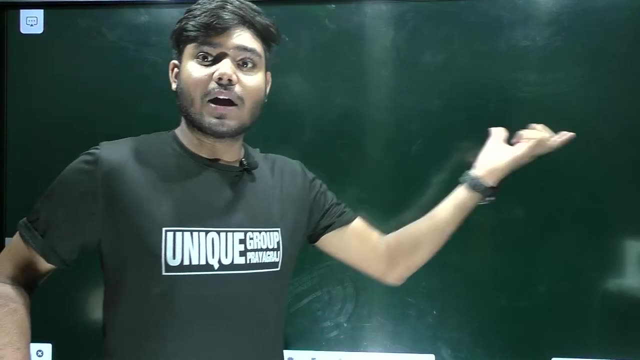 It was very easy. It's okay. This is how it should be. When there is a question in the exam, we will say: what is this question? We will solve it in our sleep. Right? These are the basic things. If you solve these basic things, 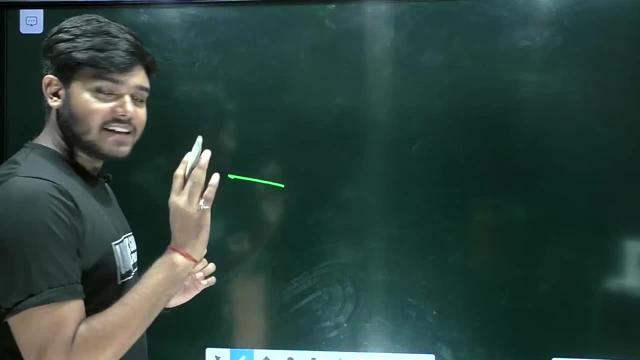 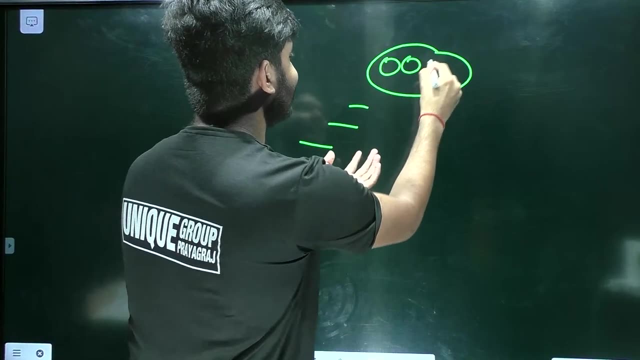 then the first step is to climb the stairs. The first step is to climb the stairs, Then the second, then the third. If you reach the roof of the house, there is a big rock And you will find a water lily. 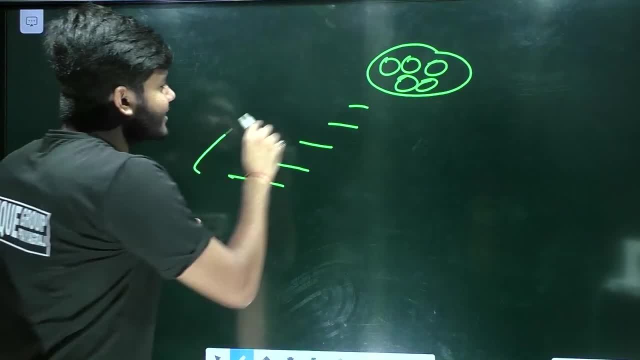 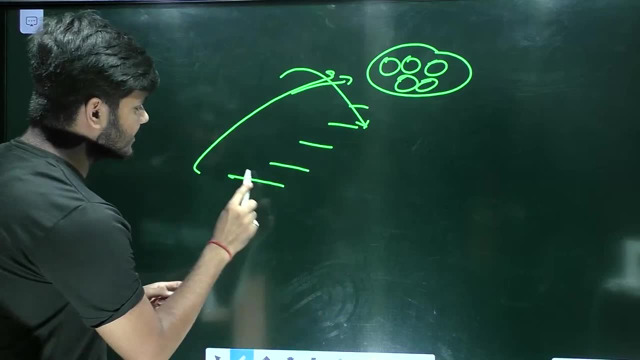 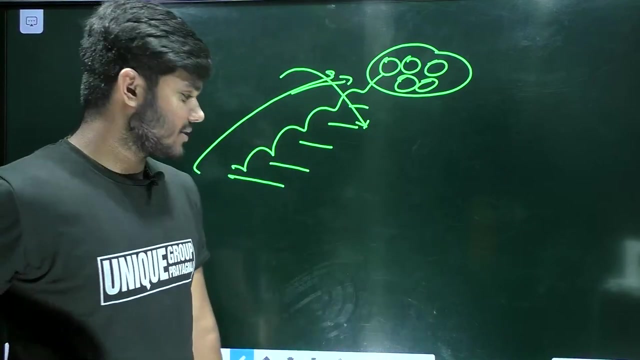 Go and check the water, lily. Anyone who tries to jump directly will fall down here. Even if he reaches these kids will reach before him, who will practice from here. Okay, The first thing is that you should not be afraid. Some kids start screaming because of fear. 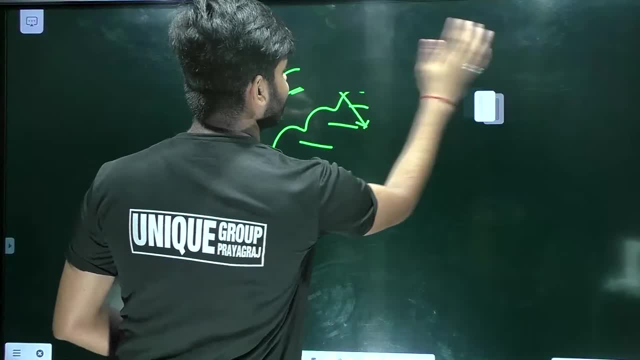 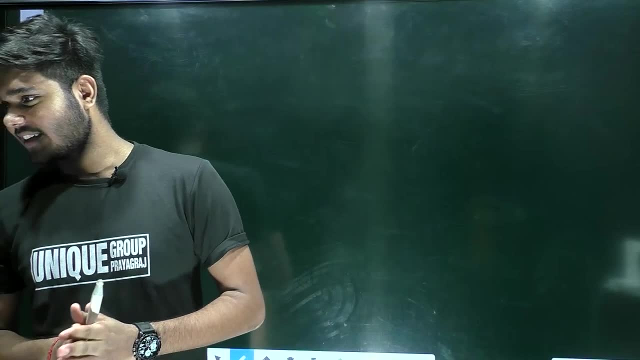 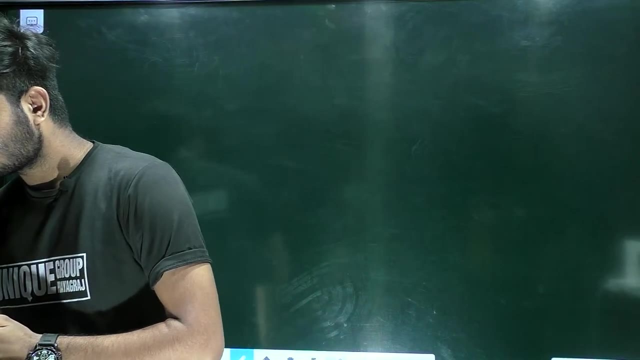 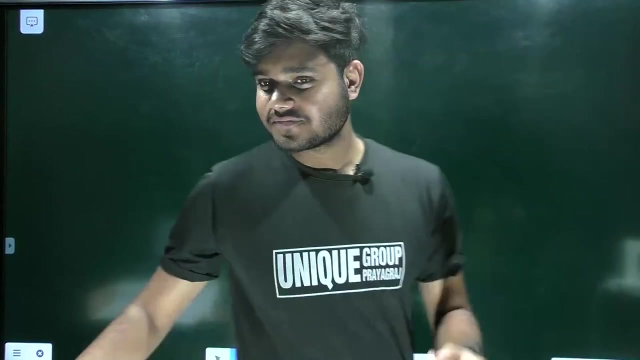 But don't be afraid of me. Why are you scared? You are subjective. You will also be solved. It will be solved easily. There is a problem? Yes, Sachin, Congratulations, Love you. Let's take the next example. You will give the answer. We will not give anything. 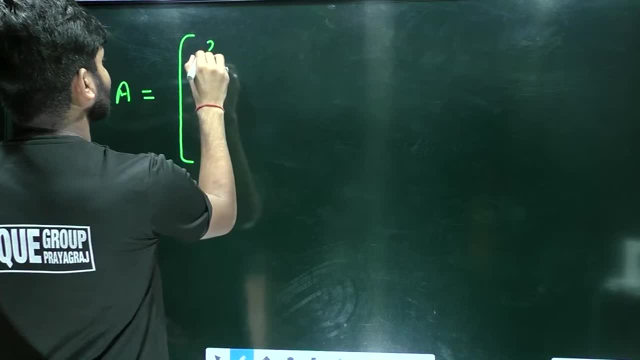 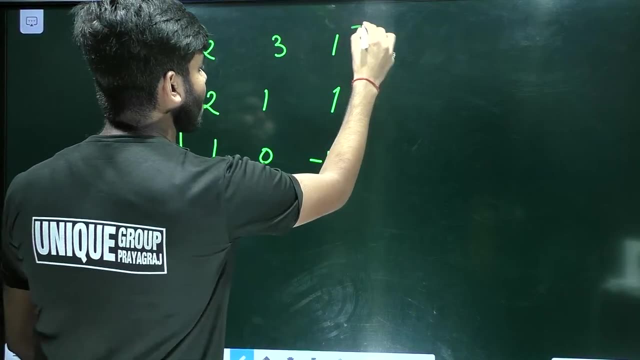 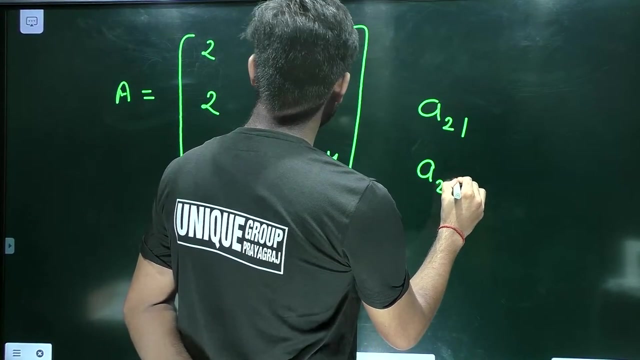 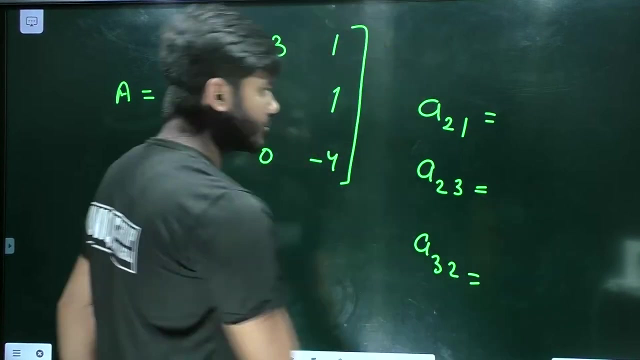 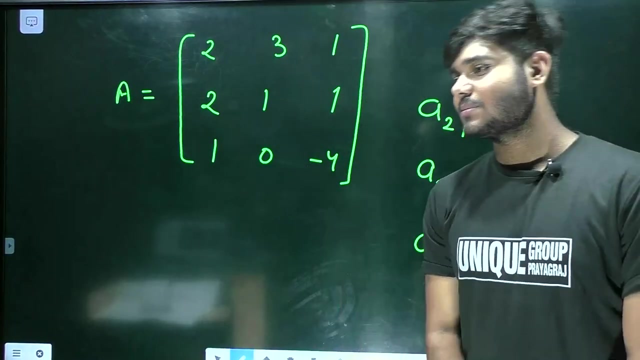 Let's see: 2, 3, 1, 2 1, 1, 0 minus 4. Tell us What is A2 1? What is A2 3? What is A2 3? Tell us, Let's see. I hope you will also be fine. 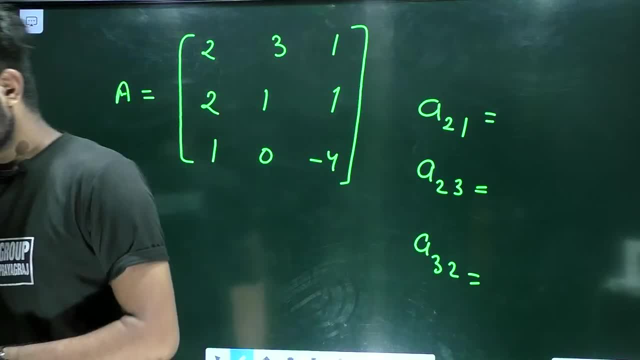 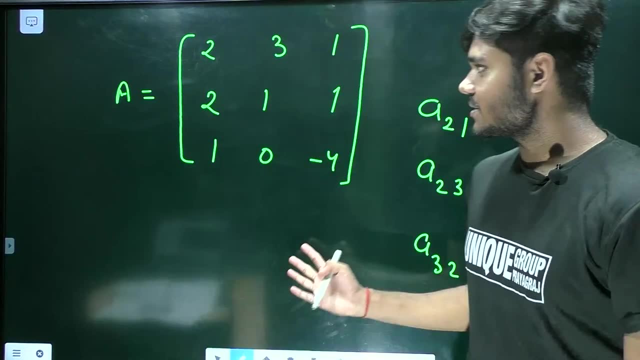 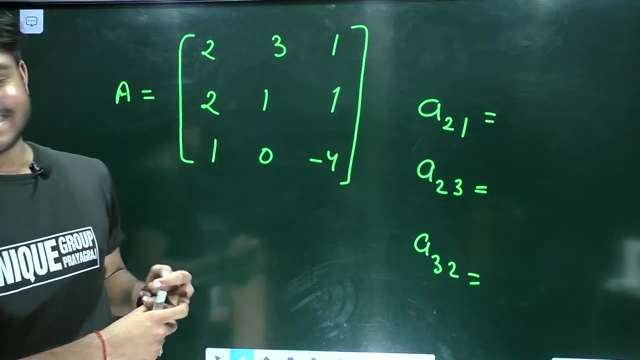 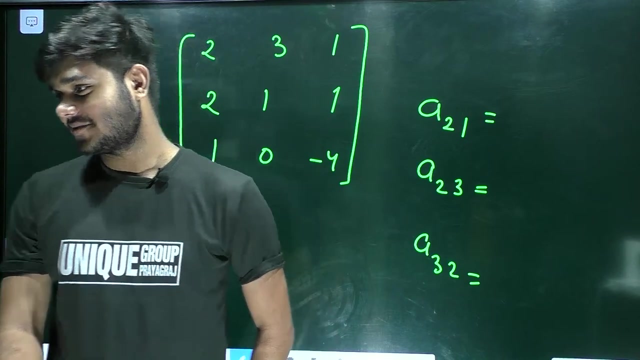 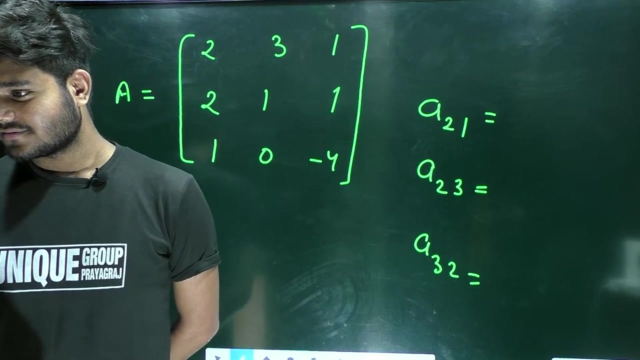 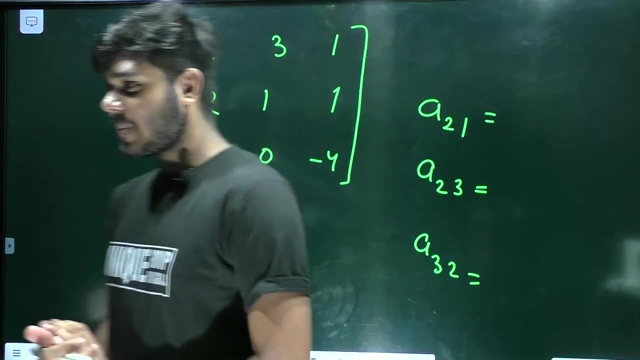 You are fine, Let's explain again. I will explain again with this example. Ok, We will revise it with this example. Don't worry, Intelligent boy, Tell us What is A2 1, What is A2 3? Tell us, Tell us quickly Calculate. You are perfect, You are excellent. 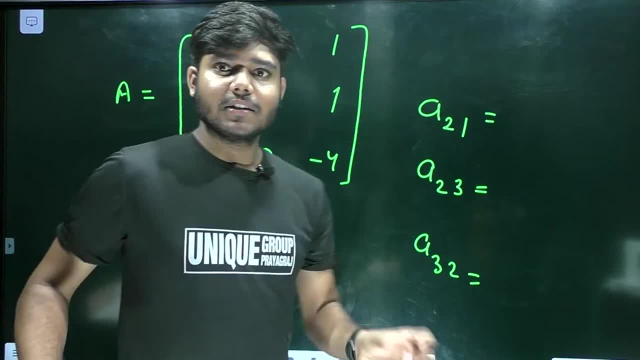 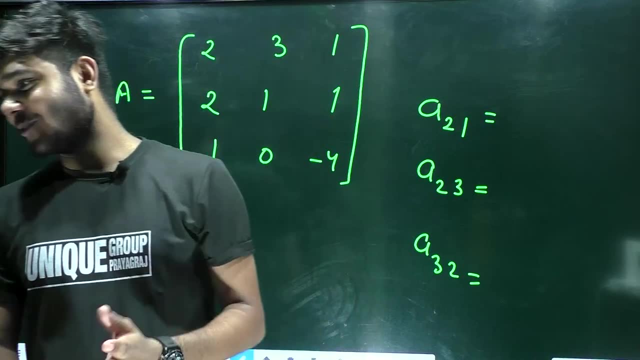 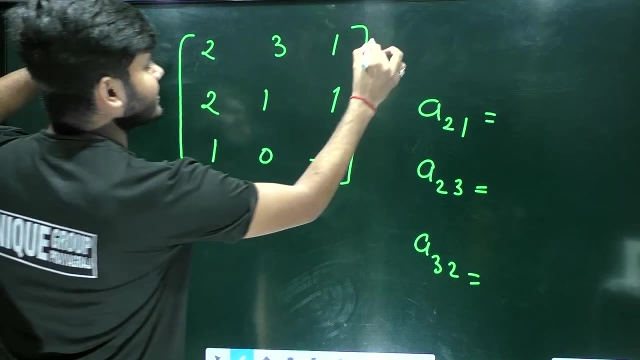 You are a heavy. What is A? You are a heavy driver. you are a heavy driver. What is A2 3? You are a heavy driver. Oh, you are a heavy driver. Let's see what are the columns. Let's see what are the rows. Horizontal 1st row. 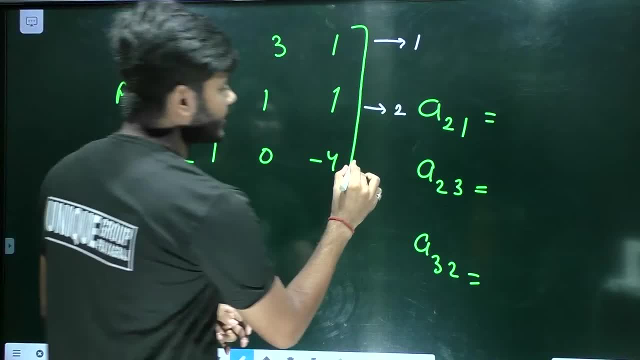 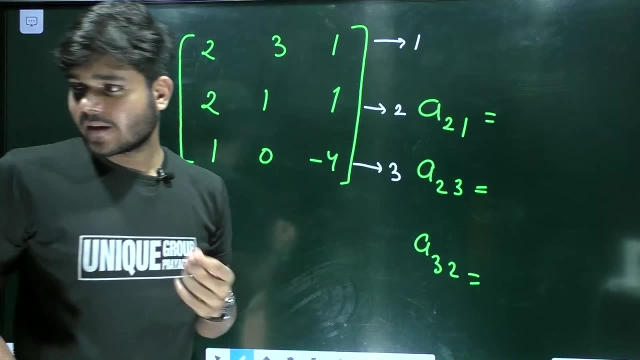 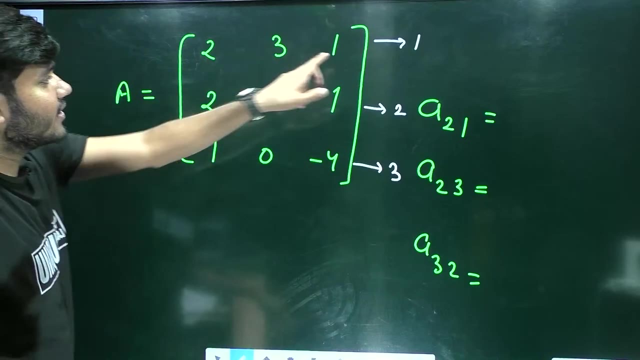 2nd horizontal, 3rd horizontal. 3rd row: How many rows do we have? How many rows do we have? We have 3 rows. Those who don't understand, we will explain later. So what did we say? How many rows do we have? 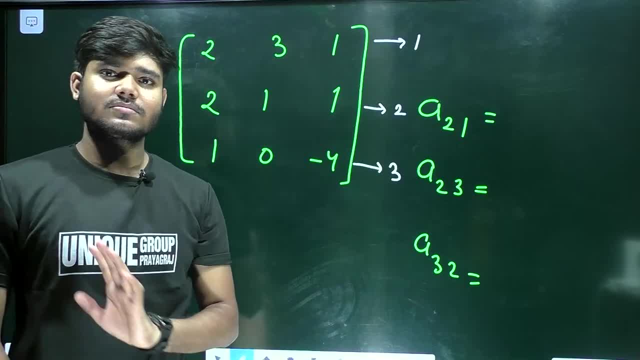 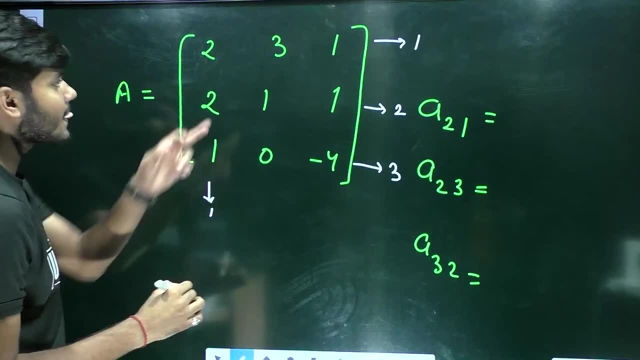 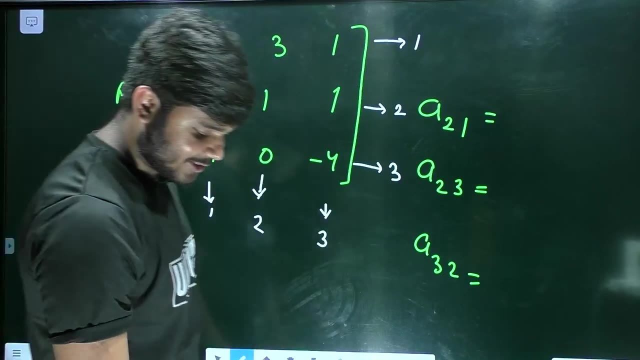 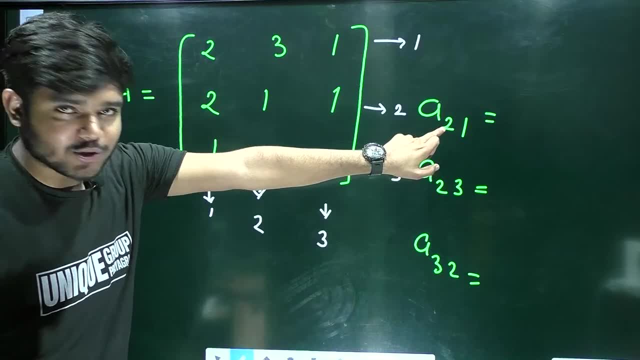 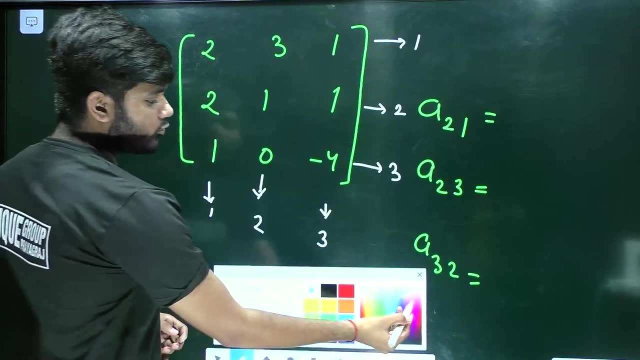 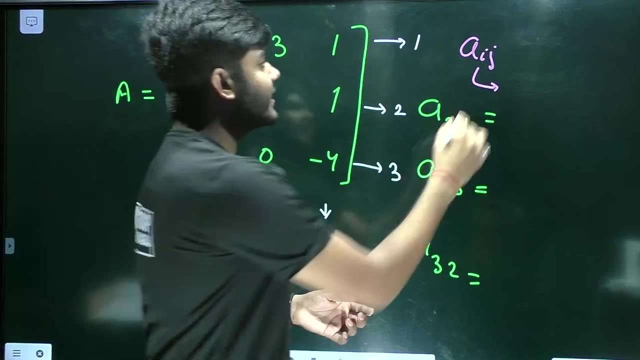 So now you can tell What does 2 mean? The element is in 2nd row. I told you Aij A is written in the form of ij. A is written in the form of ij, Where i is in row And j is in column. Do you understand? 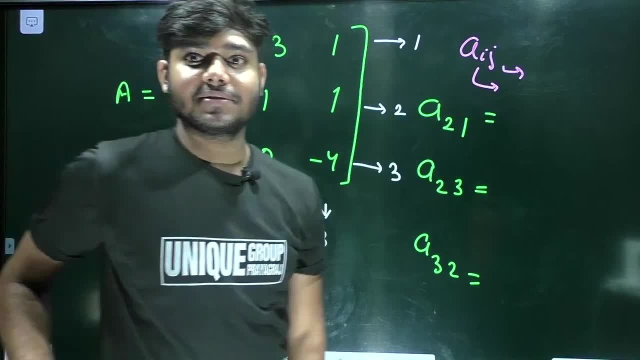 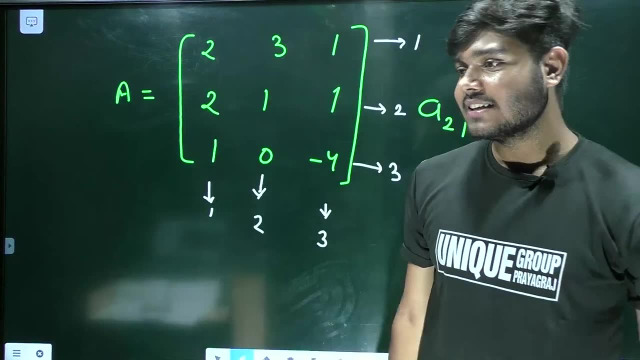 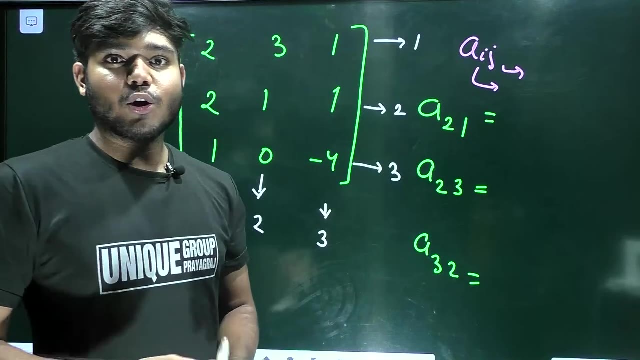 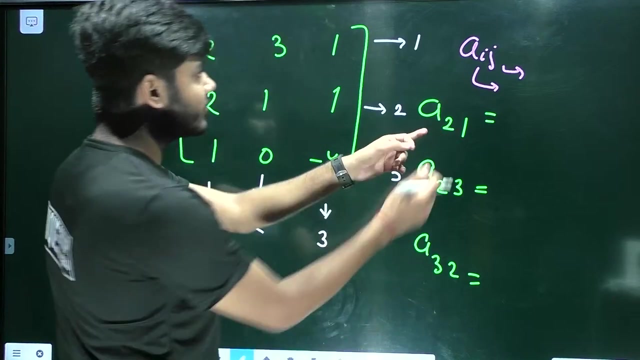 So now see What is a21?? What is a21 element? So now what will you say? Square matrix? Very good, We will come to types, We will tell about types And will ask you. So we will come to types, No problem. Let's see What is 2?. 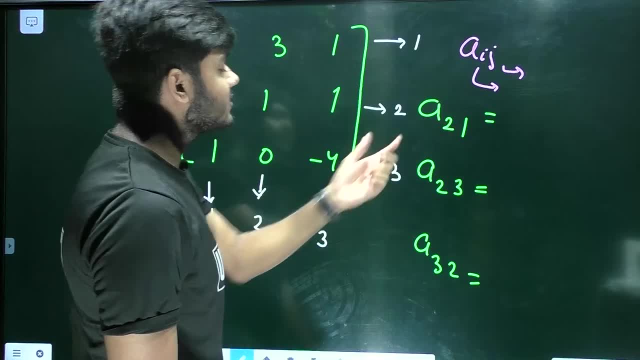 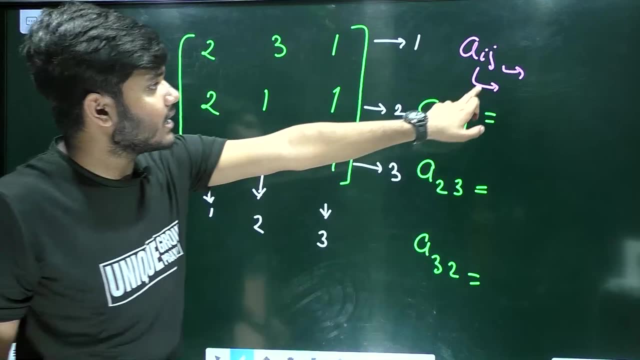 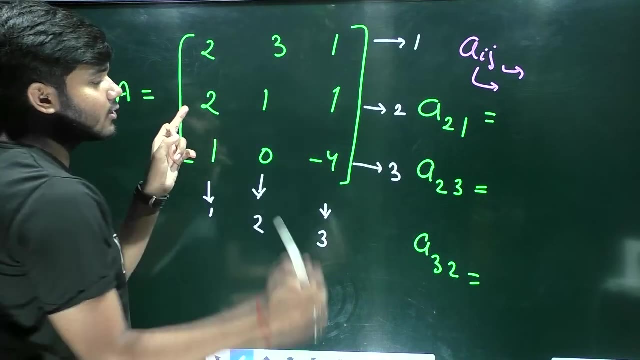 Number of rows. What is 2?? It is row Where you saw 2. It is in 2nd row. Column is in 1st row. What does i tell us Row? What does j tell us It is row? OMG, If we see, It is 1st row. 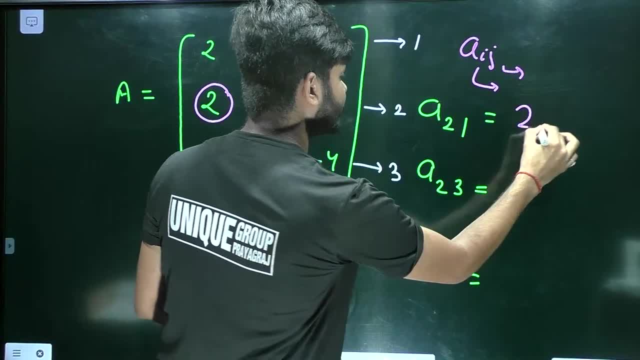 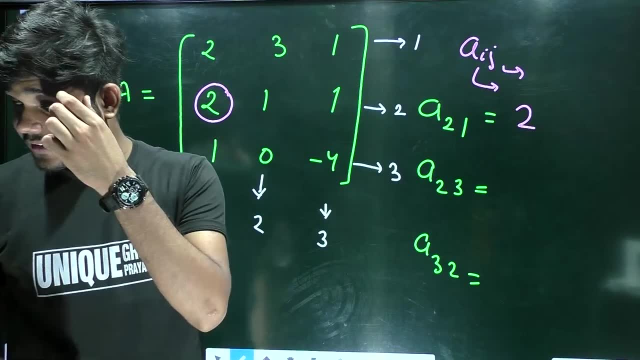 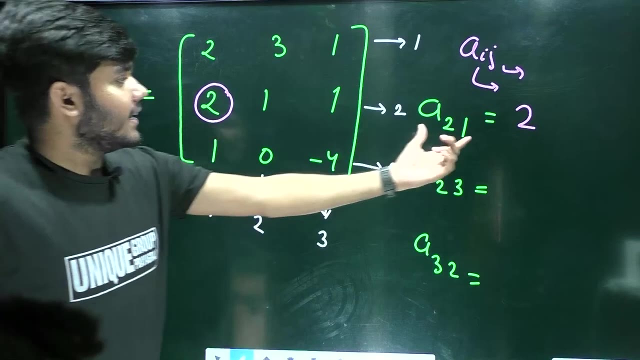 Column 2 Row: Ok, So if you see A 21, That means 3 row, N3, 3, 2, 3 1 2 1 1 1 1 1 1 3. 1 1 1 1. 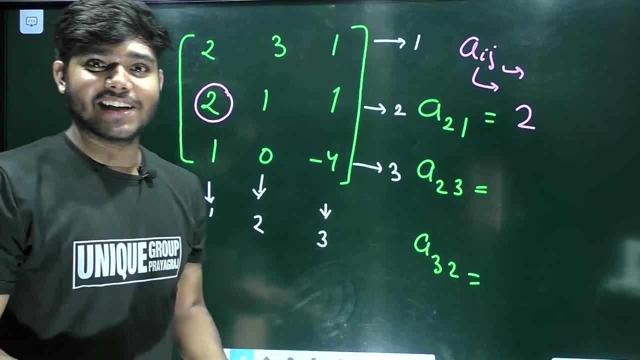 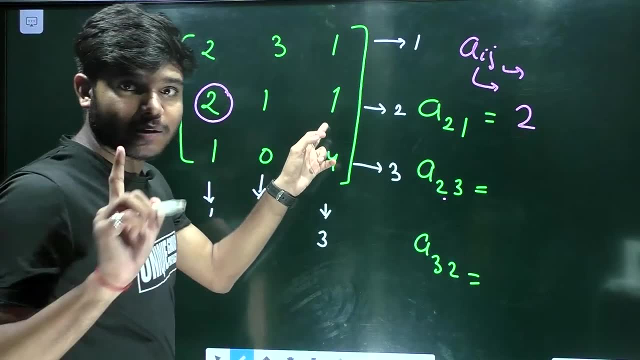 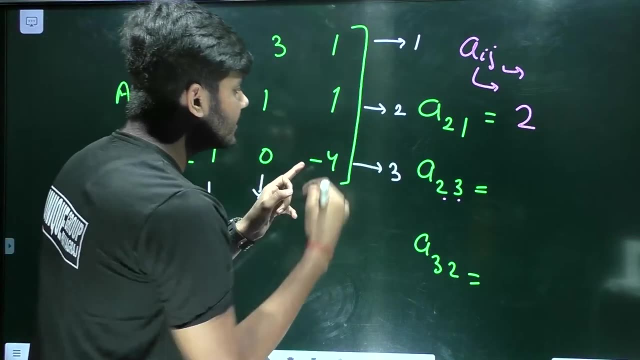 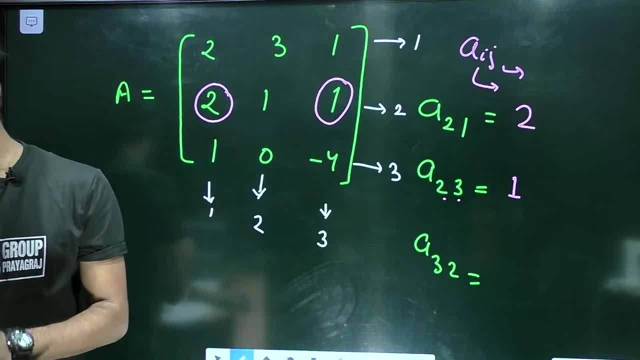 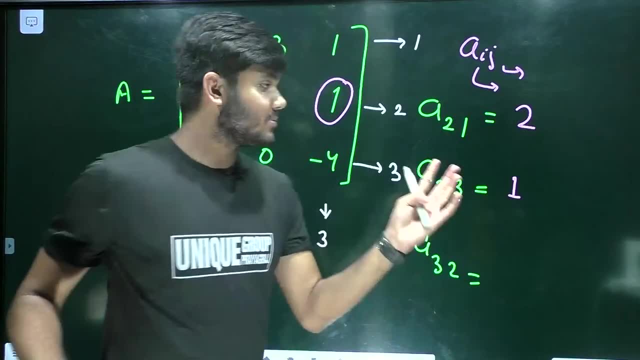 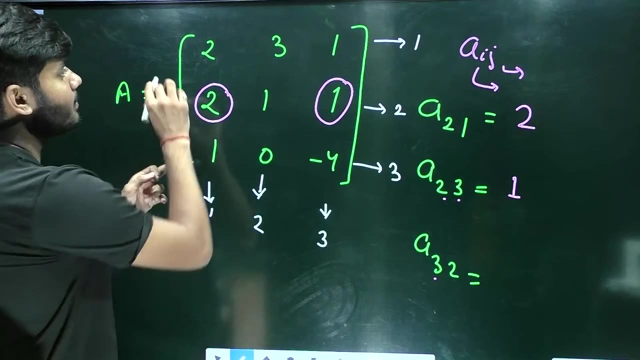 What is the element 1? Now it is getting clear Slowly. Now it is getting clear, We will give questions for homework. What is A32?? 3 means 3rd row. 1st, 2nd, 3rd. Now in 3rd row. 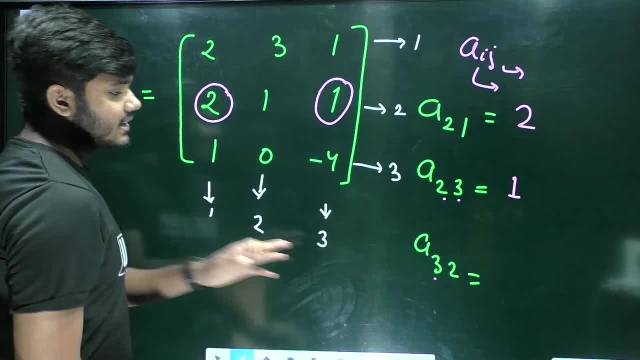 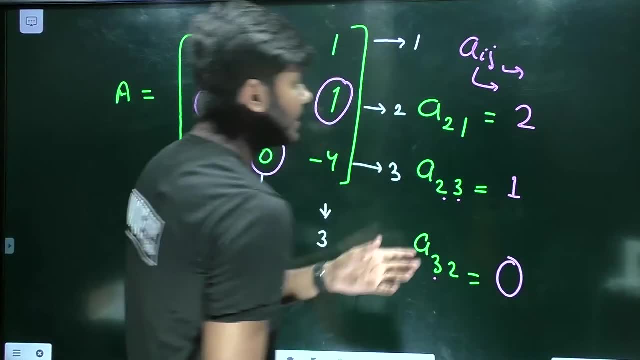 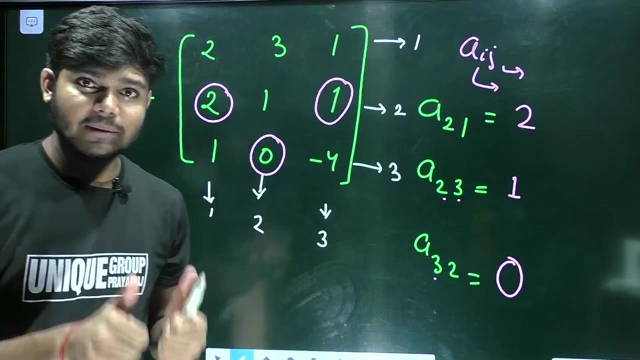 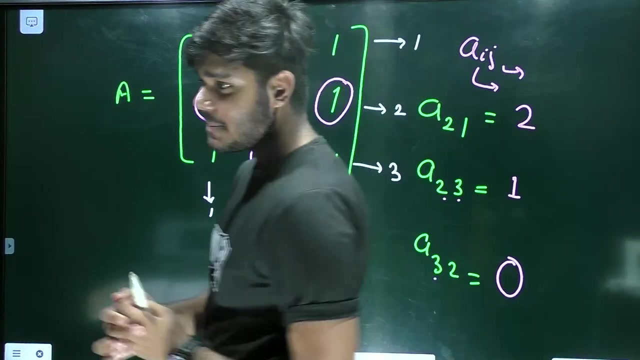 Go to 2nd column, Go to 2nd column, 1st column, 2nd column, And this is our answer And this is our particular element. If you understood Show thumb, If you understand Like, Because we understood Like And you are no more sharing, No problem. 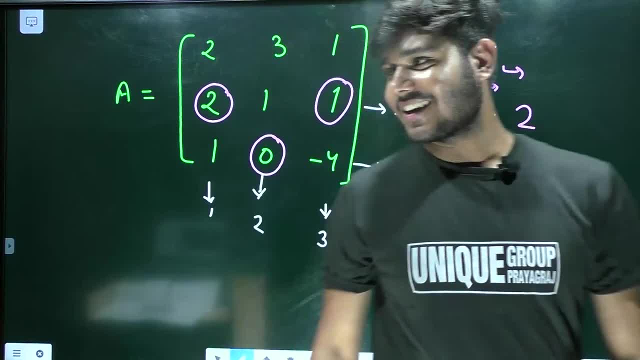 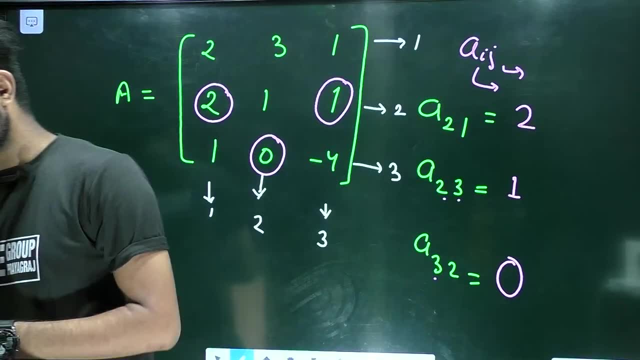 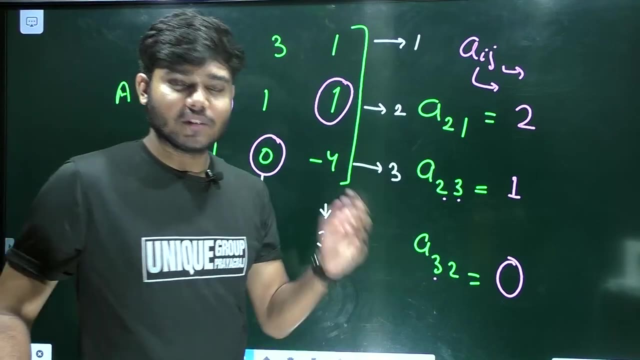 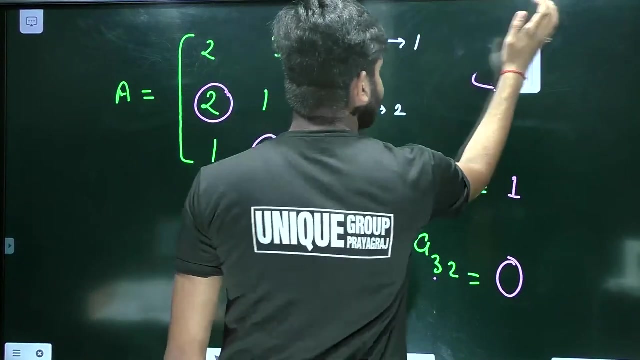 If you like, Then do like. If you don't, Then tell everyone That Sir didn't like this. We will tell you this. So we have, for A31, A2 to A32, Understand. Do you know how to identify an element? If you know how to identify an element, then we are just giving you one more to see who will be the first to tell you. 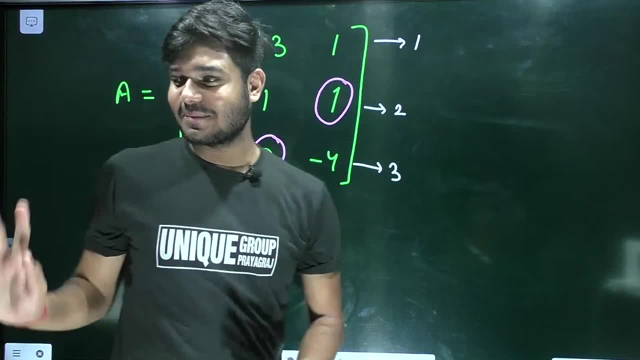 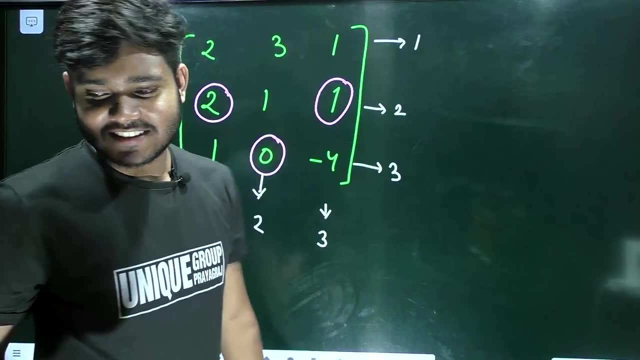 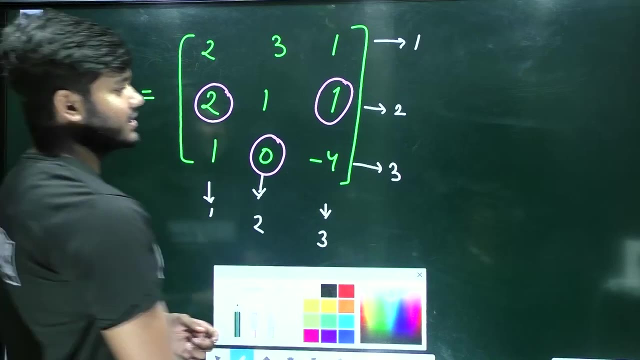 The one who will tell you first will be given a reward. For now it will be given online, But when you get it offline you can take yours. Okay, So let's see who will tell us first. First of all, tell us what is the element of A3-1.. 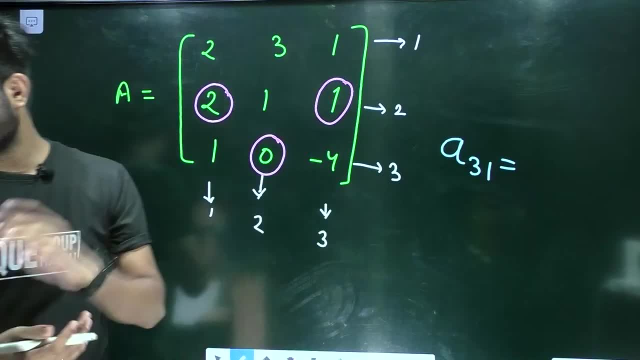 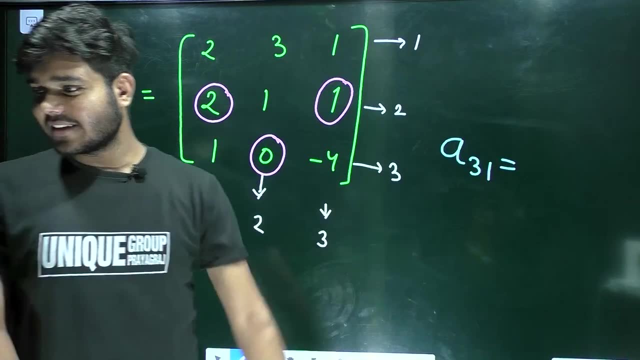 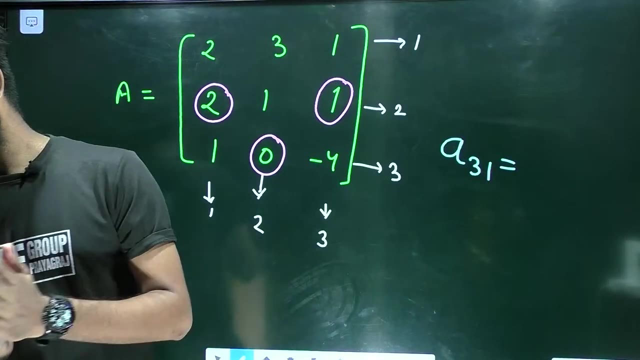 Come on quickly. A3-1,. quickly, Very good, Thank you, Jai Shankar ji. Come on quickly. A3-1.. Let's see who will tell us first. Wow, Why are there two? Someone is saying A1,, someone is saying A2.. 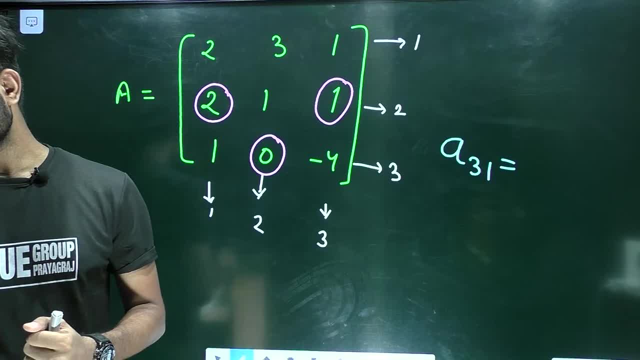 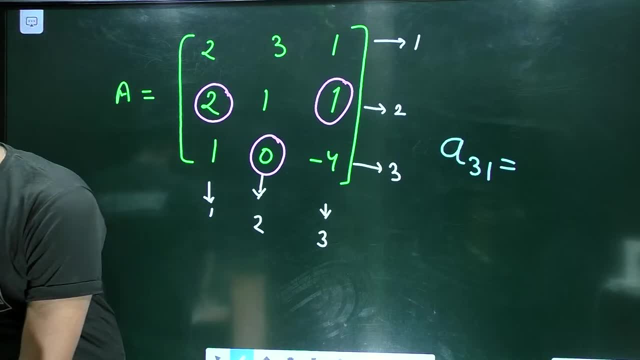 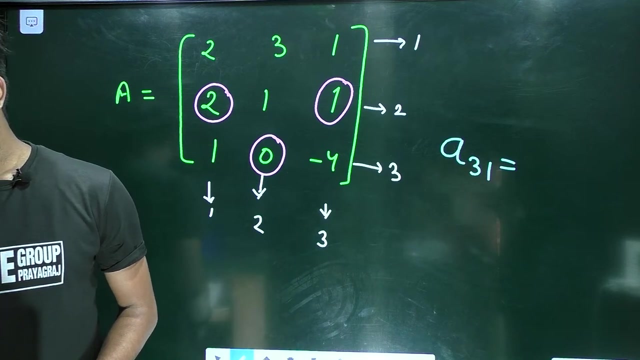 Is there any confusion? It seems to be A1.. There is a confusion. A2 is a three-dimensional element. It depends on the number of elements. A2 is a three-dimensional element. A2 is a three-dimensional element. It depends on the number of elements. 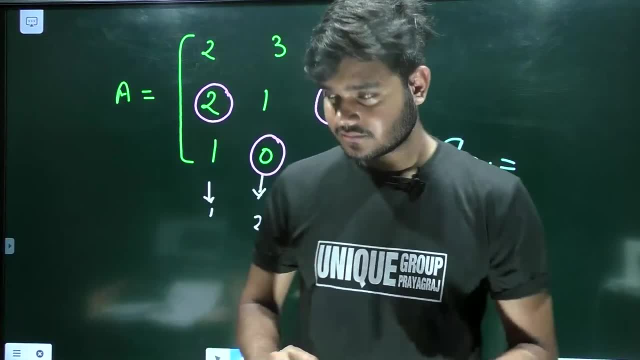 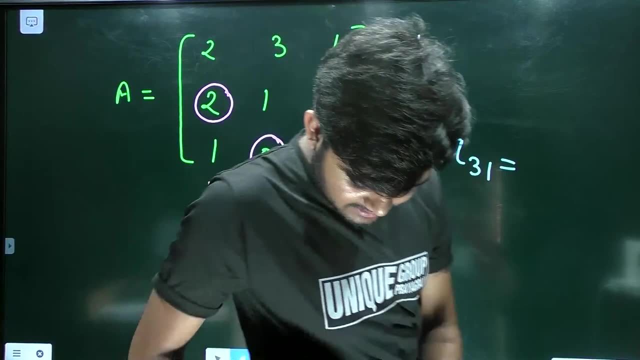 It depends on the number of elements: A2, A3,, A2, A3.. Did you understand, Can't you see? Can you understand? If you understood the demo class or the first day of the class, then it depends on you. 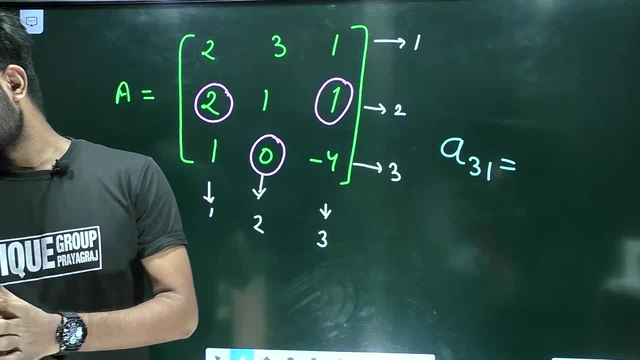 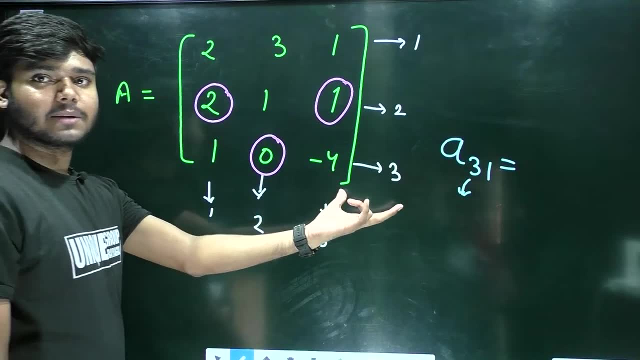 Okay, Let's see the answer. 1 and 2 are the answers. What is the meaning of 3 and 1?? What is the meaning of 3?? What is the meaning of 3?? You go directly to the third row. 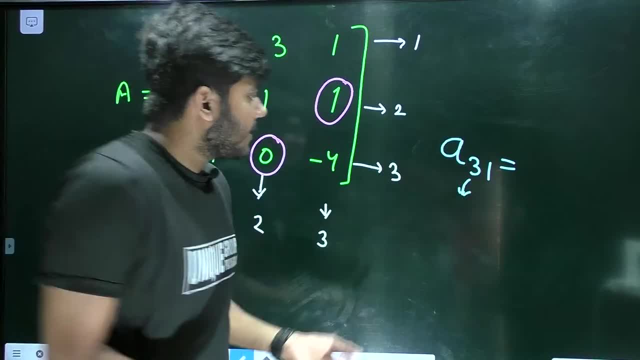 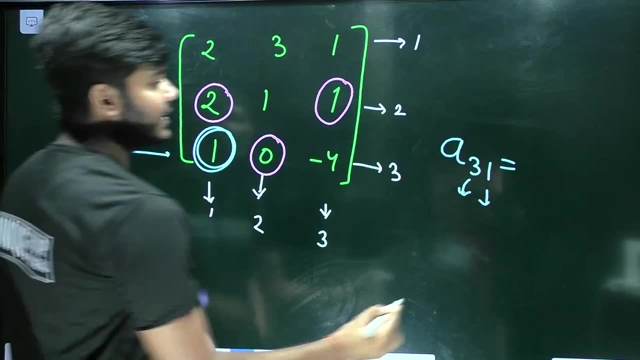 This is the third row. Row number is third. Now see what is written here. What is 1?? What is 1?? The first column, That is the value of A31, will be 1.. That is the value of the element. A31 will be 1.. 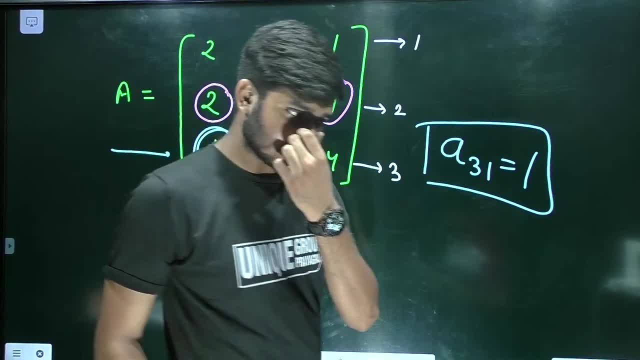 That is, the value of the element A31 will be 1.. Very good, you guys are doing very well. Very good, you guys are doing very well. Very good, you guys are doing very well. You got it right. 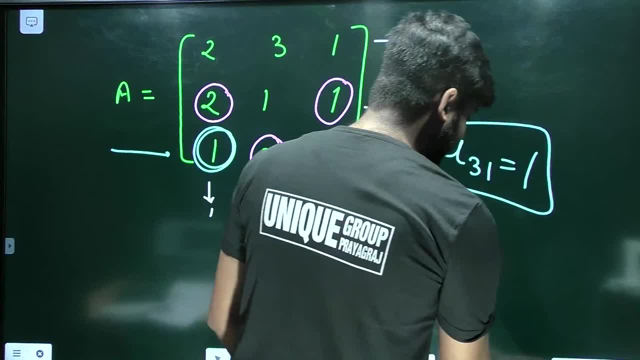 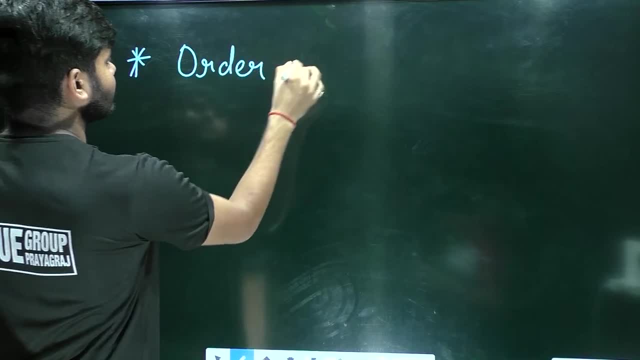 You got it right. So, now that you have understood, I am telling you the last topic, Very good and very easy. We call this order of matrix, We call this order of matrix. We call this order of matrix Very good. 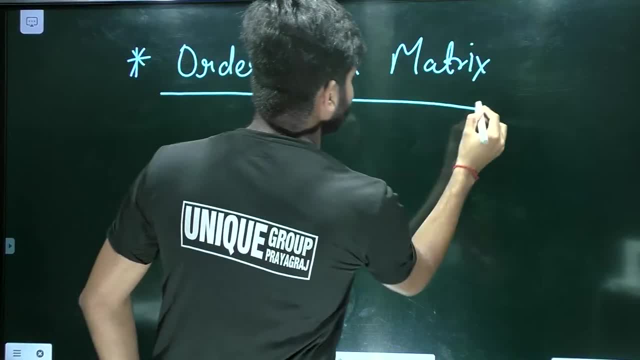 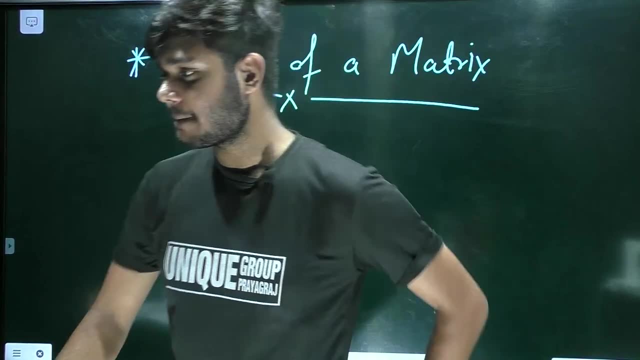 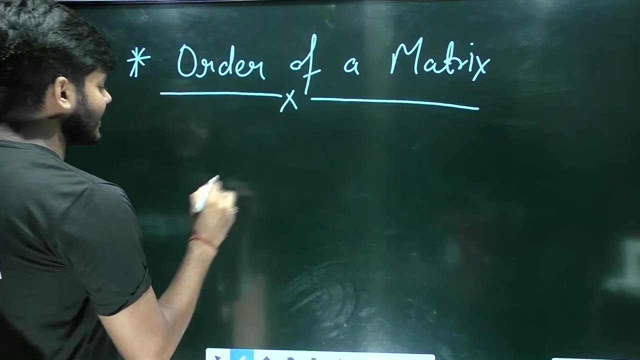 Very good, Very good To understand this. you just need to know how many rows and columns are there in our particular matrix. Okay, Let's go Look. what do we need to see the order? First of all, we need to know how many rows and columns are there in it. 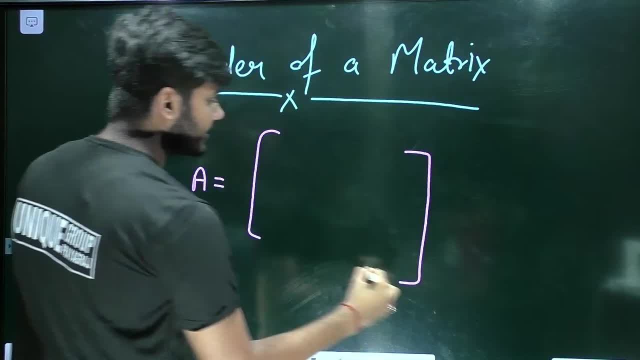 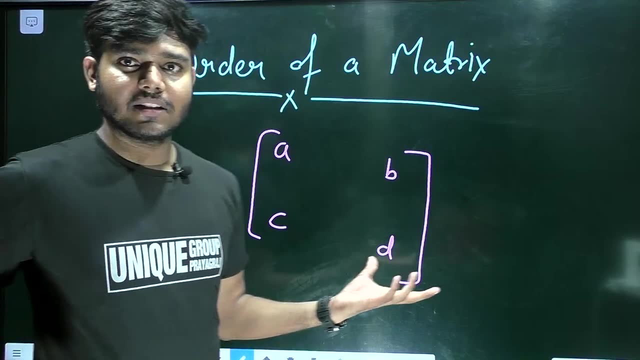 Okay, So suppose we have taken a matrix. Which one? a, b, c, d? What have we taken? We have taken a matrix. Keep in mind that in a matrix your numbers can also come: 1,, 2,, 3,, 4, any number of any type can come. 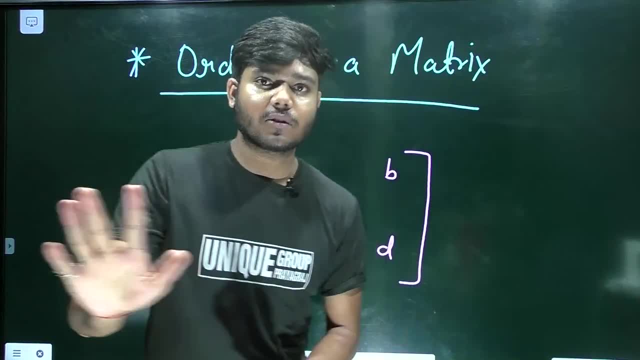 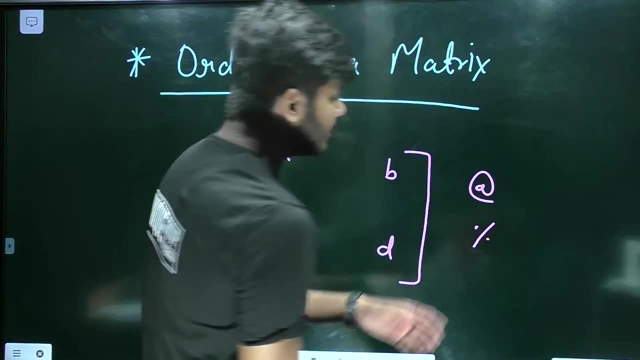 In a matrix, any element- a, b, c, d, e, f, g, h, any coefficient can come. Okay, And along with that, if you want, any symbol can come, For example ad rate, percentage dollar, anything. 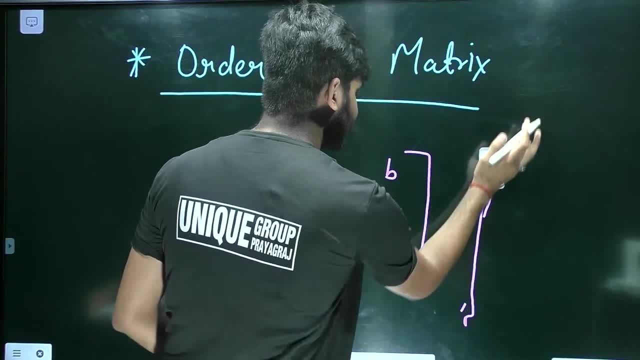 Okay, So all these things can also come. So you don't have to look like this: that sir a b c d came here. Okay, You don't have to look like this: that sir a b c d came here. 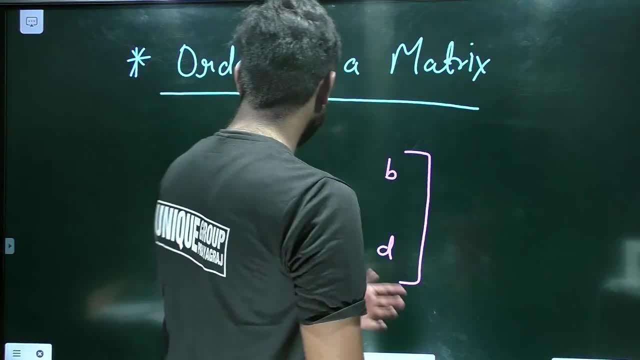 Okay, Okay, okay. everyone will get it. Everyone will get it. See here. Then what did I say? to know the order of matrix Basically, first of all, you should know that: how many rows are there and how many columns are there. 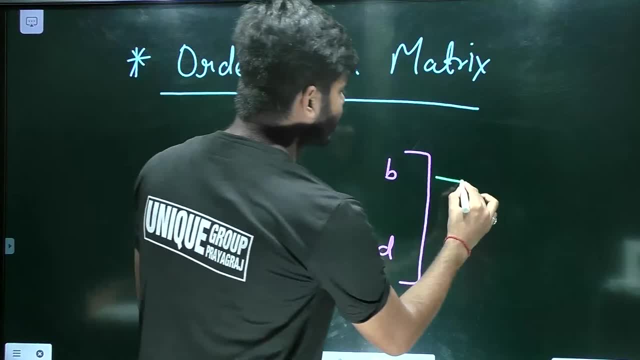 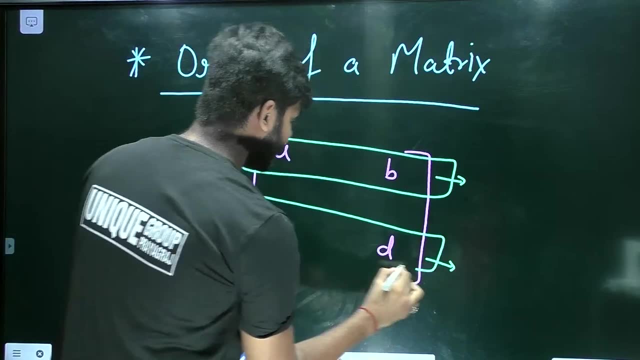 Okay, So how many rows are there in this particular? So how many rows are there? 1, 2.. See horizontal, Whatever is horizontal. This is the first horizontal. the second is horizontal. So the horizontal is 1 and 2.. 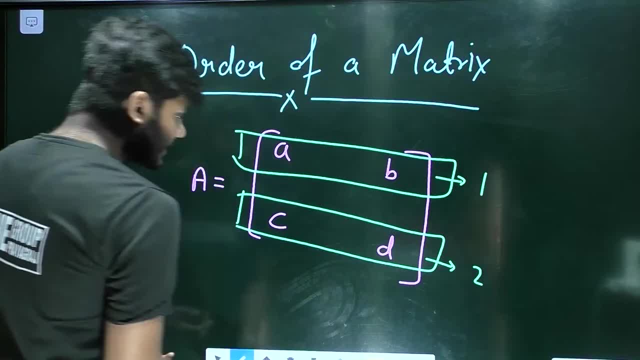 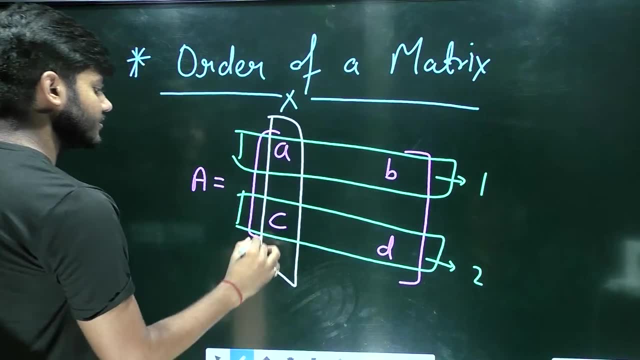 What is this? Your number of rows? Okay, And along with that you will also find out the column. Okay, So what will you see in the column? This column is yours, So 1 is 1-column and this big one is 2nd column. 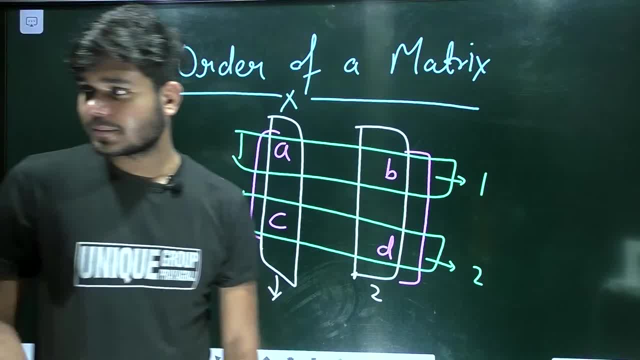 1st column and 2nd column. You have any doubt? speak up, Say, say, say, Make it fast. What is the doubt? We will put you into doubt now. Speak fast. if you don't want to, then just speak in between. 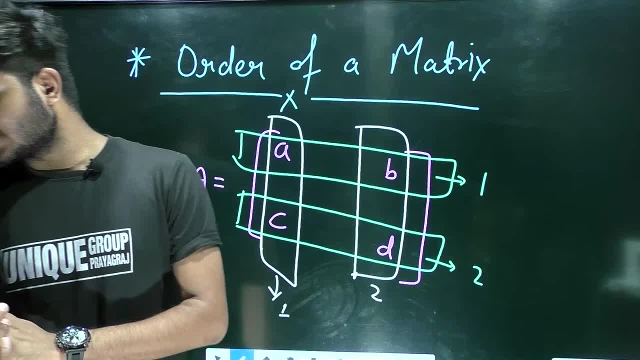 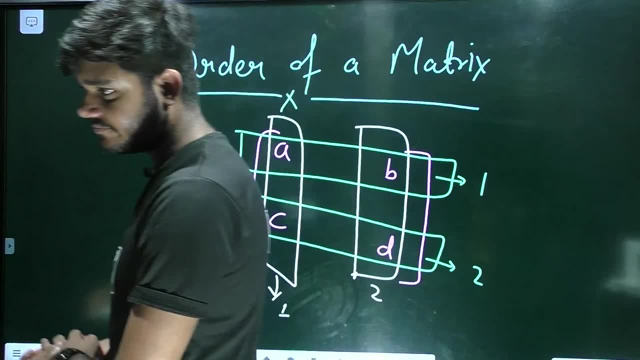 Let's move it a little further. Speak fast. Speak fast In the middle. If you have any doubt, speak fast. Please tell us. Yes, you will have daily classes, Daily classes. No, it is not much different. It is not much different from the mathematics of BCA and VTech. 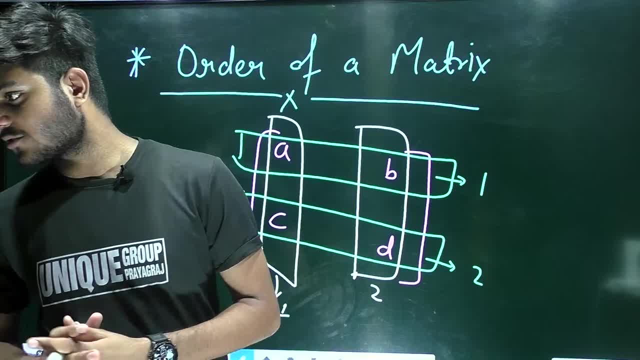 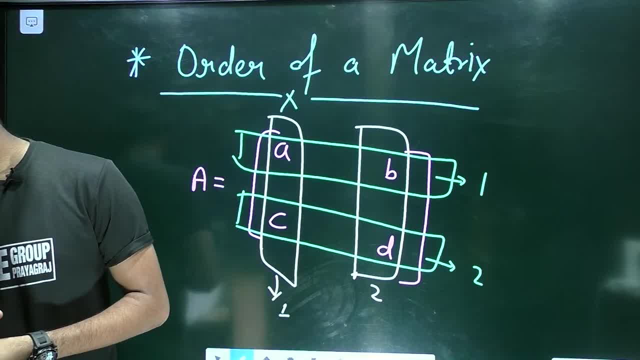 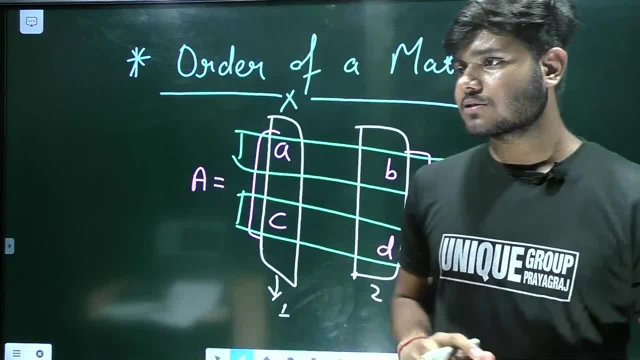 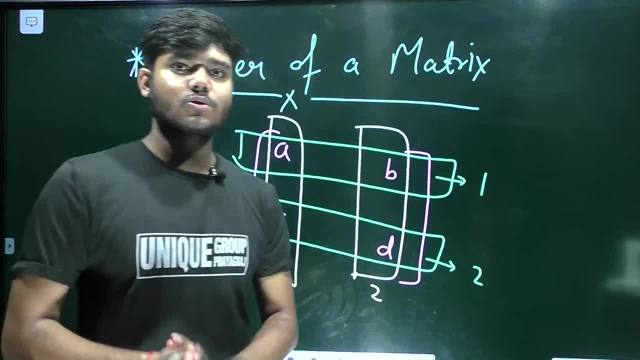 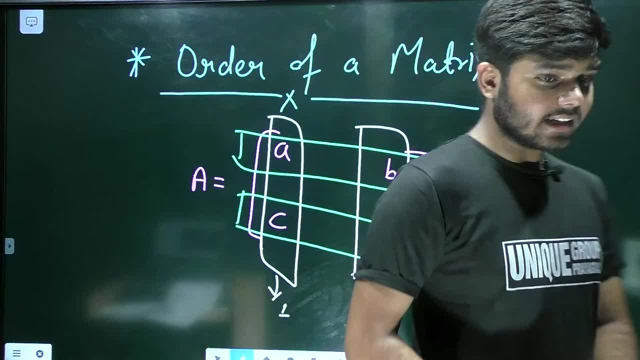 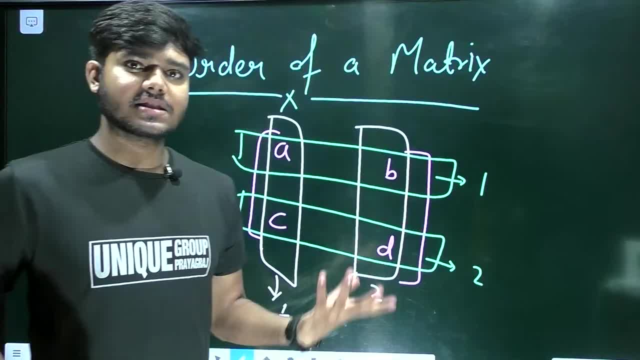 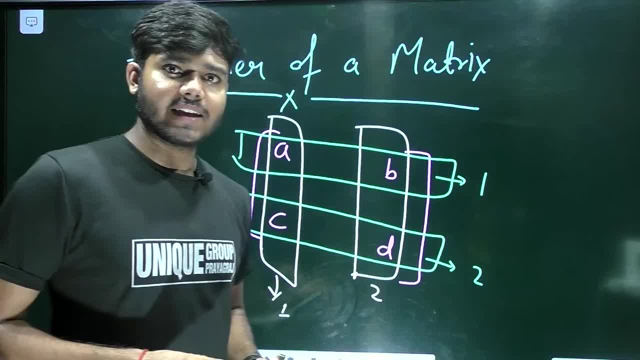 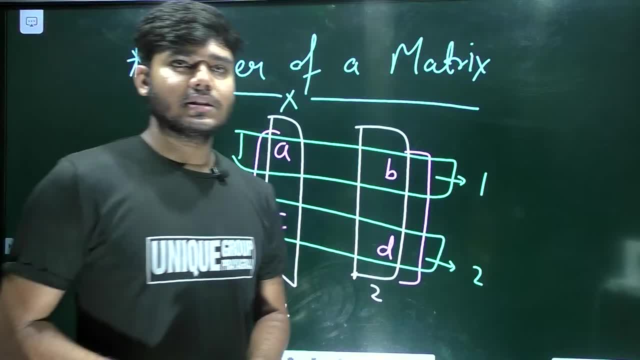 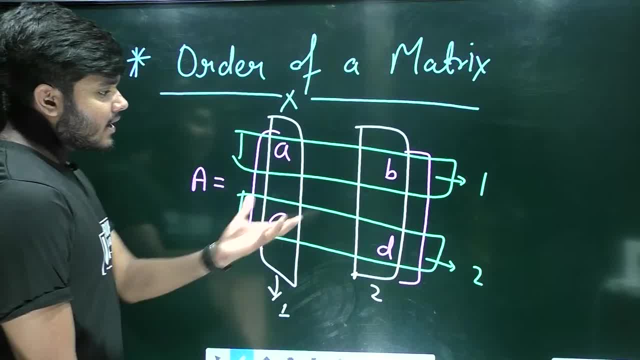 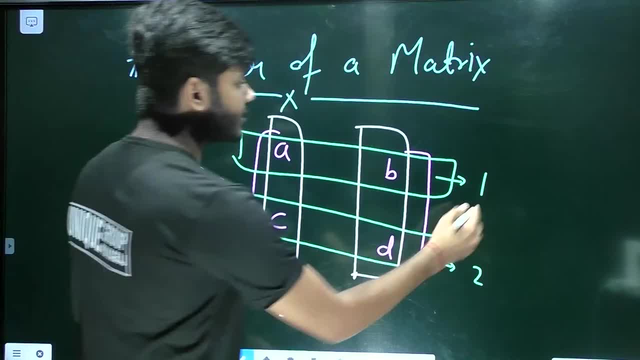 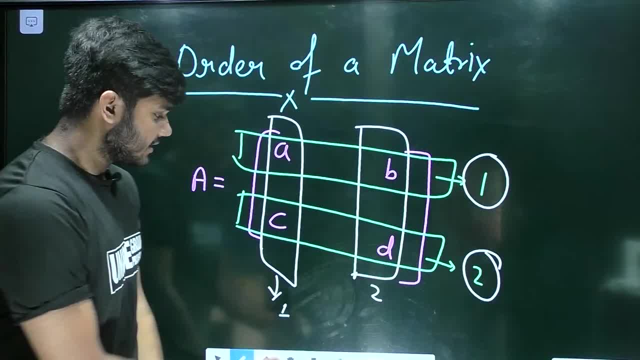 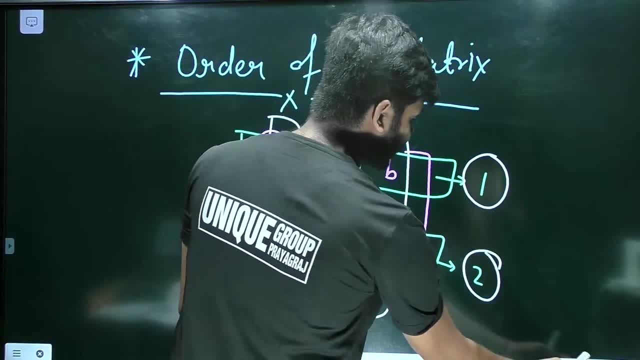 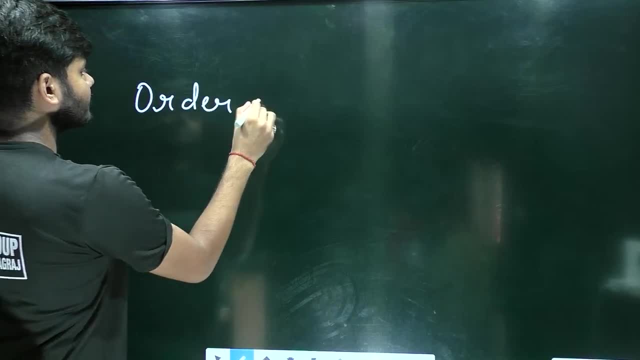 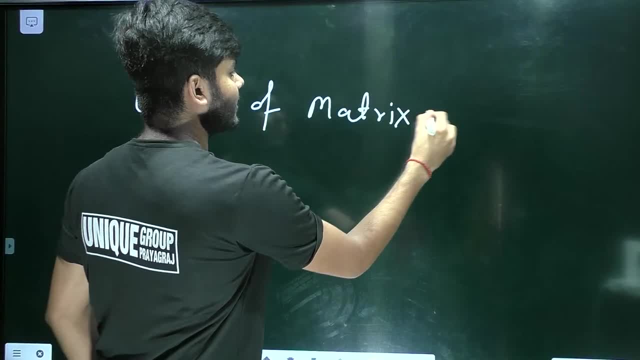 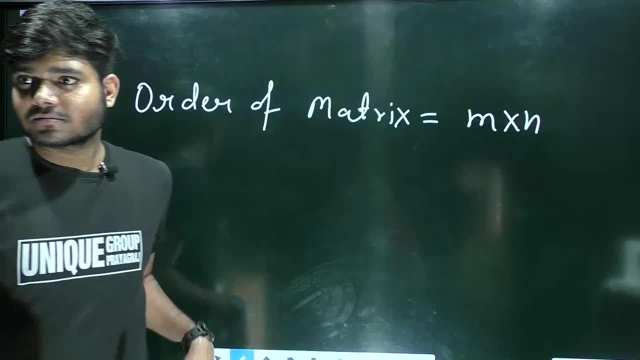 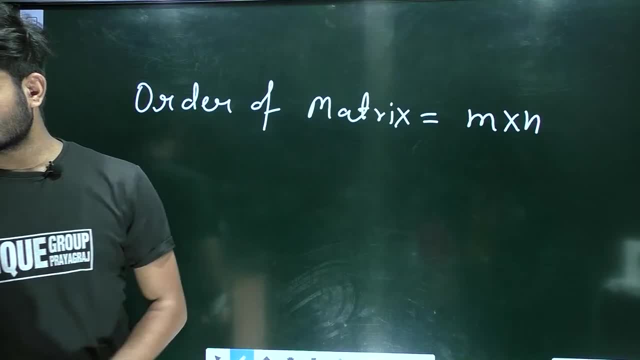 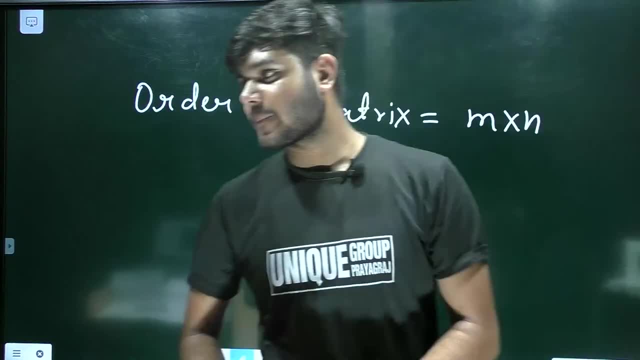 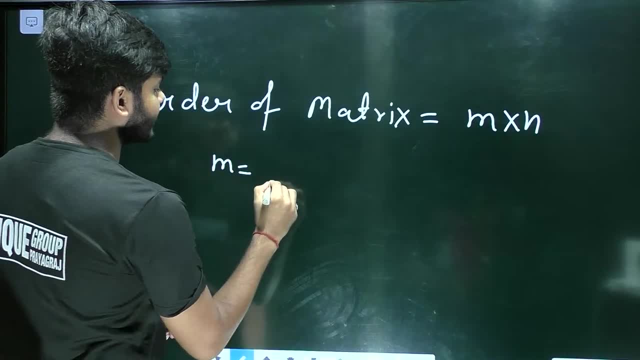 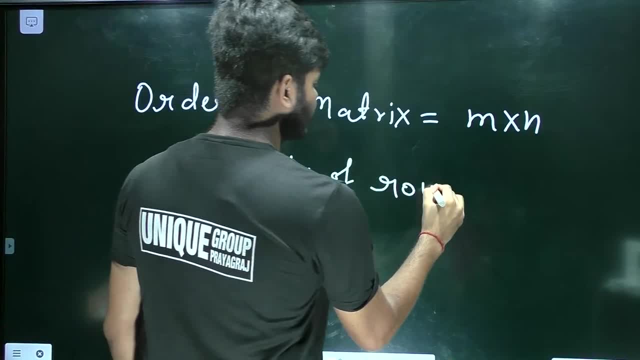 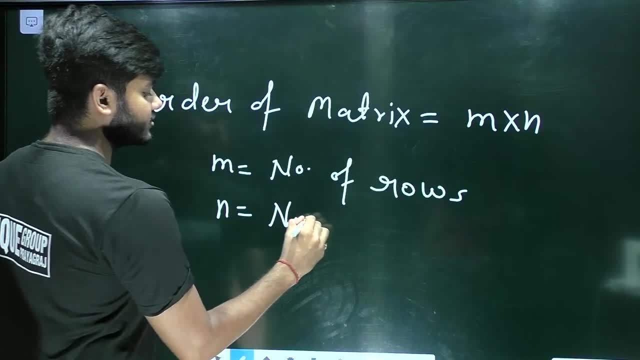 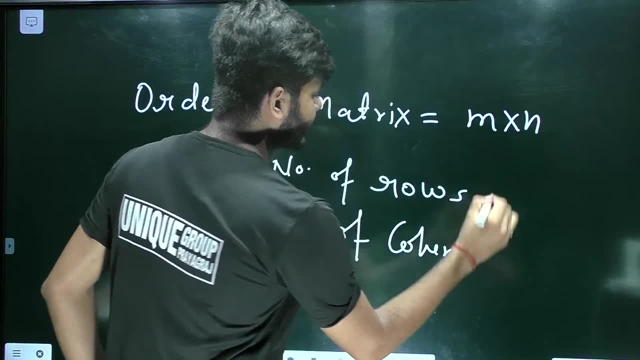 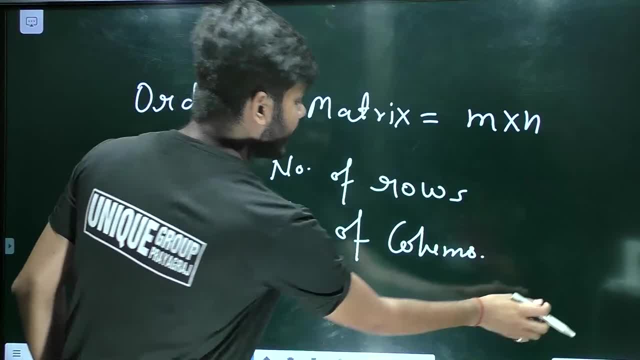 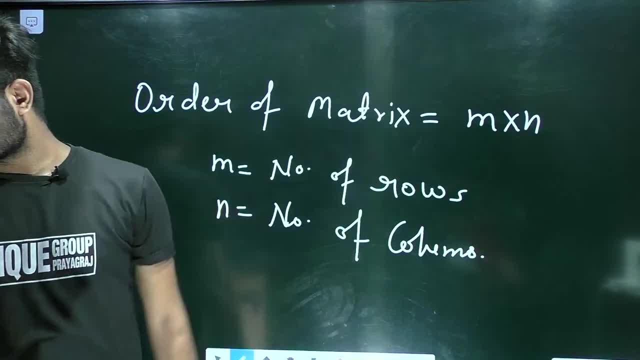 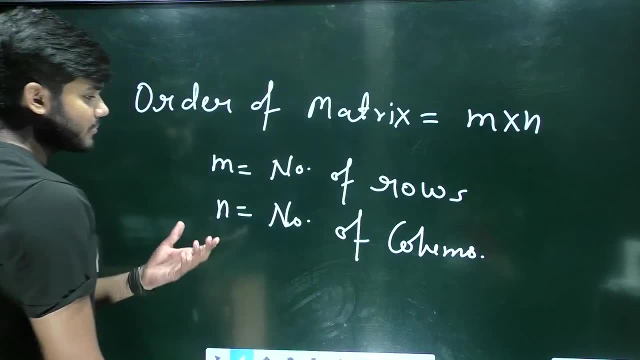 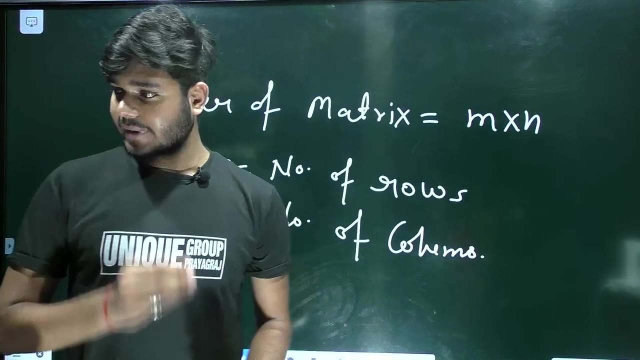 Okay, Remember it is m and n. Okay, Okay, Bro, there may be no matrix in BTech. There is in BC. Right, Let's see, Bro, there is matrix in BTech too. If it is not in your particular university, then, bro, you can study. 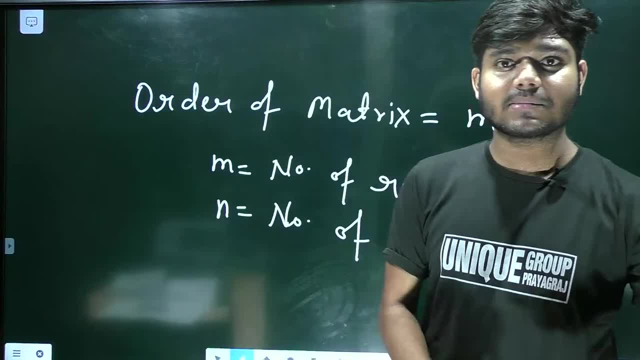 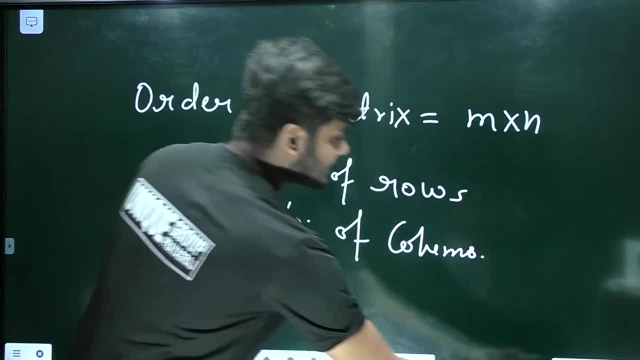 If it is not in your first semester, then it may be in your second semester, But it is there, Okay? So see here What is m? It is the number of rows and n is the number of columns. So now tell us that the particular we have taken, A, B, C, D.